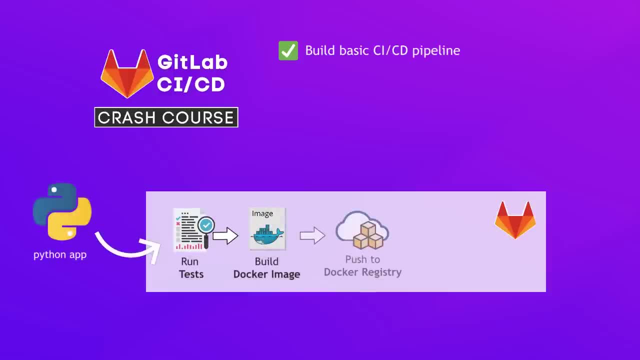 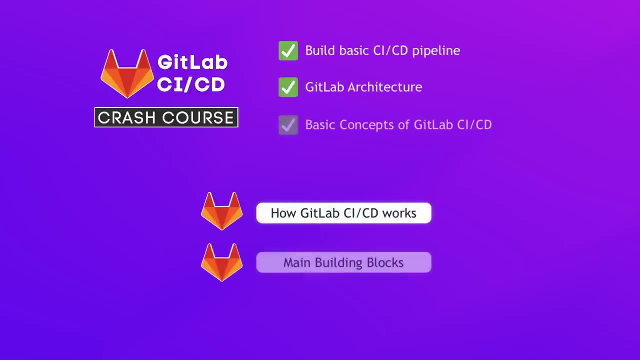 run tests, build a docker image and push to dockerhub's private repository, and then finally deploy the newly built image to a remote Ubuntu server. And while building the pipeline, you will learn the core concepts of how GitLab, CICD works and the main building blocks, such as jobs stages. 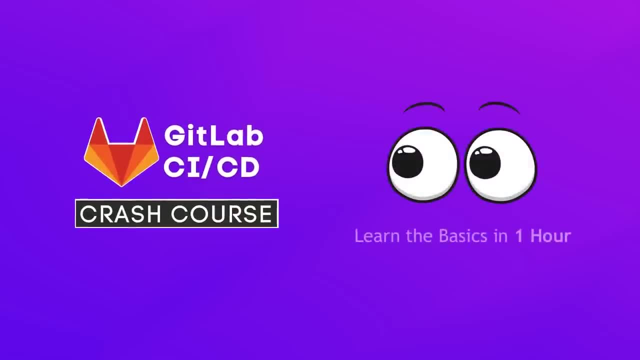 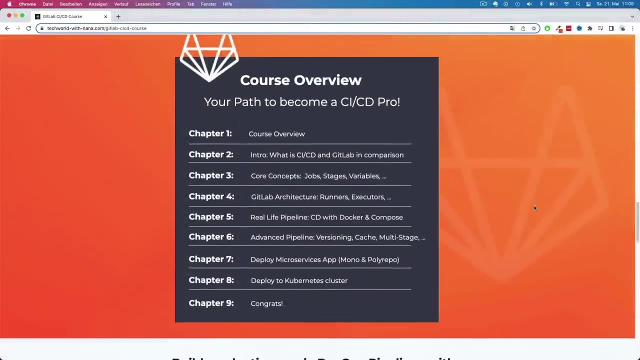 runners, variables, etc. Now, of course, you can learn only so much in one hour, right, And this will help you build foundational knowledge and get started with the GitLab CICD platform. But if you want to dive deeper and start building real-life DevOps pipelines for releasing your applications, 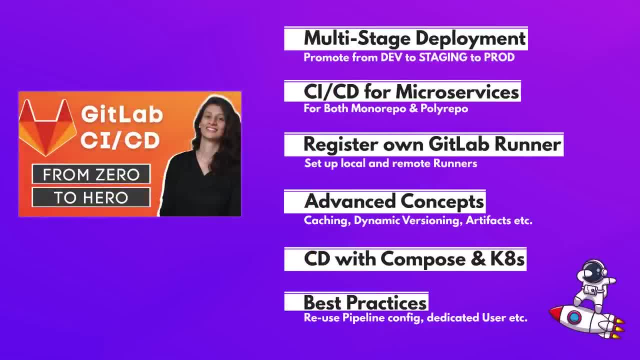 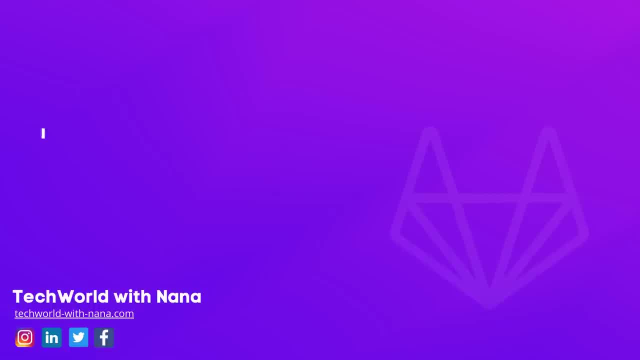 I actually have a complete GitLab CICD course on it, which I have linked in the video description. so if you're interested, you can check it out there. So with that let's get started. First of all, what is GitLab CICD? 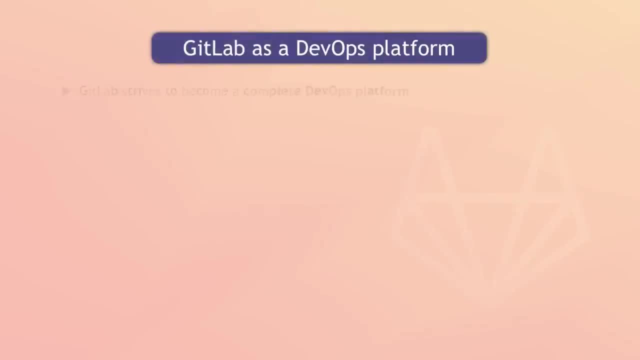 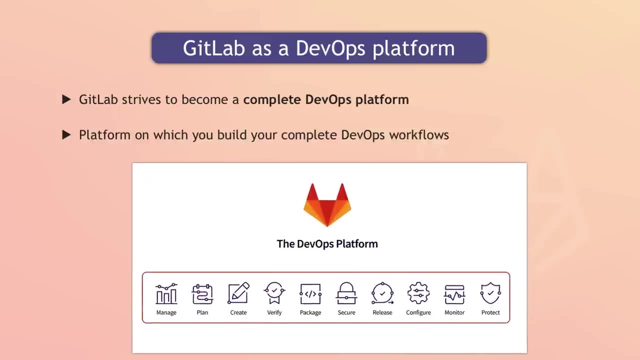 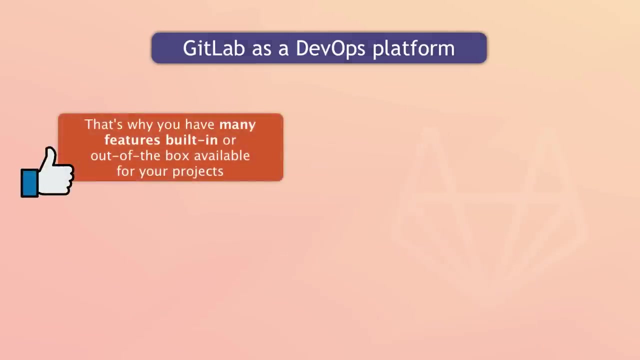 And why should you even care? Now, GitLab platform generally is striving to become the DevOps platform or a one-stop shop for building DevOps processes for your applications. So they have exactly this roadmap and they're working towards that, which means they are actually integrating and creating new features to basically give you everything in one platform. 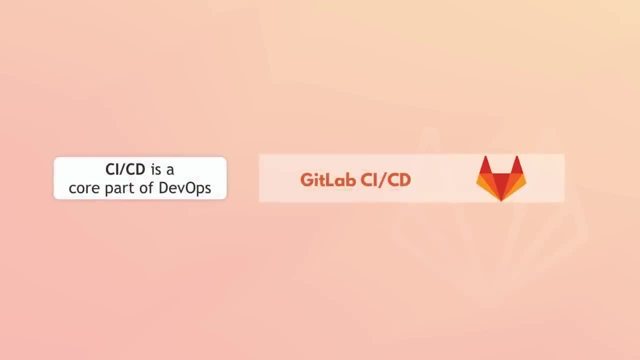 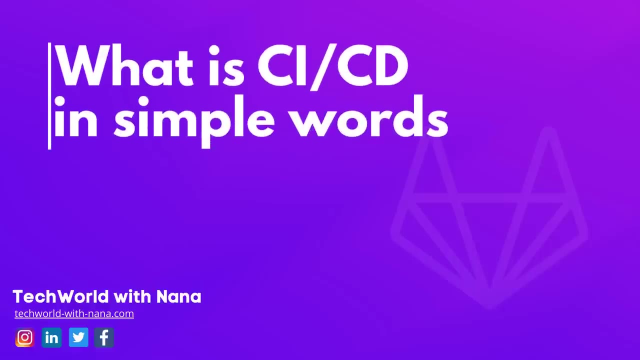 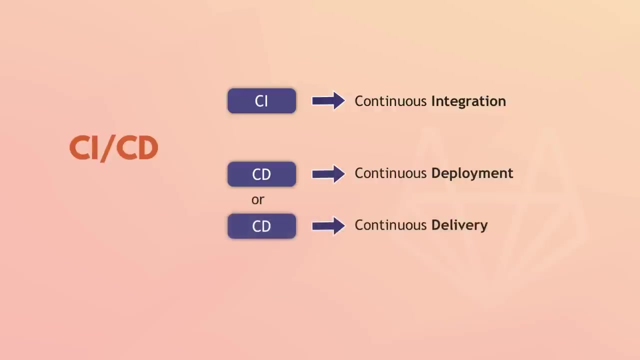 to build complete DevOps processes, And big part of those processes is a CICD pipeline. So, first of all, what is CICD? in simple words, CICD stands for continuous integration and continuous deployment, or continuous delivery, And what it basically means is automatically. 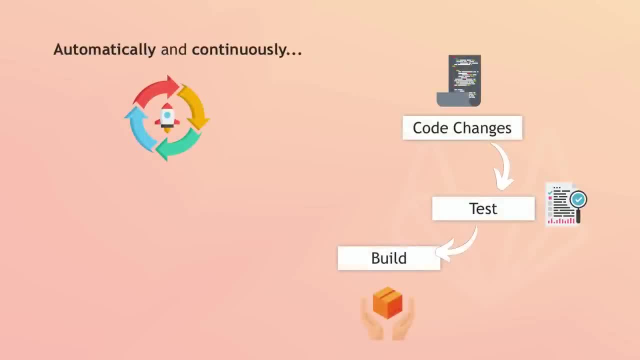 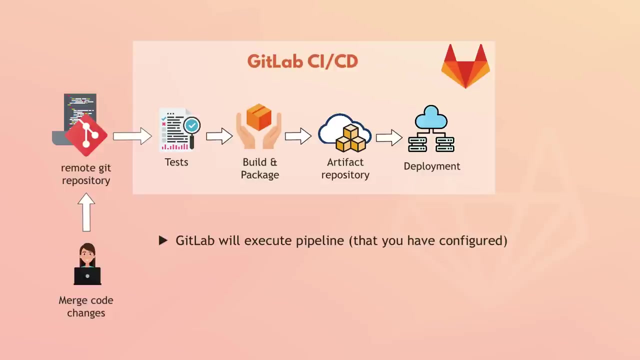 and continuously testing, building and releasing code changes to the deployment environment. So that means when a developer commits a new code into the GitLab repository, GitLab will automatically execute a CICD pipeline that you have configured for your project to release those code changes to the end environment where the end users can access them. But the CICD concept 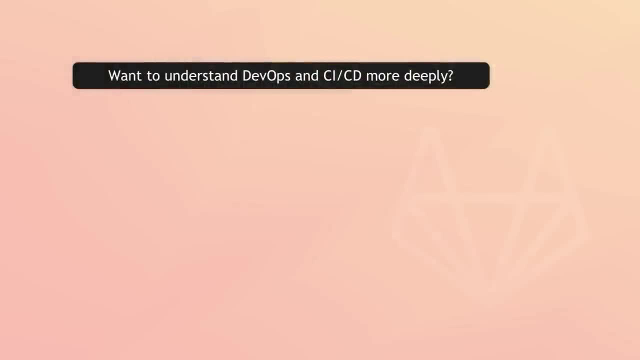 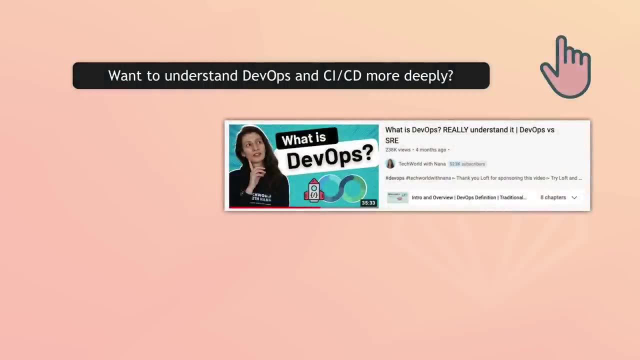 is a topic of its own, so if you want to understand it on a deeper level, then you can check out my other video about DevOps and CICD pipeline, where I explain this in more detail. But, as I said, in simple terms, CICD is to: 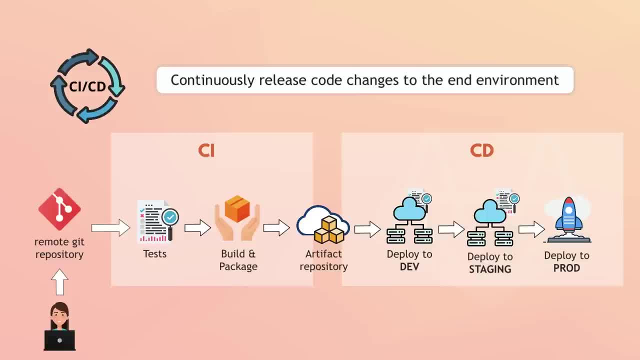 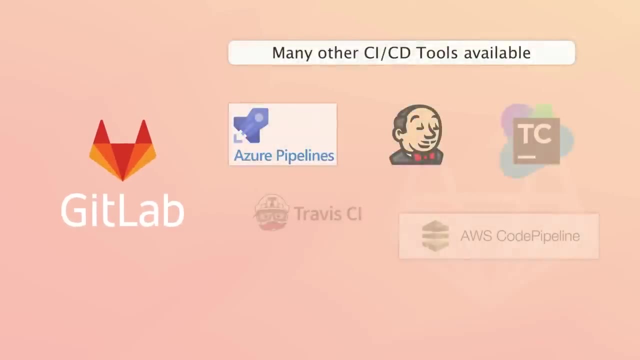 continuously release your code changes to the end environment and in this crash course, We will be building a simplified version of a CICD pipeline using GitLab CICD. And, of course, there are many CICD tools, one of the most used ones in the industry still being Jenkins and 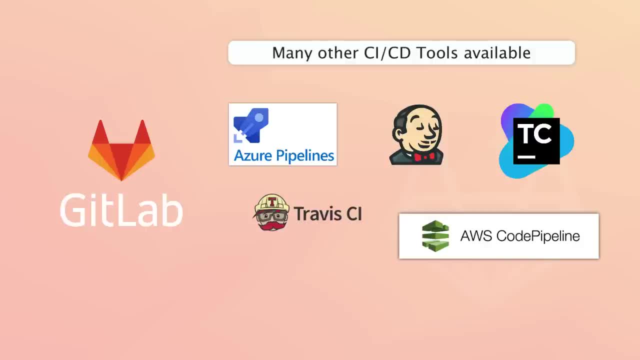 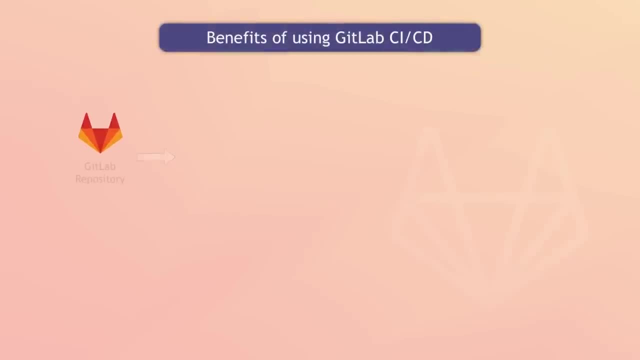 GitLab CICD is just one of those other CICD tools and all of them have their Advantages and disadvantages, But a big advantage of using GitLab to build CICD pipelines for your applications Is that you already have your code on GitLab. 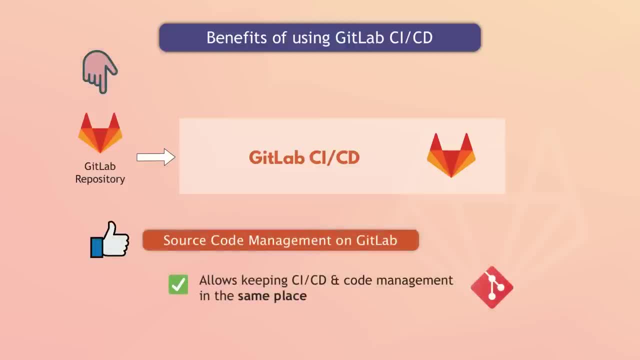 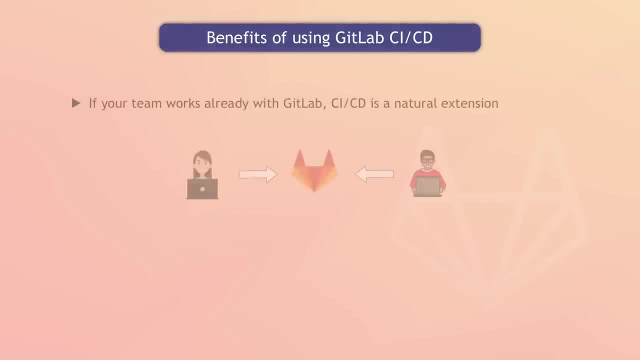 So this is an extension of your software development Processes in your team, where you can also build CICD pipelines on the same platform. So your team already works with GitLab. you have your code there. So this is basically additional feature that you can extend your workflows. 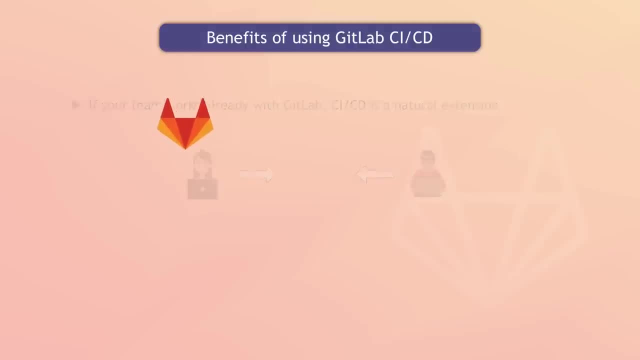 on GitLab with, and you don't need a separate tool for that. apart from that, GitLab makes that extension very seamless by allowing you to get started without any Setup effort and also having your pipeline as part of your application code, Compared to Jenkins, for example, where you have to set up and configure the Jenkins server. 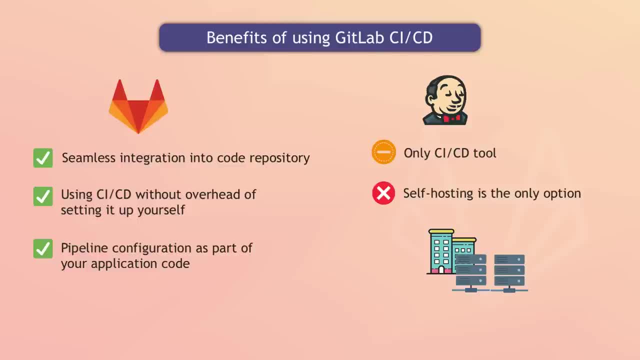 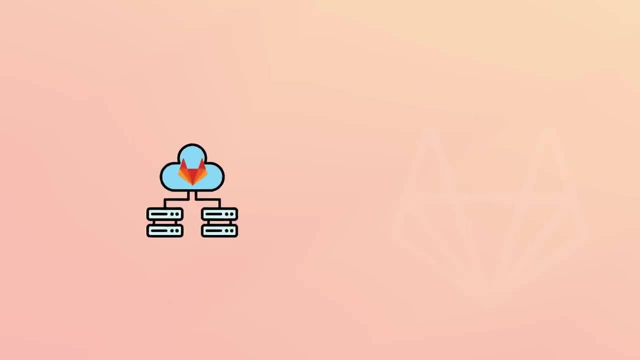 Create a pipeline and then connect it to the Git project. with GitLab, you can start without any of this configuration effort, and We will see that in the demo part. Now, if you don't have to set up anything and configure any servers to run the pipelines, How does it actually work? and this leads us to the topic of GitLab architecture and how it works. 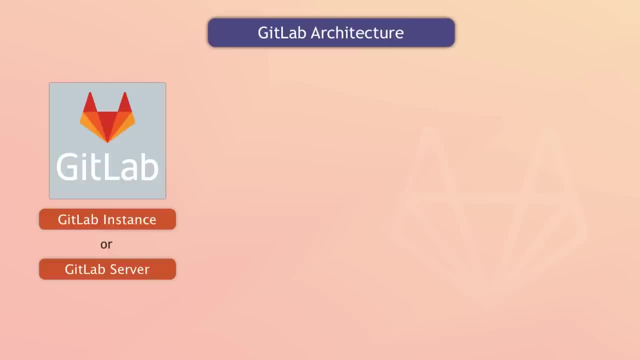 you have a GitLab instance or GitLab server that hosts your application code and your pipelines and basically the whole configuration, so it knows what needs to be done, and Connected to that GitLab instance You have multiple GitLab runners, which are separate machines connected to the GitLab server machine. 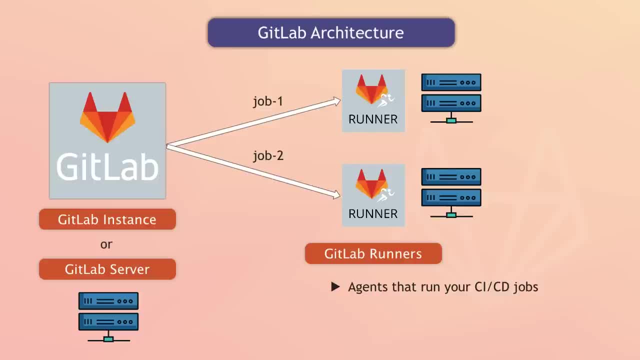 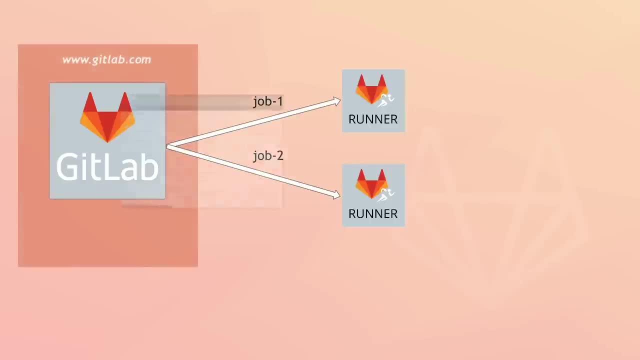 Which are actually the ones executing the pipelines. So GitLab server knows what needs to be done and GitLab runner actually does that, and GitLabcom is actually a managed GitLab instance that offers multiple managed runners already out of the box. So these are all maintained by GitLab and that's why you can start running your pipelines without any. 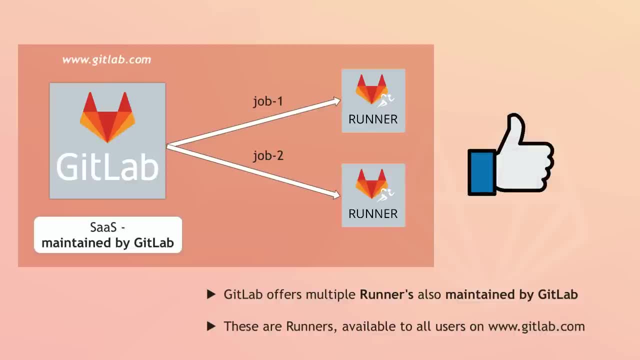 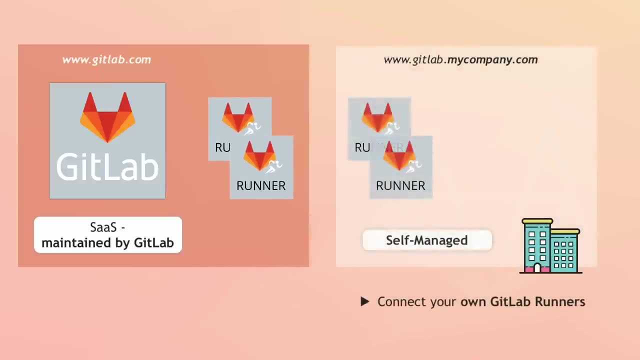 setup and configuration effort Using this managed setup, and this is already enough for starting out, But, of course, for your own organization You may want to manage the runners or the whole setup yourself, So you can create partially or completely self managed GitLab setup as well in this crash course. 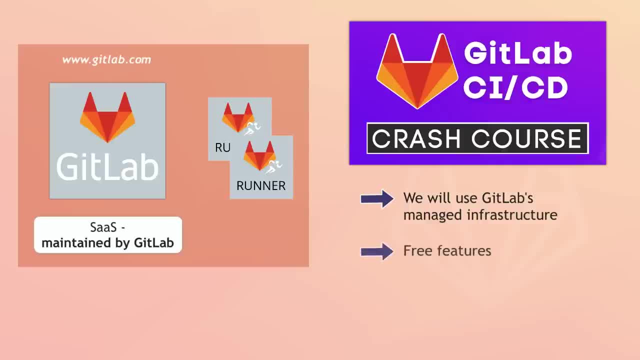 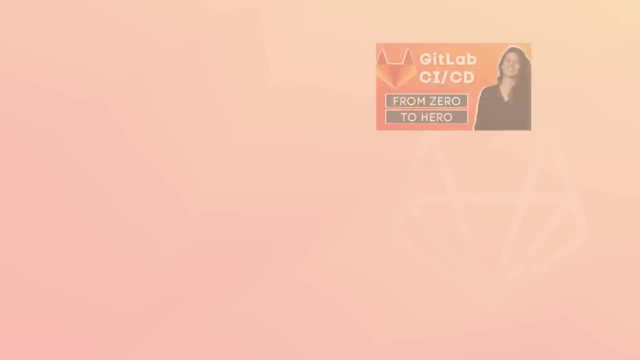 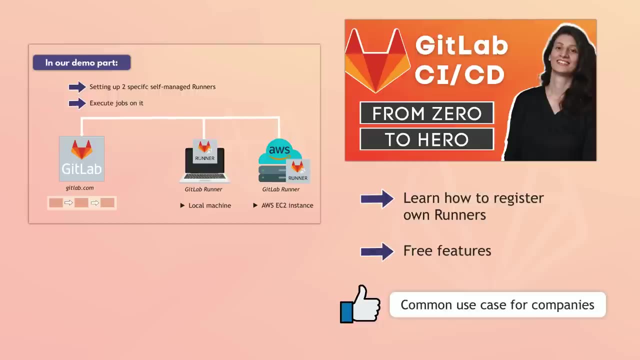 We will use GitLab's managed infrastructure and free features to build our release pipeline, So we will not need to configure anything ourselves. In my GitLab CI-CD complete course, However, you actually learn to create and connect your own runners to the GitLabcom instance. 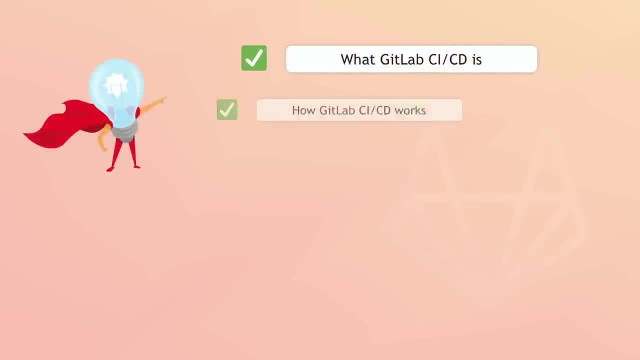 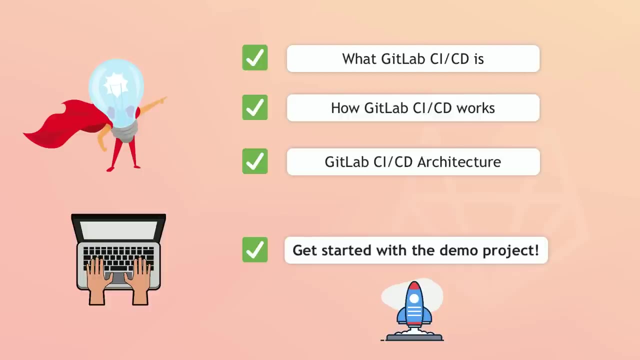 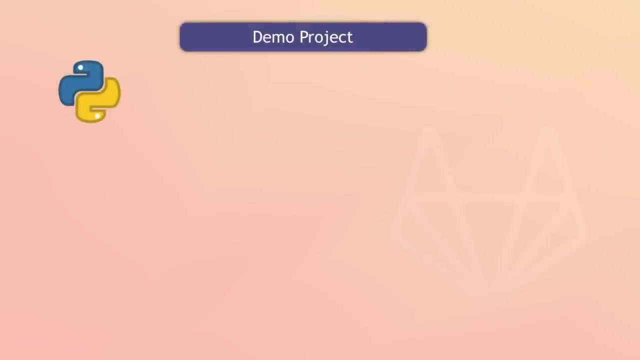 So now we know what GitLab CI-CD is, how it works, how the architecture works. So with that, let's get started with the demo project and learn how to build a CI-CD pipeline. And for the demo project, we're going to use a Python application. 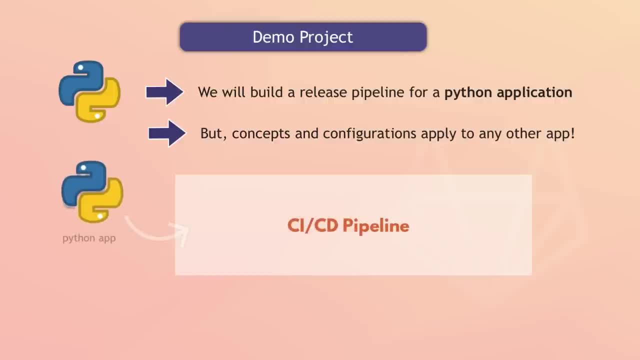 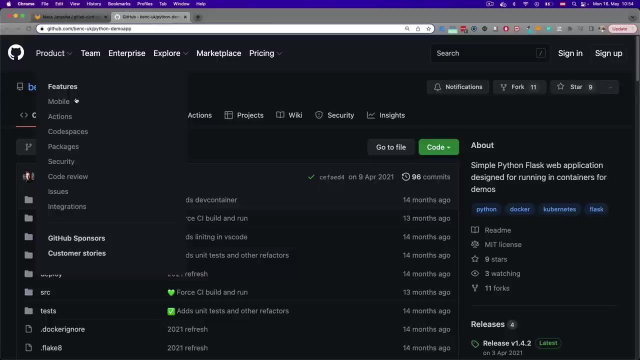 So we're going to be building a simple CI-CD pipeline for a python app where we execute the tests. We built a docker image from the Python application and then we deploy and run it. So it's a web application and the code is from this repository on GitHub. 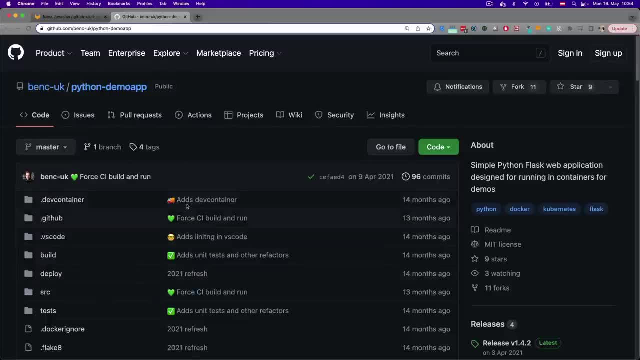 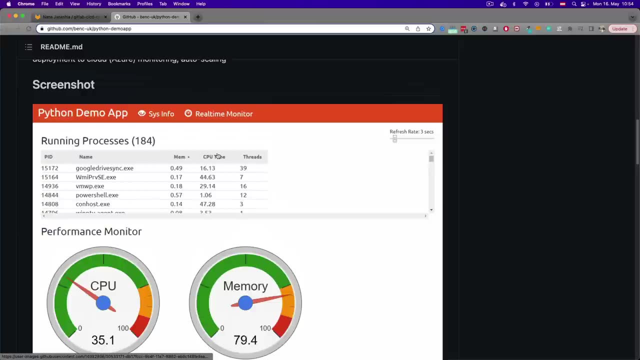 I will link this as well in the video description. So that's basically the original application. It's a demo app that provides some system information, and that's how the UI looks like. You don't have to understand the code behind. We are just gonna concentrate on that at this point. 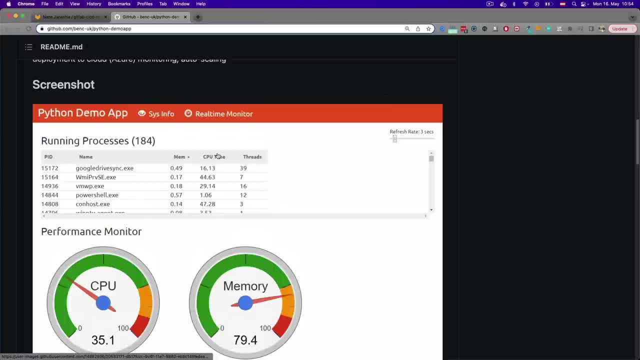 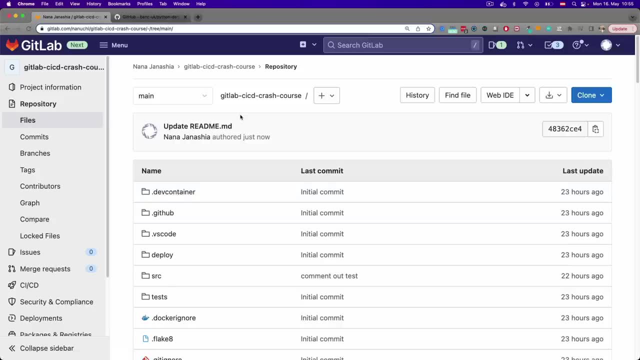 on how to take this application and deploy it using a CI-CD pipeline. I have made just a couple of adjustments here and I have created the repository on GitLab, because that's where we're going to be working with And I'm going to highlight any part of this application code. 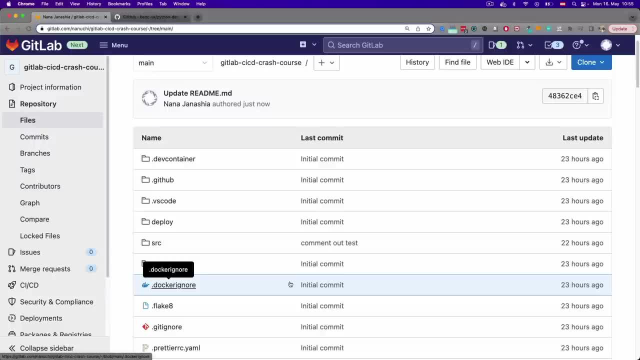 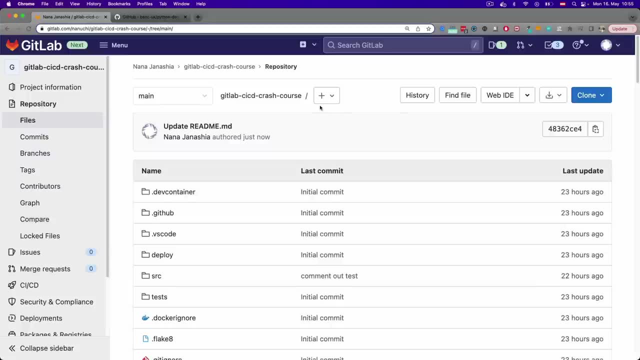 that is relevant for us in order to build the CI-CD pipeline. The rest of them you don't need to worry about. you don't even need to understand how Python applications are written. So what I'm going to do first is I'm going to clone this repository locally so that I can show you how. 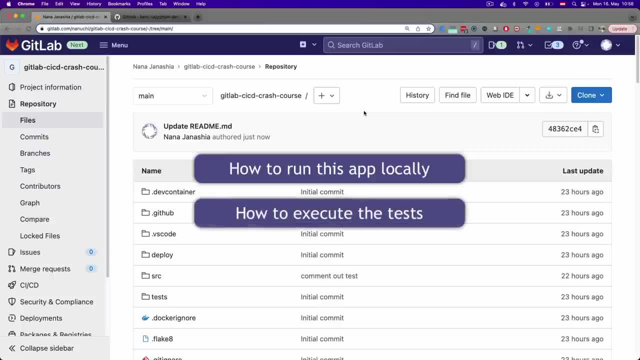 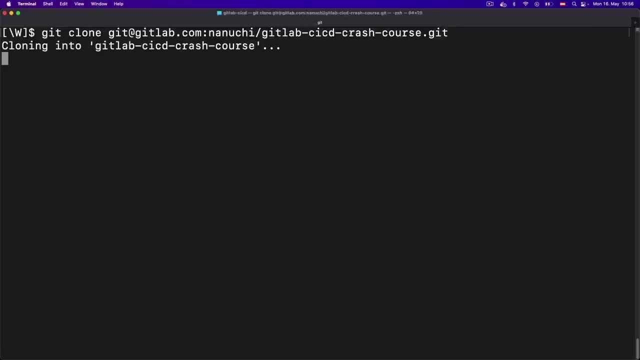 to run this application locally and how to execute the tests, Because we're going to be running tests on the pipeline, so we need to know how that's done. So I'm going to grab the clone URL. So, switching back to the terminal, I'm going to do git clone and the project URL and we called it. 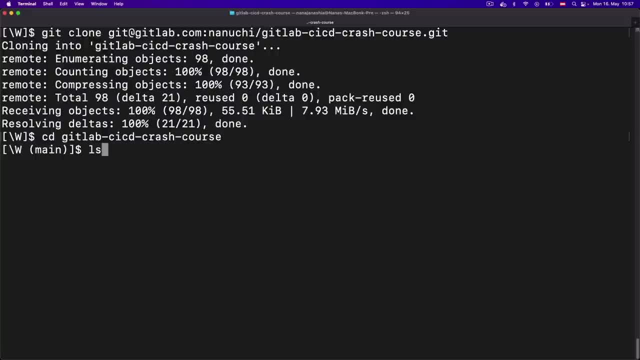 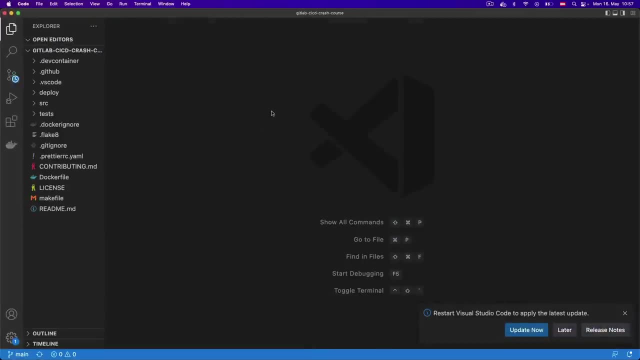 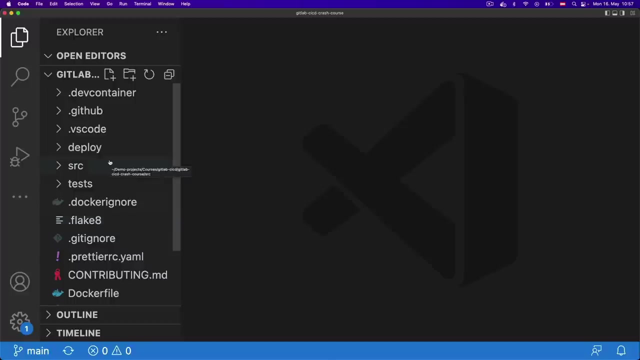 GitLab CI-CD crash course, And that's basically our application. Now I'm going to open this in a Visual Studio code so that we have a better visualization, Make it bigger and let's see exactly what parts of this application code is relevant for us. 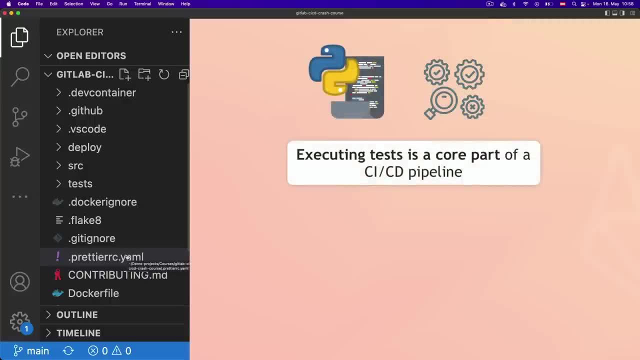 So first, as I said, we're going to be running tests. So in this application we have a couple of tests which we will look at. We'll run during the pipeline which is there to make sure that application code is correct. 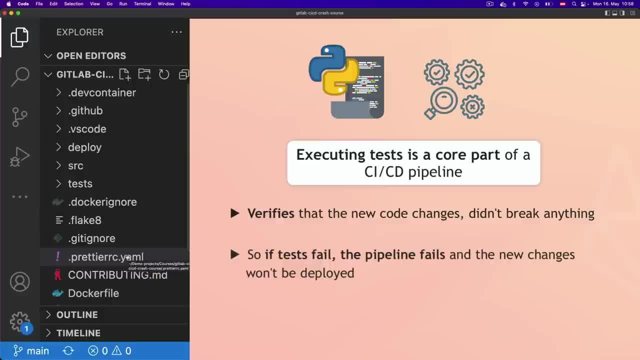 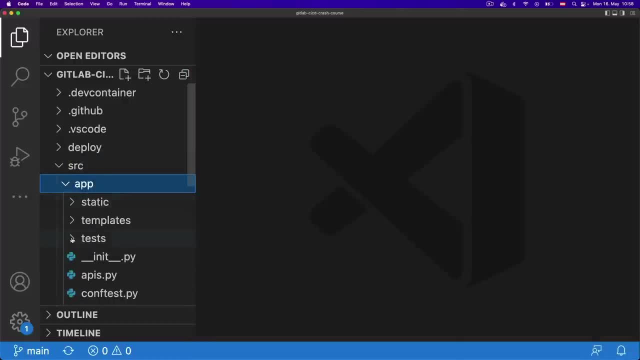 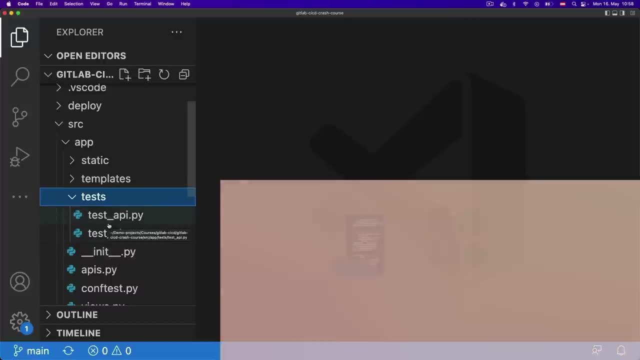 So any changes that we make didn't break the application and the tests can validate that. And in the source folder right here in app we have a folder called tests And inside there we have these two test files that include the test. Again, you don't need to understand how these tests are written, what they actually do. 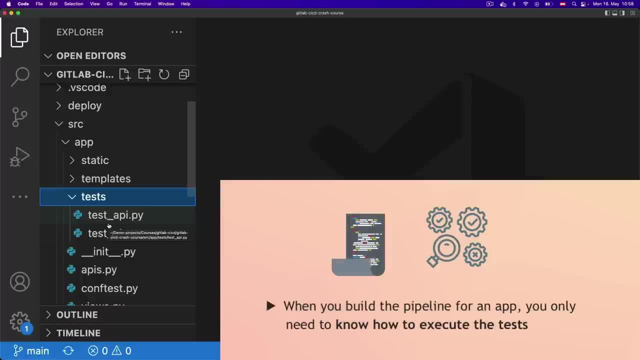 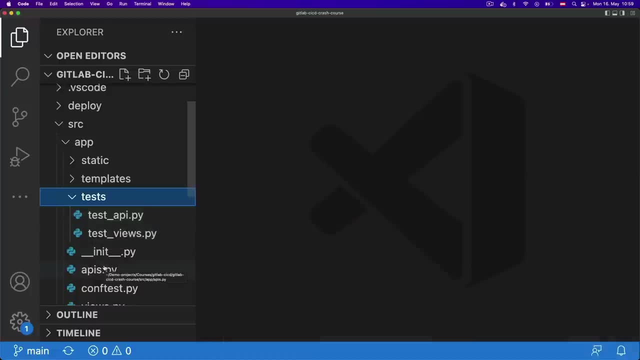 We're using it as an example to Demonstrate how to run tests for any technology, any application inside the pipeline, So you can apply this knowledge for any other application written in any other language. So we have these tests- I think there are four of them- and they're using this configuration file in the test folder to execute those tests. 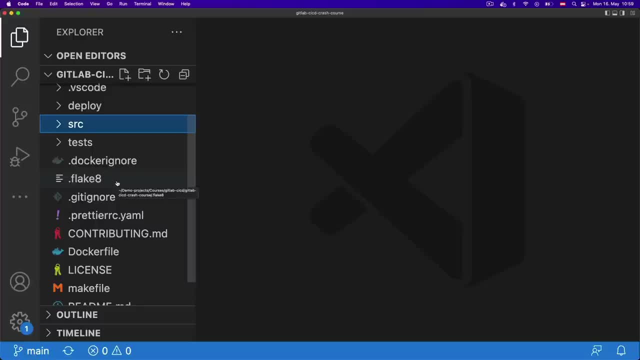 So, as a first step, let's actually see how the tests of this specific project can be executed- And I'm going to open a terminal for that. And again in this specific project to execute the tests, we have this make file that includes a couple of commands, and one of them is test. 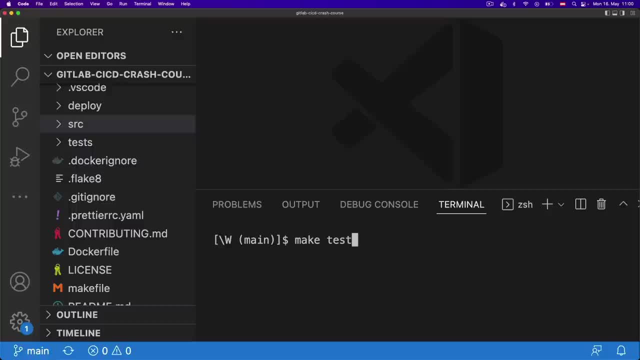 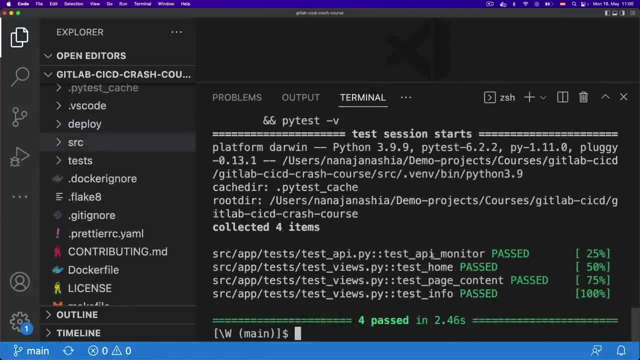 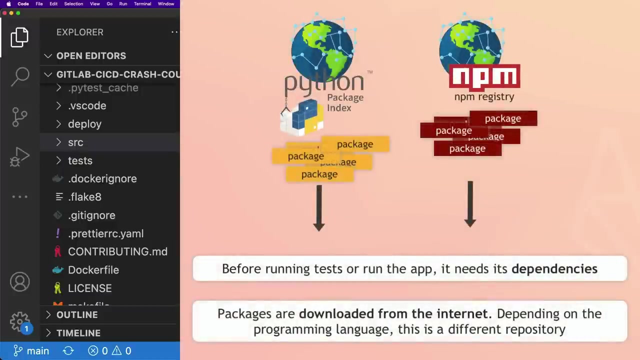 So, using make test, we can execute the tests, basically. So let's run it And there you go. So first of all, it's a general concept in any application with any programming language. applications have dependencies, So these are third party libraries that we include in our application. 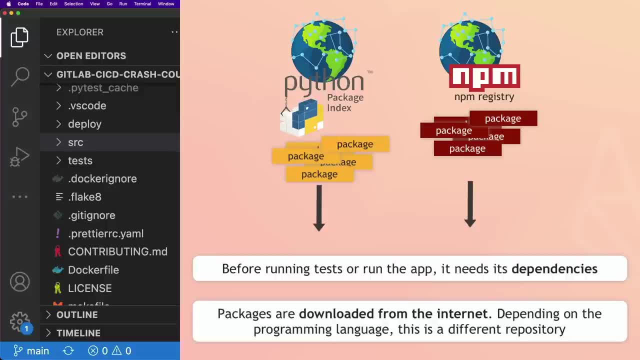 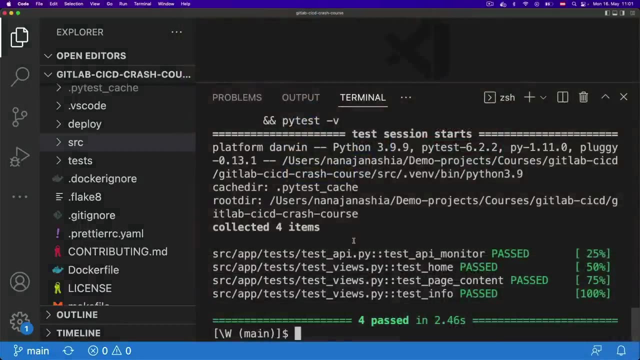 So we don't have to code them from scratch. So we include code that other people wrote that we can use in our applications. And these dependencies have to be downloaded from Internet, Right, Because they live in some code repository. So they need to be downloaded and made available locally so that we can actually run our application. 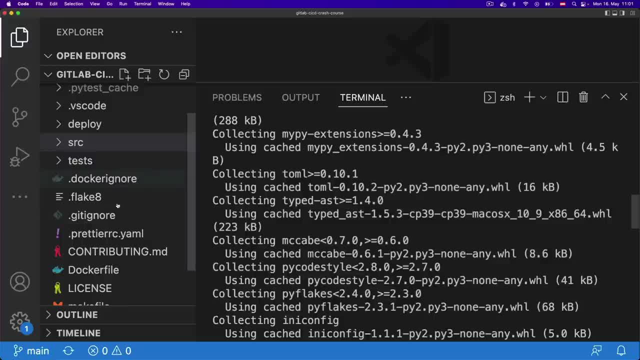 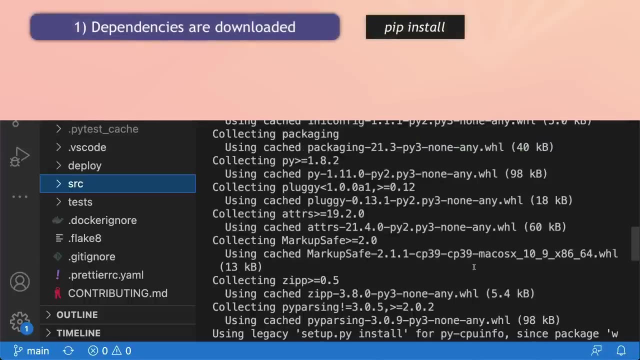 Right, And we have dependencies for tests as well. So in Python specifically, those dependencies are defined in a file called requirements dot txt- Again, different languages, They have different files for that, And at the beginning all the dependencies are downloaded that are needed for the test, and then tests are executed. 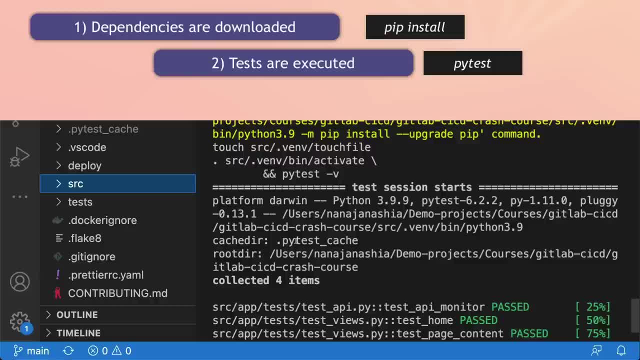 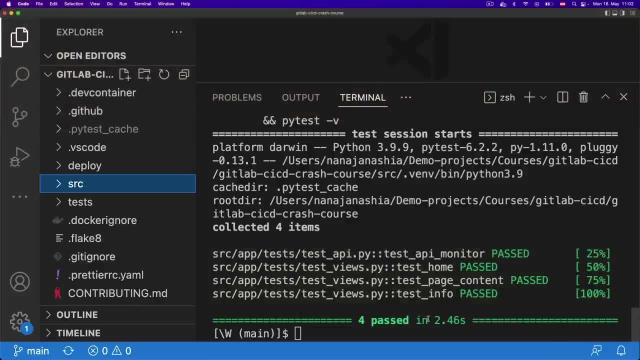 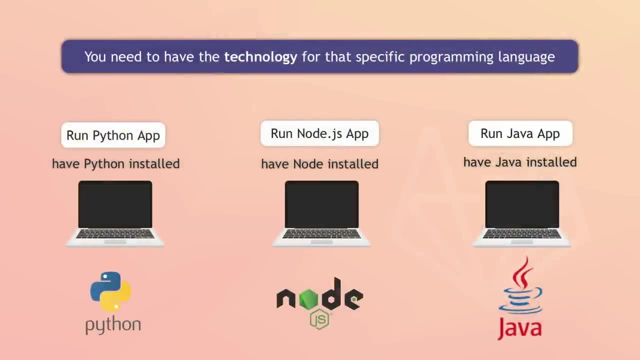 You see here, internally a pi test command gets executed and then we have result of text execution. We have four tests and all of them passed. So that's how it looks like And this is also a general principle. When you run an application, whether it's Java or Nodejs or Python application, you always need that technology. 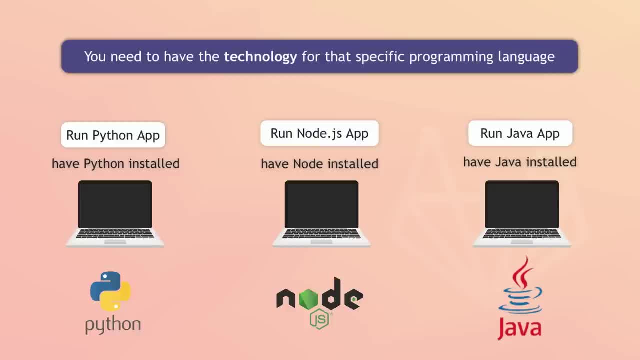 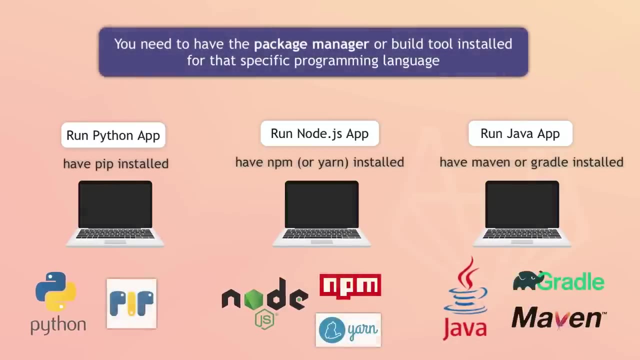 The tool. It Is installed locally, Right? So if I run Python application, I need obviously Python to be available on my machine. If I run Java application, I need Java to be installed and available locally, So I have Python. I also need to have peep installed, which is a package manager for Python, which is the tool that actually downloads and fetches those dependencies from the Internet. 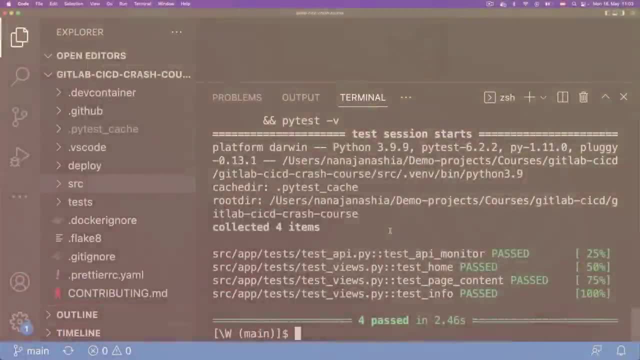 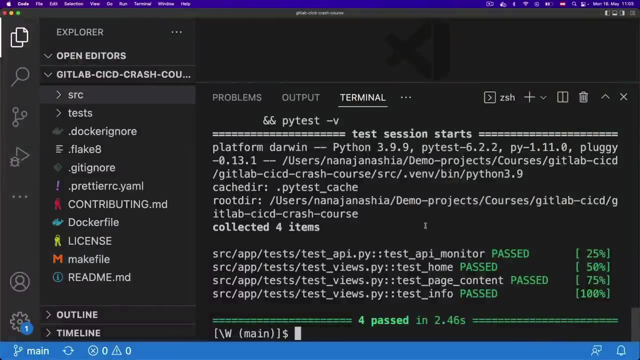 Again, other languages have their own tools for that. And finally, because we have the make file here To execute those commands, we need make command as well to be available on the machine, And this means that we need these three tools to also be available inside our pipeline when the tests are executed. 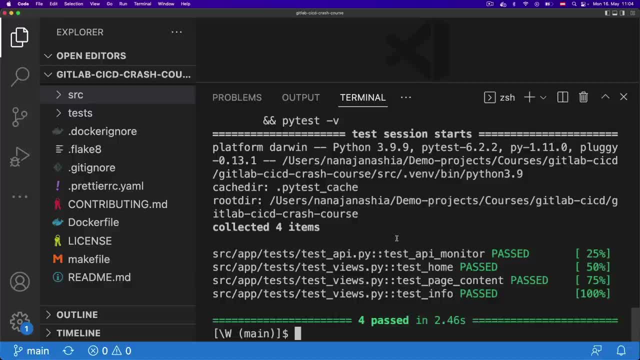 And we're going to see that a bit later. Now I'm going to do one more thing, which is actually start the application locally and see how it looks in the browser, And for that we have another command called make run, And this will start the application. 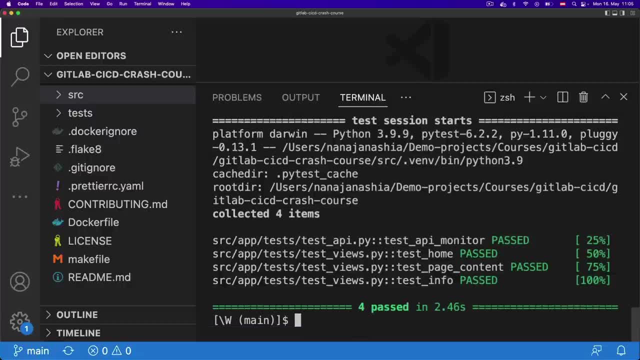 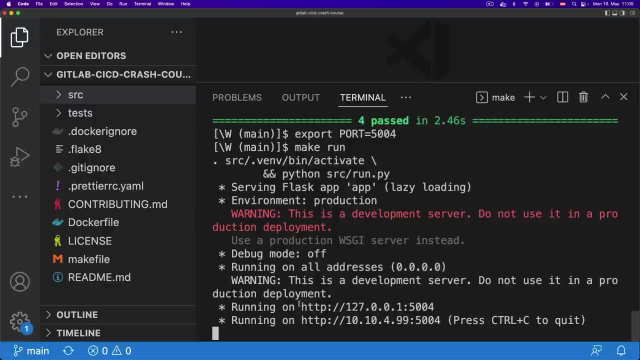 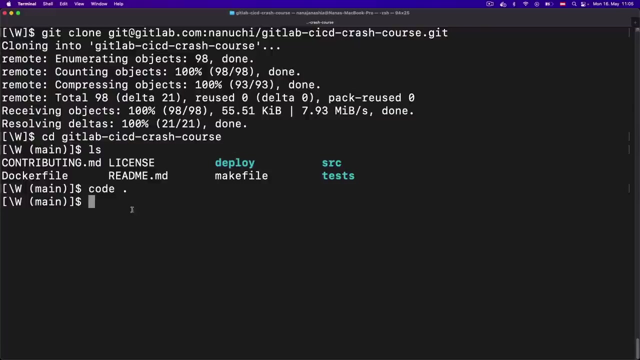 On port 5000, if I want to change the port- and I actually do want to change the port because I have already something running on port 5000. So I'm going to set port to- let's do- 5004 and make run, and this will start the application locally and then I can access that local host, port 5004.. 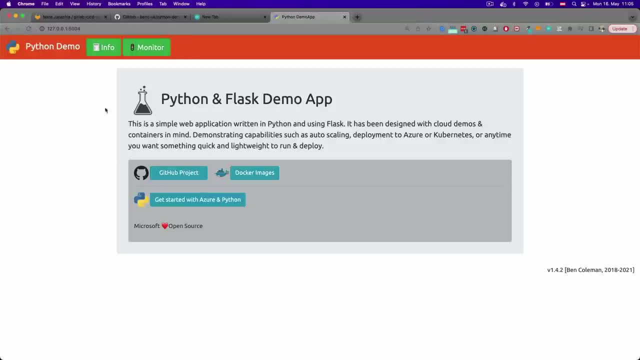 Let's see that. And there you go. That's how the application looks like. We have The monitoring dashboard info and some other stuff. So that's the application that we want to release using a city pipeline on a deployment server. So now we know how the application looks like, how to run the tests. 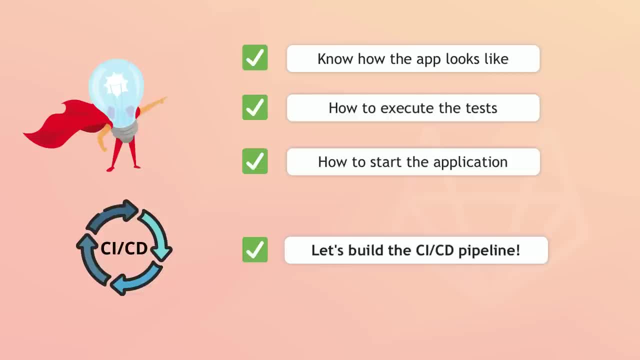 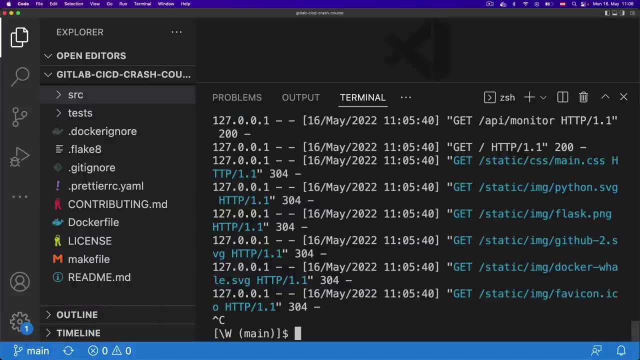 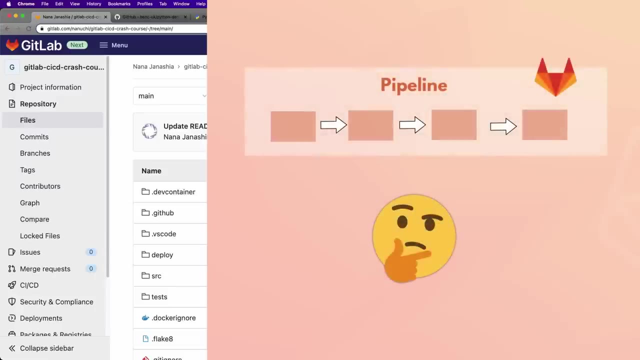 So let's actually go ahead and build a simple city pipeline for this demo application. So I'm going to stop this. Let's actually remove the terminal. And now the question is: how do we create a GitLab CI city pipeline? Well, following the concept of configuration is code. 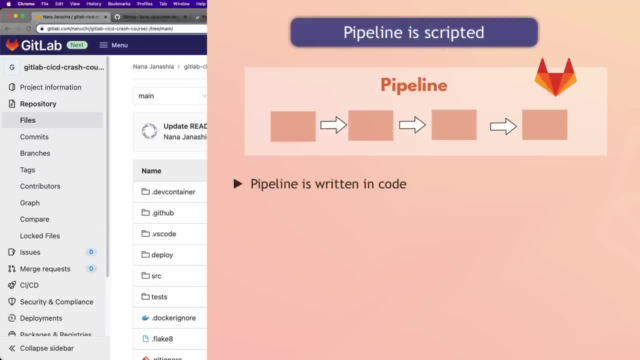 The whole pipeline will be written in code and hosted in the applications Git repository itself in a simple YAML file, And the file has to be called dot GitLab. dash CI, dot YAML. GitLab can automatically detect the pipeline code and execute it without any extra configuration effort from our side. 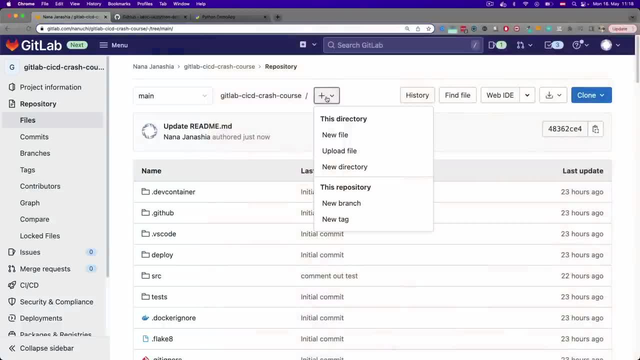 So in the root of the project repository we're going to create this YAML file and we're going to write all the pipeline configuration inside, And we can actually do that directly in the GitLab UI as well, So we don't have to switch back and forth from the editor to GitLab. 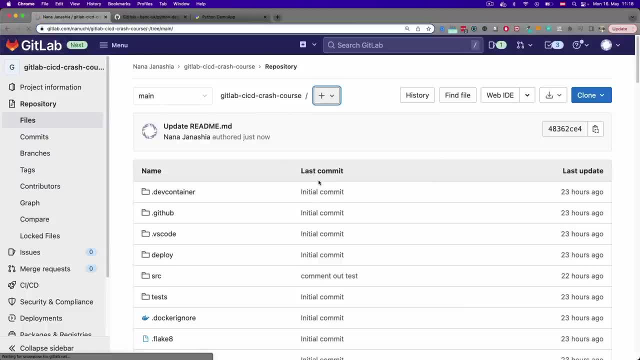 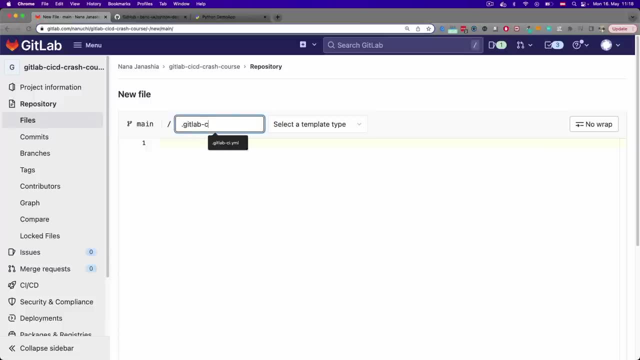 So I'm going to do that directly here: Create new file And, as I said, it has to be called dot GitLab, dash CI, dot YAML. And as soon as I type that in, you see that it automatically fills out the rest, because it detected that we're creating the pipeline code. 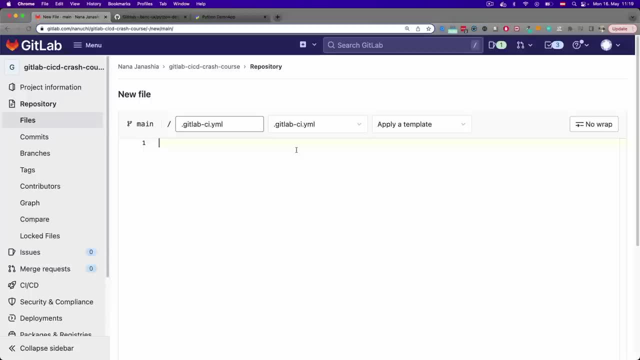 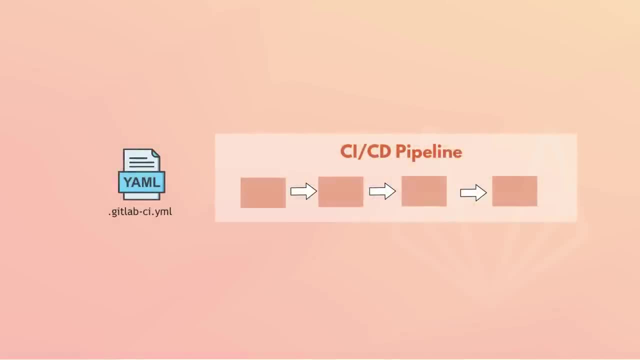 And now let's write our pipeline in a simple YAML format. So the tasks in the CI city pipeline, such as running tests, building an image, deploying to a server, et cetera, are configured as what's called jobs. So let's create jobs for all those tasks. 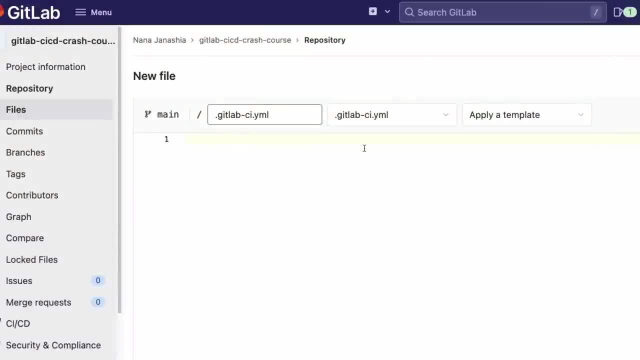 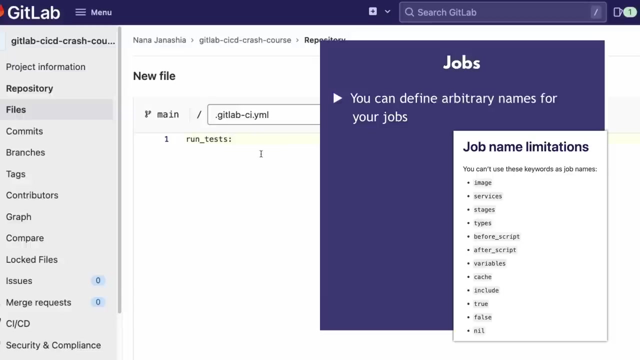 So first let's create a job that will run the tests, And we have a super simple syntax for that: We simply write the name of the job. So let's call it run tests and underscore to separate the words is a standard syntax in the pipeline configuration code on GitLab. 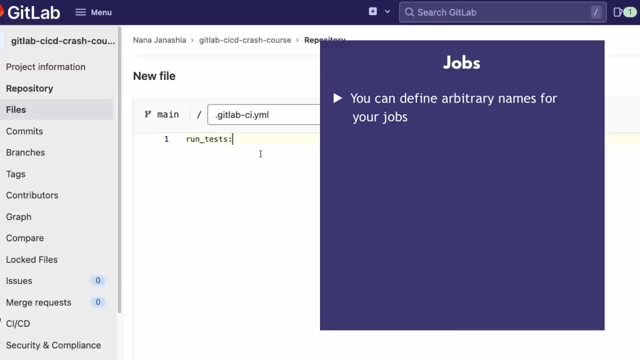 So that's what we're going to do, We're going to use, So that's the job name And inside the job we have a couple of parameters or a couple of attributes or things that we want to configure for the job And, again, know the syntax of YAML. 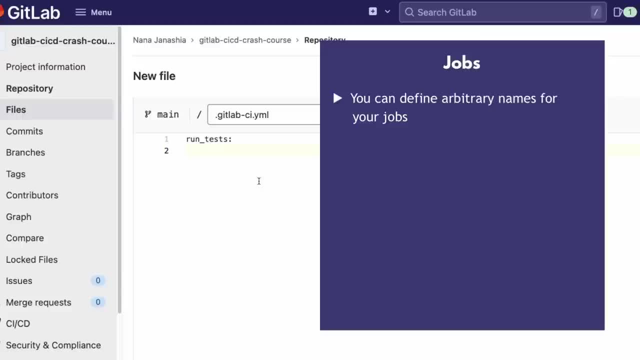 where we have the indentation for each attribute. So the first attribute and the required attribute of a job is what's called a script, And script is basically where we list any commands that should be executed for that job. So, for example, run tests- make tests is a command that needs to be executed in order to run the test. 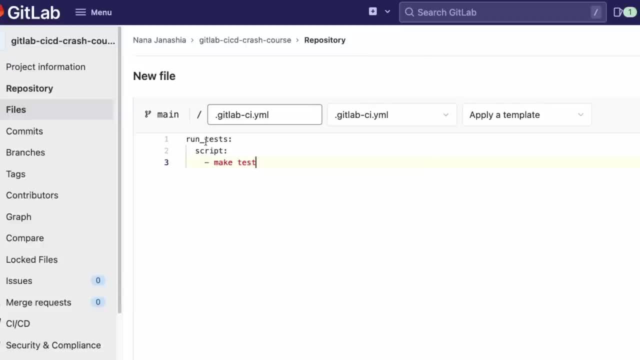 So we're going to write that command right here. So that's actually a job configuration to run the tests. Simple as that. We have the name of the job and inside that we have a script that tells what should this job actually do? and we're saying that it should run command called make test. 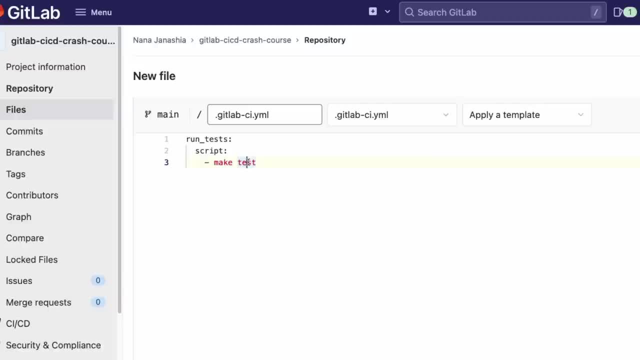 which will execute the tests just like we did locally. But in order for this to run successfully, we need to do a couple of things. Remember I told you that the make test command to be successful, needs first of all make command to be available wherever this job runs. 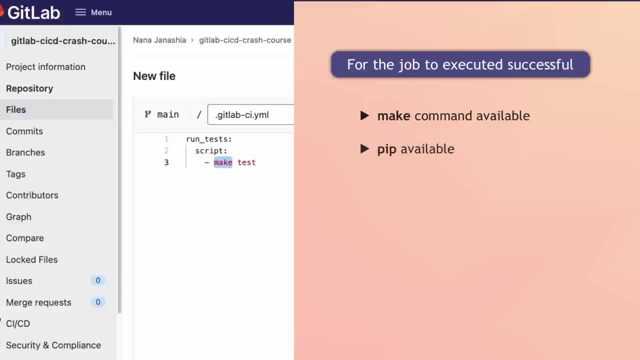 But also in the background. it will execute PEEP to install the dependencies, and it will also execute Python, because tests are written in Python, So we need that to be available as well. So these three things need to be available on the machine where this will run. 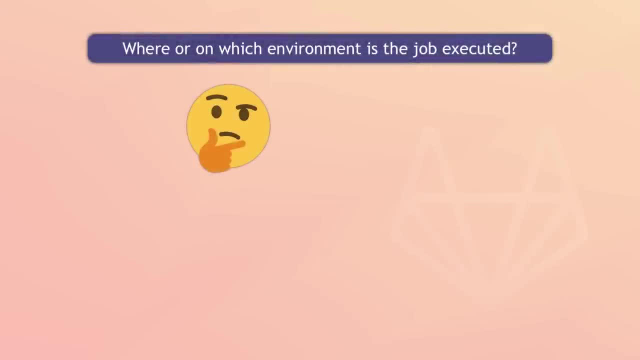 And now we come to the question of where will this job actually be executed? on which machine, on which environment? Is it a Linux machine? Is it Windows? What is it? As I mentioned in the beginning, pipeline jobs are executed on GitLab runners. 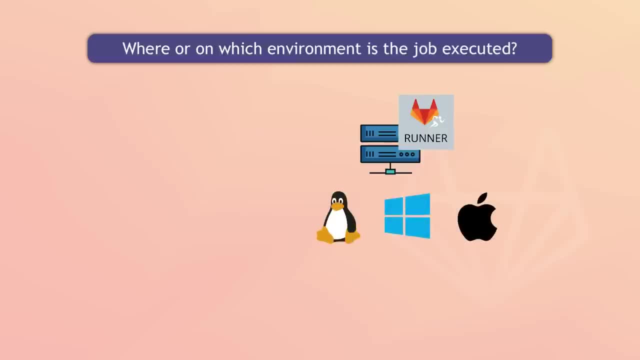 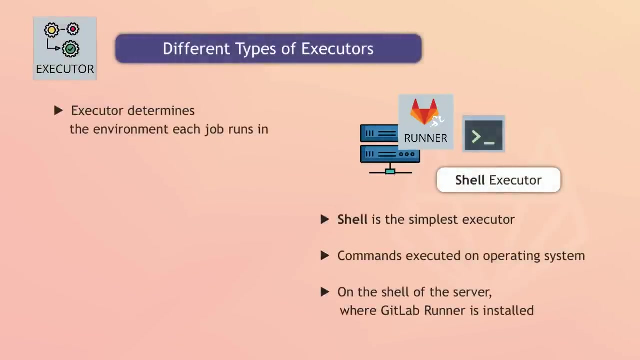 and GitLab runners can be installed on different environments. It could be a different operating system, like Windows, Linux, different distribution of Linux, etc. And that's what's called a shell executor. It's the simplest type of executor, simplest environment, what we know from Jenkins, for example. 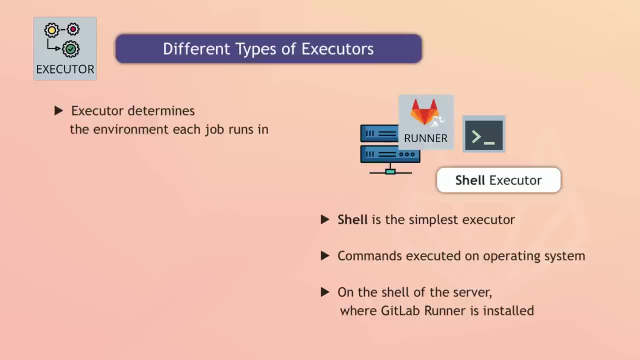 where you have a simple server on Linux machine and you execute shell commands on them as part of your job directly on the operating system. But another common execution environment on GitLab is Docker container. So instead of executing the jobs directly on the operating system, like on a Linux machine, for example, 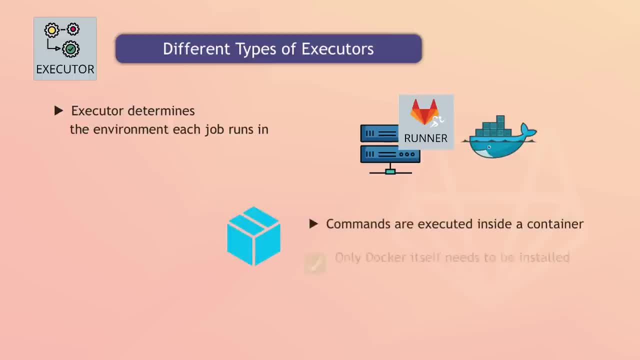 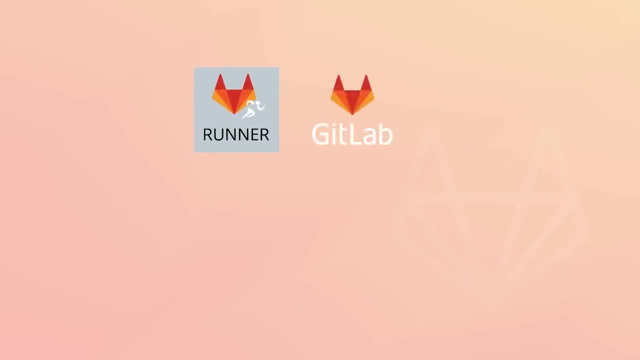 we execute the jobs inside containers. So the GitLab runner is installed on some Linux machine And on that machine GitLab runner creates Docker containers to run the jobs. And the managed runners from GitLab that we get available out of the box actually use Docker container as the execution environment. 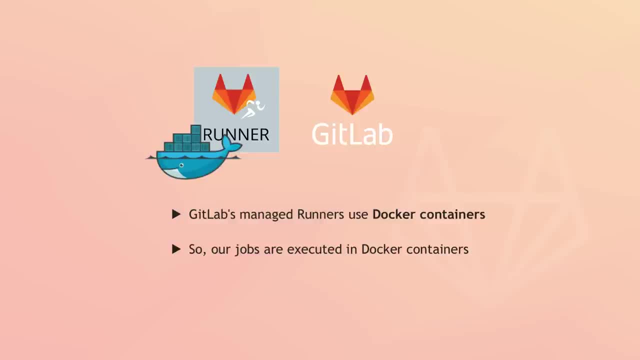 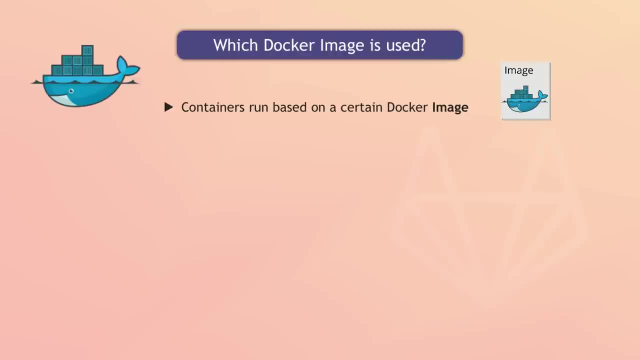 So all our jobs that we write here will be executed inside Docker containers. But, as you know, containers run based on a certain image, right, You can't run a container without an image And depending on which image you use, you're going to have different tools available inside that container. 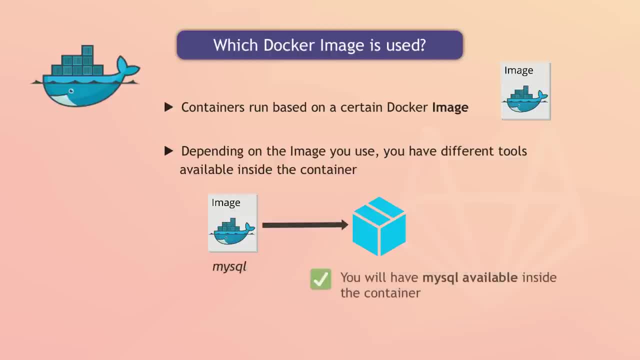 So if I use a MySQL image to start a container, I'm going to have MySQL inside plus some other tools that the image has. If I have Nodejs image, then I'm going to have Nodejs and NPM available inside the container. If I use a basic Alpine image, 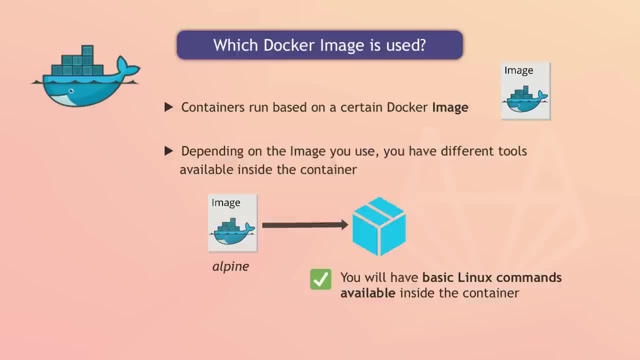 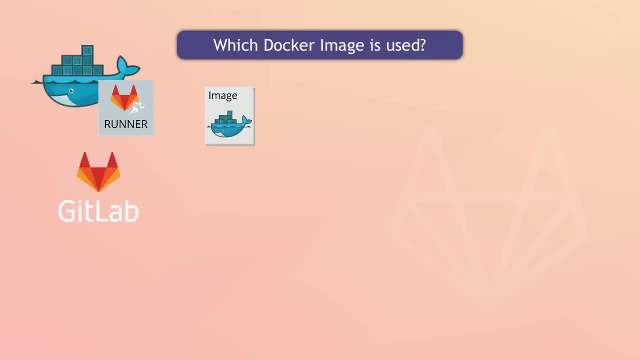 then I'm going to have basic Linux commands and tools available inside. So which image are GitLab's managed runners actually using to start those containers? Well, by default, currently, at this moment, GitLab's managed runners are actually using Ruby image to start the containers. 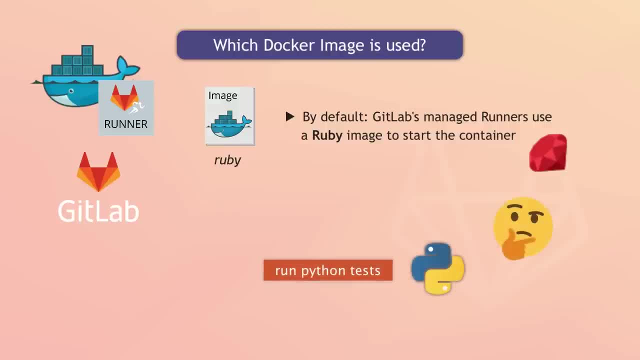 that will run the jobs. Now, in our case, this is not going to work because for our test execution we actually need a container or an image that has Python pip and make available inside them, Right? So instead of Ruby image, we want to use a Python image to execute this job. 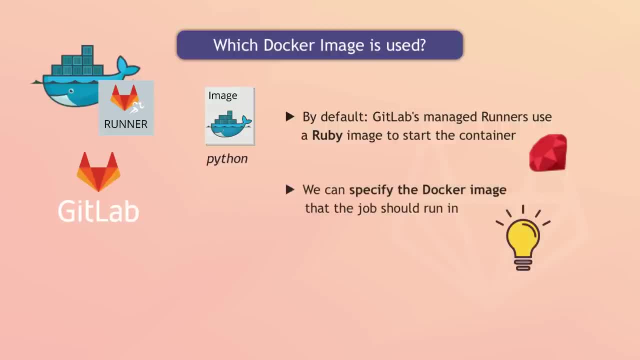 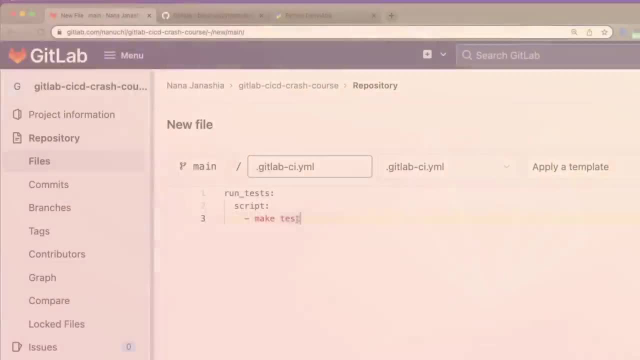 And the good thing is that we can actually overwrite which image is used by the runner for each specific job. So for each job we can say: you know what, forget Ruby, use this image instead. And we can do that using an attribute on the job called image, and then 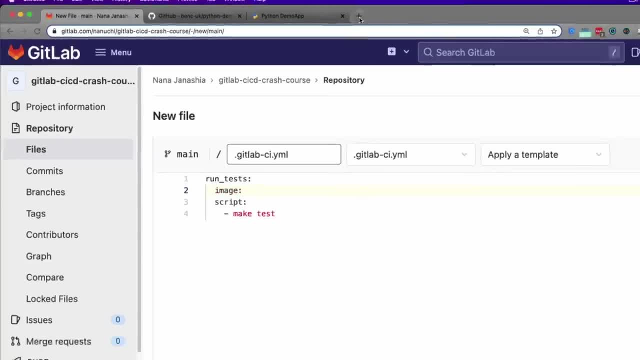 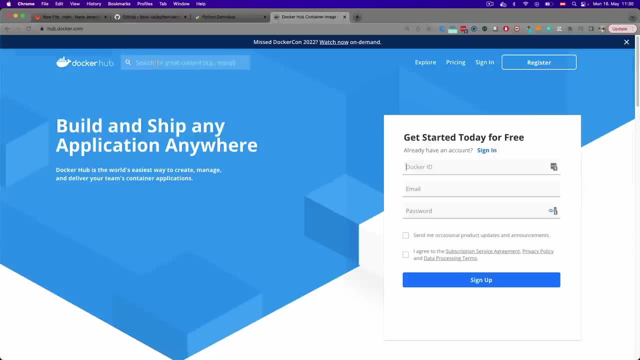 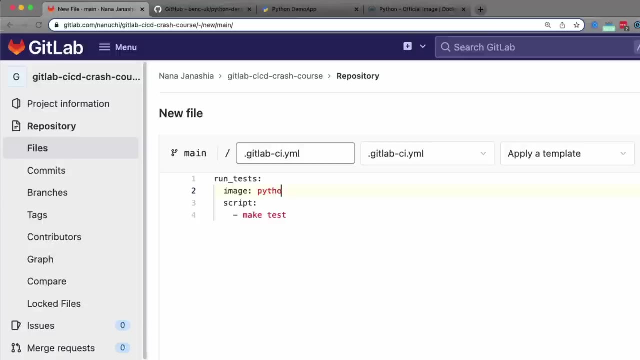 specifying whichever image we want And, as I said, in our case we're going to take the Python image from the Docker Hub, So let's actually find the official Python image. So it's going to be called Python and we can specify a tag here. 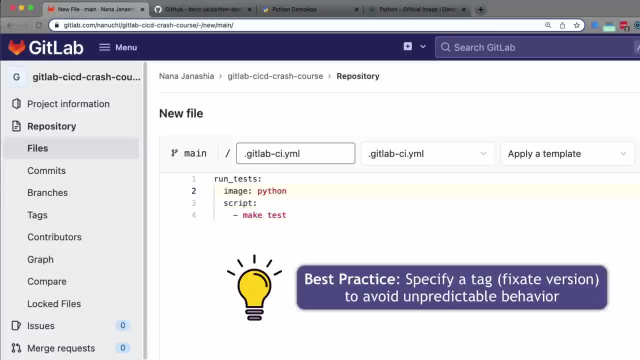 And it's actually a best practice to specify a tag instead of leaving it to the latest, because you want your pipeline to be consistent, Right? So instead of always fetching the latest image, and since the latest image gets updated all the time, you may get some unexpected behavior at some point when the latest image has some changes. 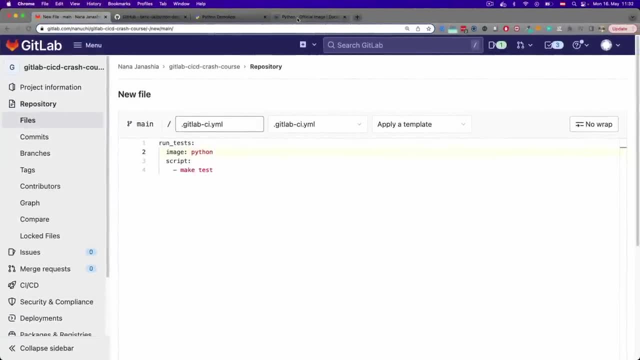 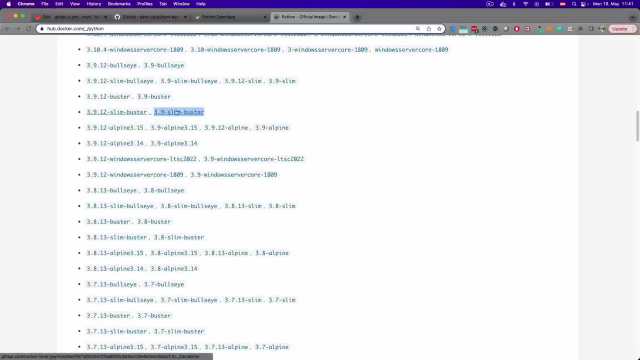 So we want to always fixate the version of the image and you have the list of those text to select from here. In our case, we actually need a specific version of three point nine, because that's what our application actually expects. So I'm actually going to go ahead and 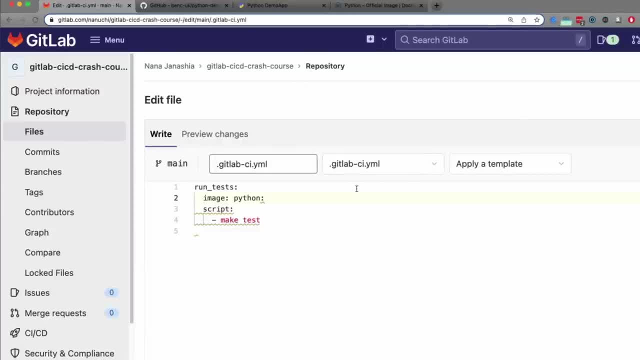 select this image tag and make sure that you do the same. So that's the version of the Python image our application needs. So now, when the GitLab runner gets this job in order to execute, it will see that we have overwritten the image. 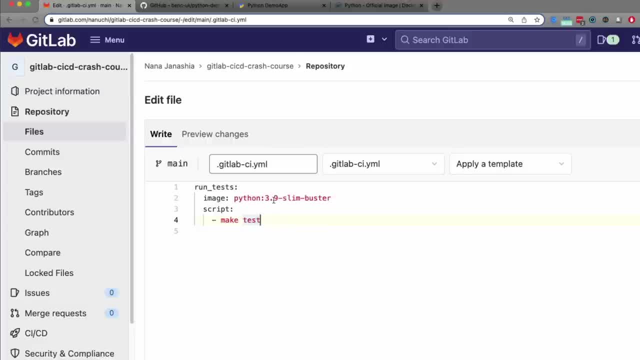 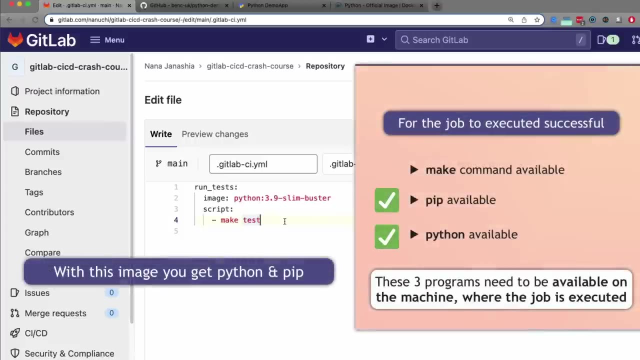 So, instead of taking Ruby, it will fetch Python image with this image tag and it will start the container with that image in order to execute the script logic inside that container. Now this image makes Python and peep tools available inside the container. However, we still don't have the make command. 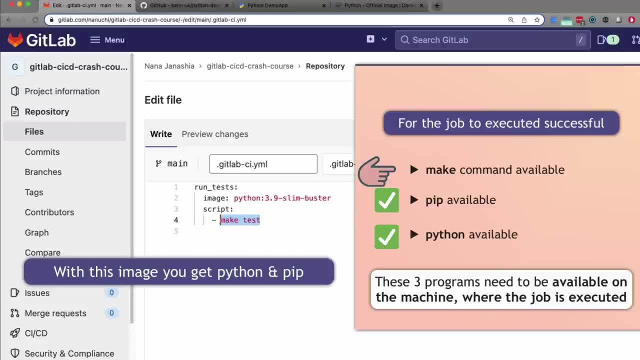 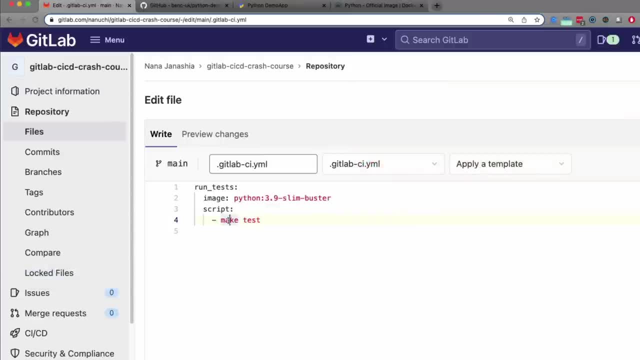 So we need that also inside the Python container to be able to execute this command. So how can we do that? A simple way to do that is to install the make command inside the Python container before the script gets executed, and we can do that using another. 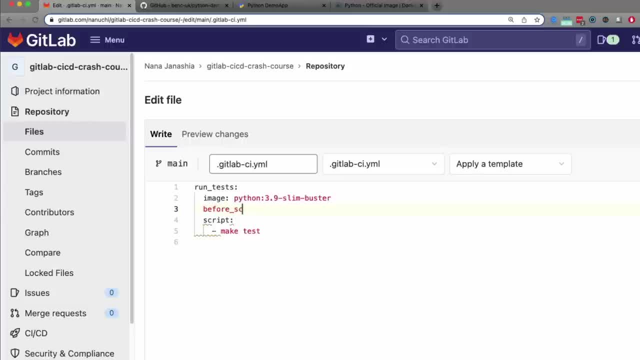 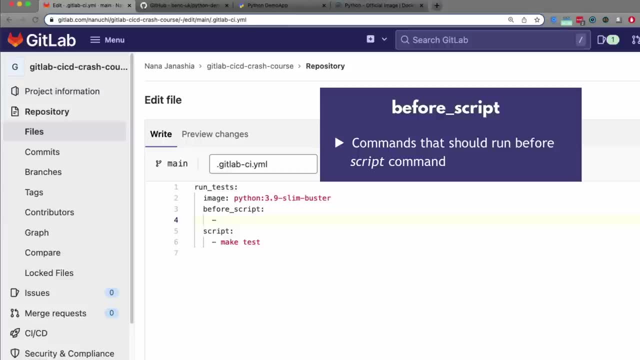 attribute on the job called before underscore script. So this is basically the same as a script with the same syntax. You can execute the same commands here as in script. But GitLab runner knows that whatever is defined here should run before the script. So this is usually used in jobs to prepare environment like set environment. 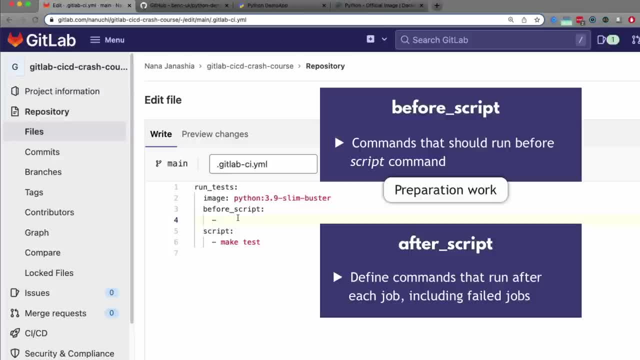 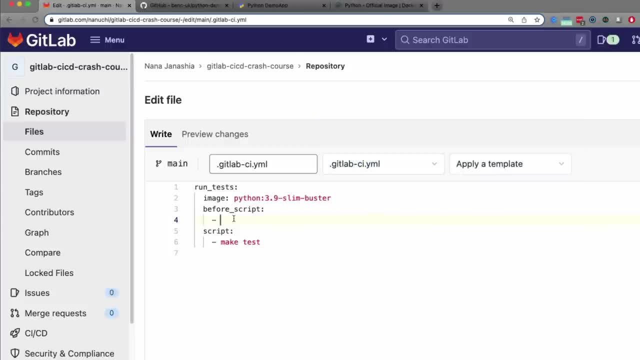 variables, create any temporary files, maybe fetch the data from somewhere or, in this case, install something that the main script actually needs for execution. So that's what we're going to do here, and we're going to install make just like you would install it on any Linux server with a package. 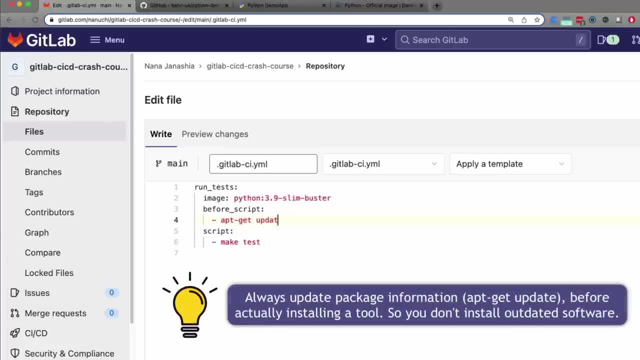 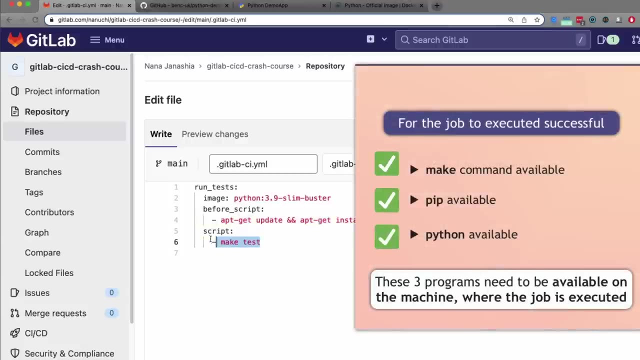 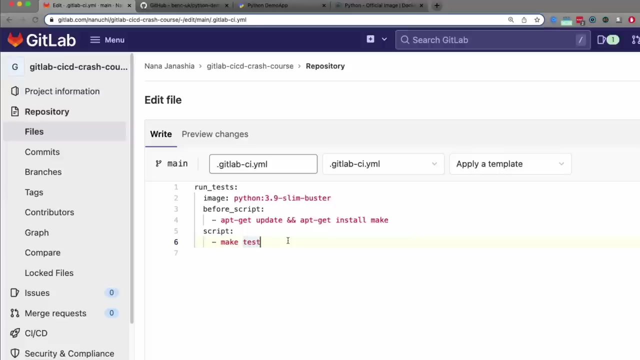 manager, apt-get, So we're going to do apt-get update and apt-get install make, So this will take care of installing make inside that container. So we will have all three tools that we need available in order to execute this command. So now, with this configuration, we already have a working. 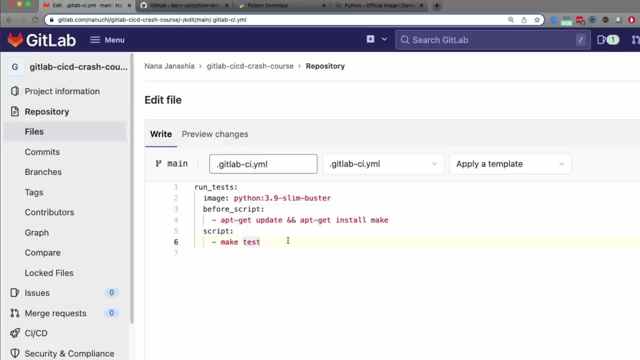 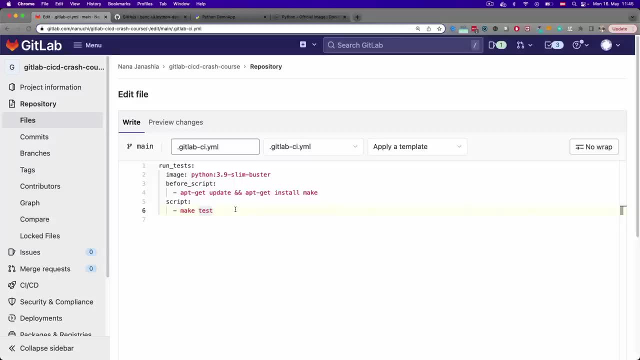 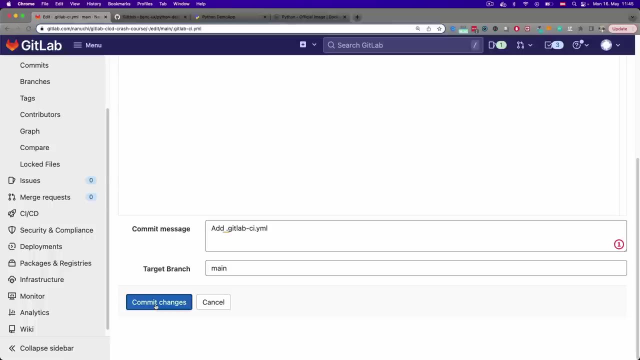 pipeline with just one job which runs tests, but still we have a valid working pipeline that we can execute for our application. So how do we actually execute the application? The only thing we need to do is simply commit this file And as soon as we commit the changes, 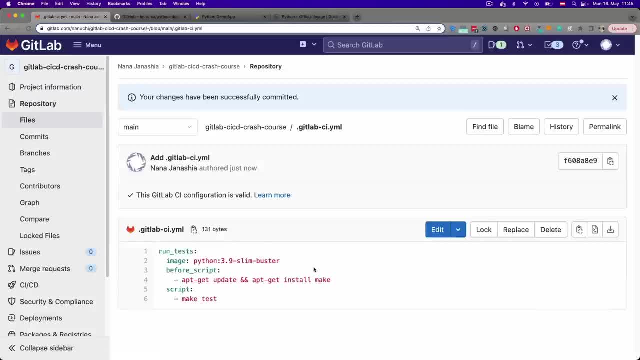 GitLab will actually detect that we have added a pipeline configuration and it will automatically execute the pipeline in the background. So the pipeline is actually already running. Now, where do we see the pipeline execution? Well, right here we are in the repository section, which lets you manage the files, commits, branches and so on. 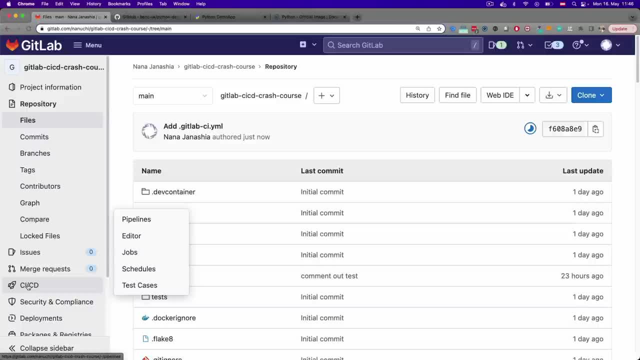 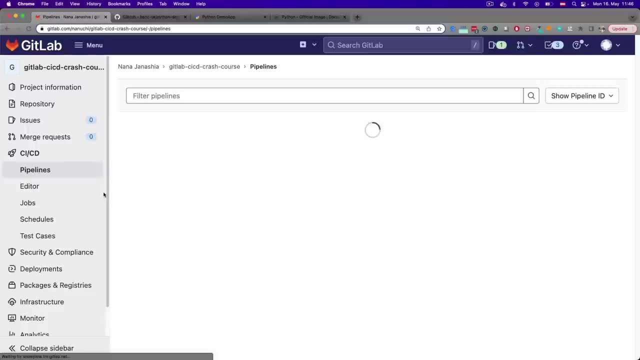 For the CI CD. there is a separate section that lets you manage the CI CD part of the project, And the good thing is you don't have to switch to some other view. You stay inside the project. You have all the configuration in one place. 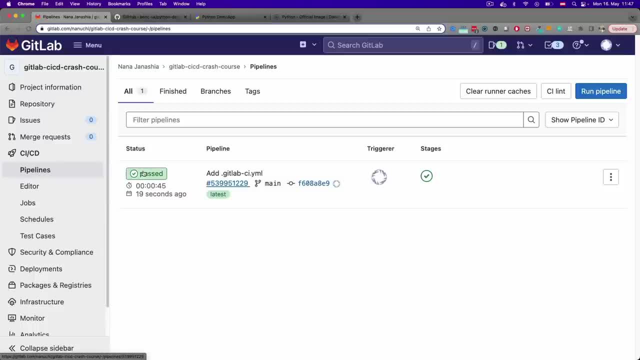 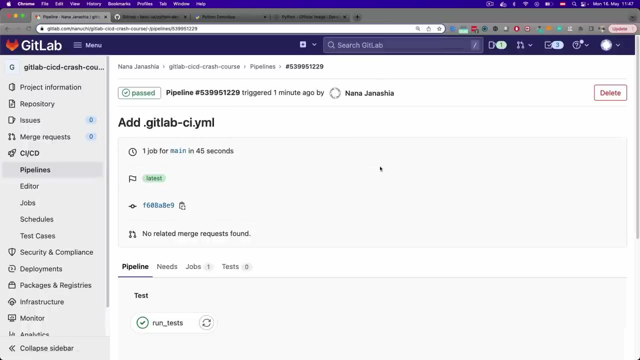 And the first tab here is pipelines And this is a list view. So this is going to be a list of all the pipeline executions for your project And we see that our first pipeline was successful. It has passed state And, if I click inside, 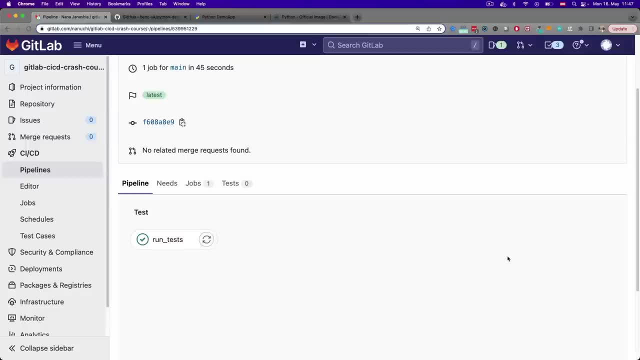 that's the detailed view of the pipeline. We actually see all the jobs that ran for the pipeline. In our case, we just have one job. We also have a separate job section where you can see the list of the jobs, And if I click inside the job you will see the logs, which is obviously. 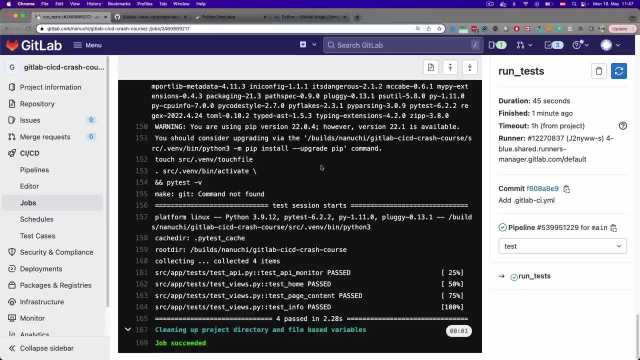 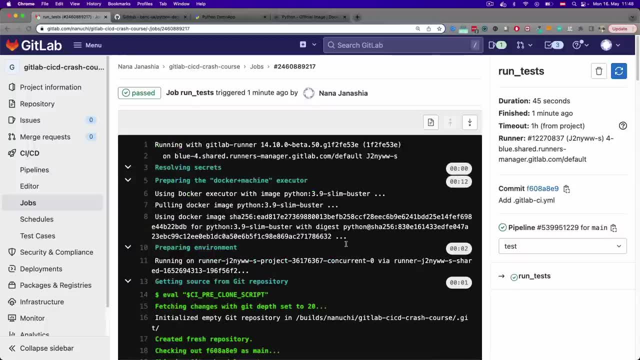 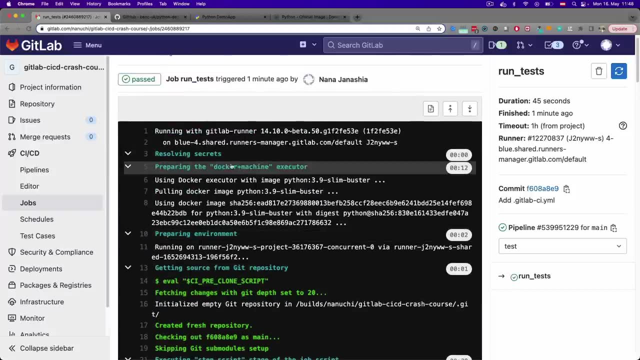 useful if the job failed, for example for troubleshooting and debugging. So let's actually take a look at our logs to highlight some interesting and important information. First of all, right here you see that the job is being executed using Docker. Right here you see using Docker executor with image. 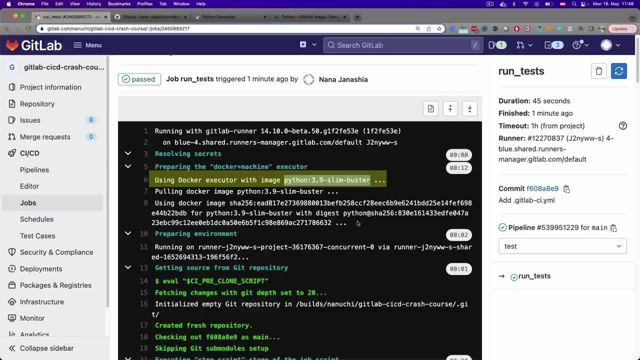 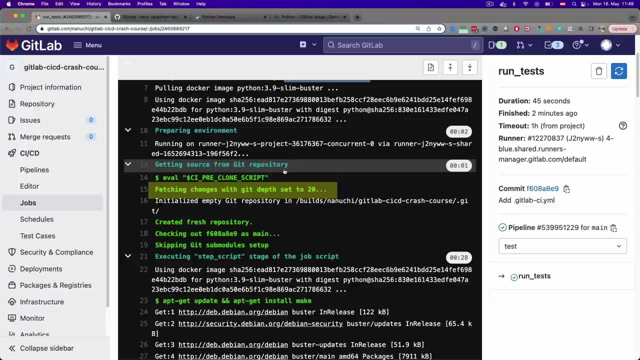 And this is the image that we specify. So by default it would have used Ruby, But since we overrode that, it is using image that we defined And it's pulling the image and starting the container from it. Once the container is created now it of course has to fetch the whole Git repository. 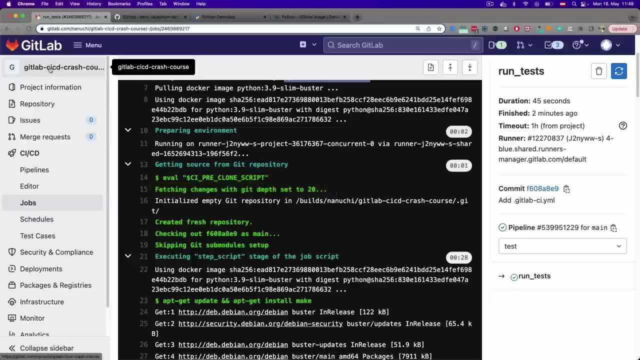 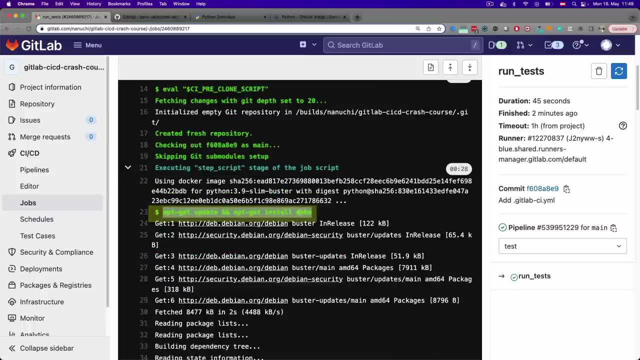 So this projects code, basically in that Docker container where we have the test files, dependencies file and everything else, to be able to execute tests, Right, But before the main script, the before script gets executed which installs make. And once that's installed, then make test command gets executed. 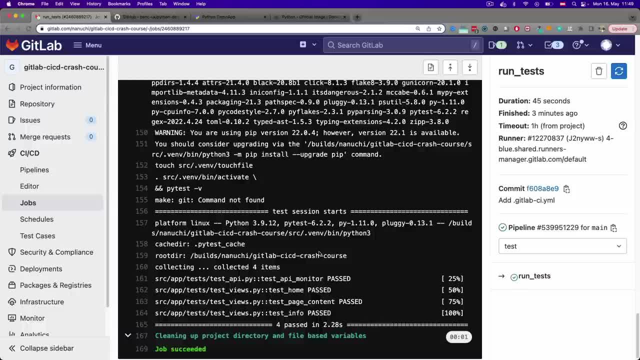 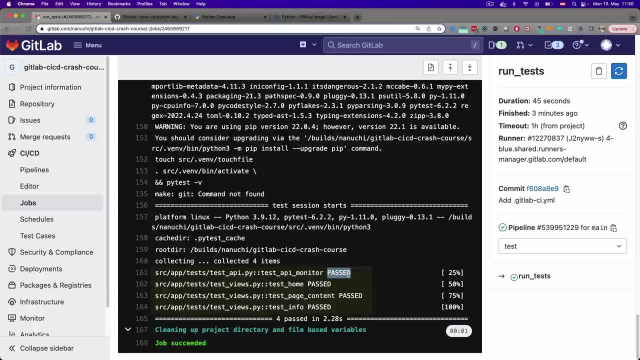 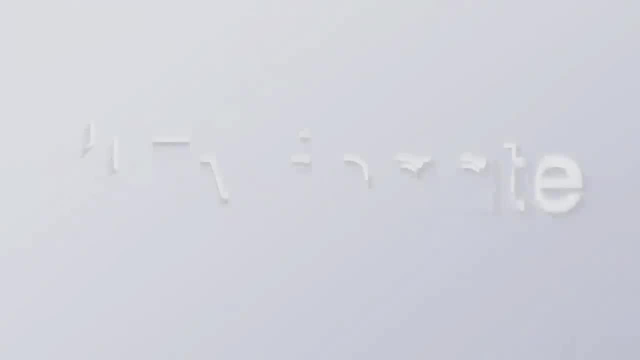 Then we have pip, install the dependencies And at the end we have our four tests. that all ran and they are in the past state. So the first step or first job of our pipeline is configured and working. Before moving on, I want to give a shout out to TwinGate. 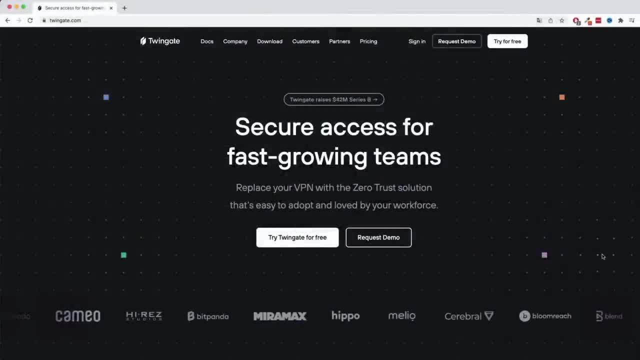 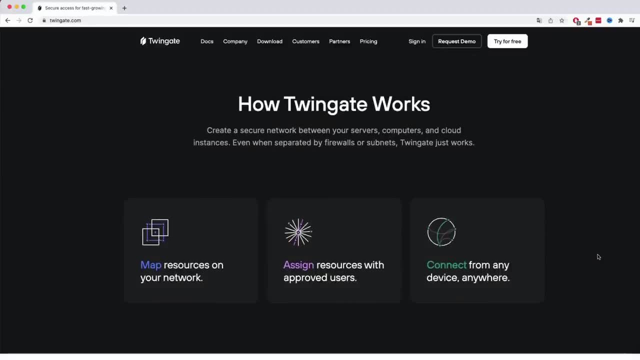 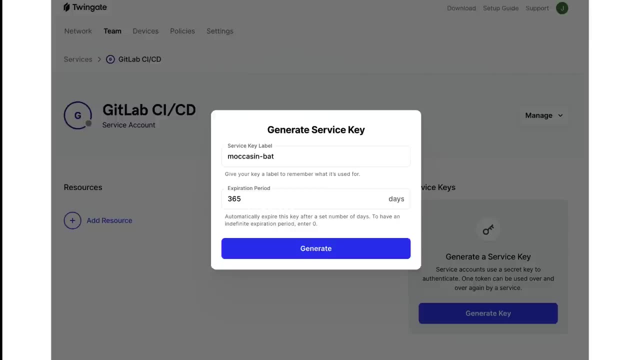 who made this video possible. TwinGate is a remote access service that allows you to easily access private services within any cloud or in your home lab. for CI city workflows that execute outside of your environment. TwinGate includes a service account feature that allows secure and automated access to your private resources. 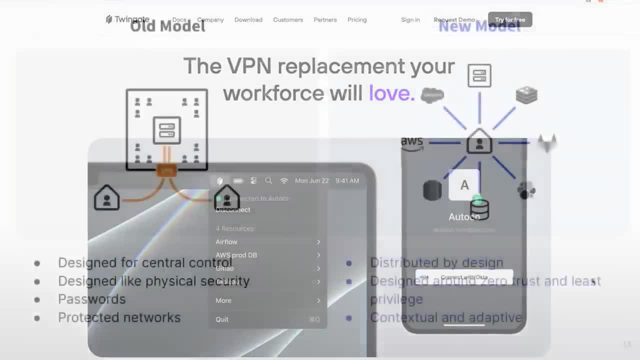 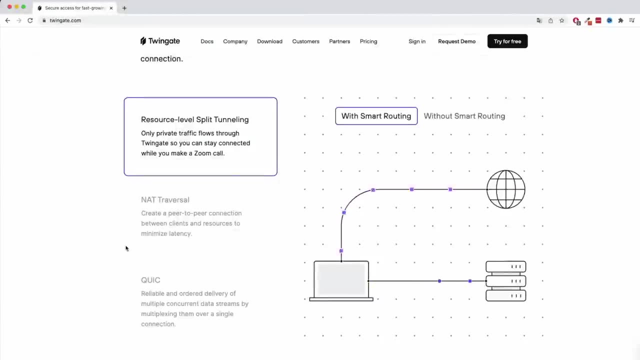 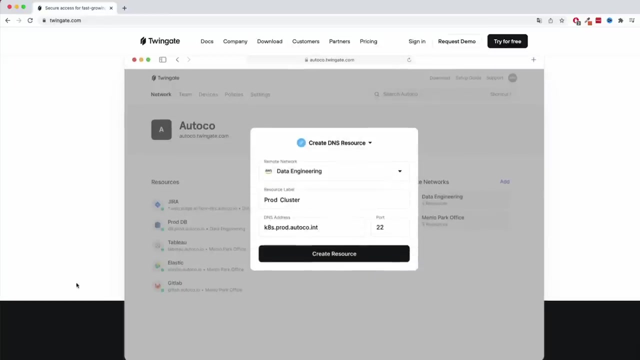 TwinGate is actually a modern alternative to a VPN that is easier to set up, offers performance and is more secure. if you need to create a workflow to deploy into your private Kubernetes clusters or if you have internal databases you need to access, then it is an excellent choice with TwinGate. 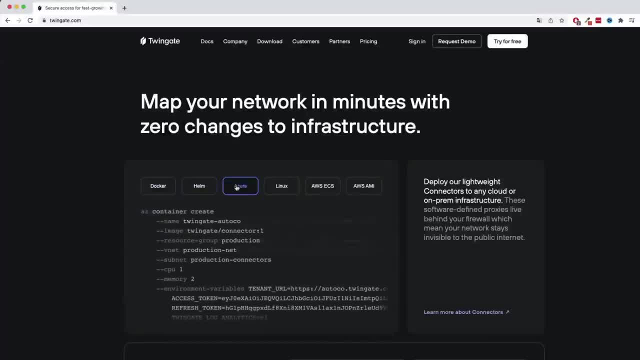 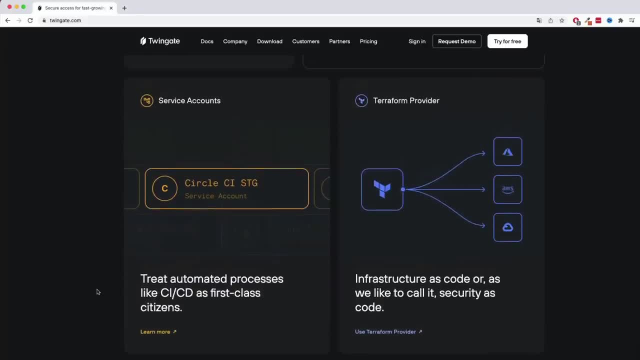 You don't need to open any ports on your firewall or manage any IP whitelist. You will also find providers for Terraform and Pulumi so you can fully automated into your existing stack. If you want to try it, you can use their free tier and get. 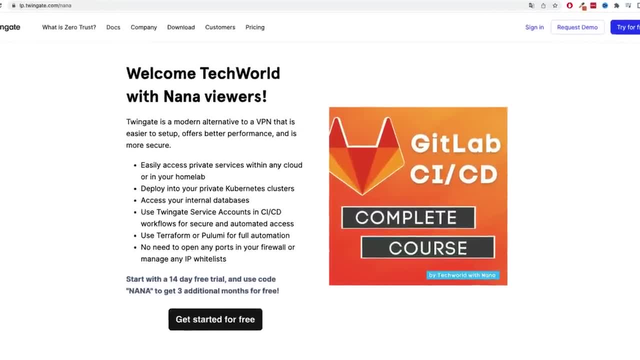 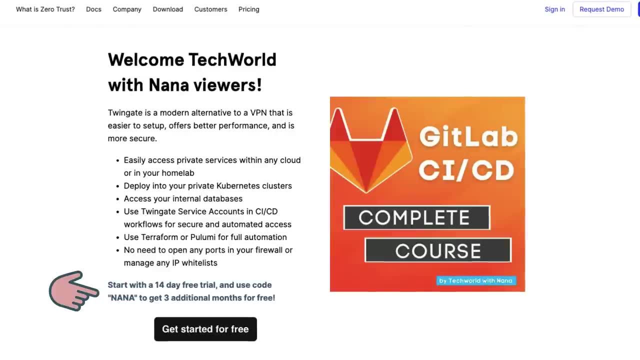 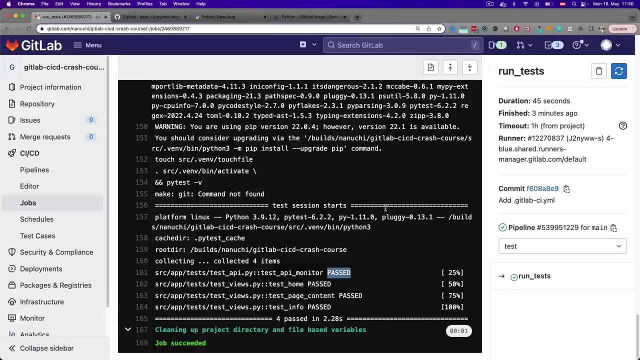 started for free, or? TwinGate has actually provided a special offer for my viewers. You can use the code Nana to get three months free of the business tier, in addition to their 14 day free trial. So now let's go back to the pipeline and add the next job that will build. 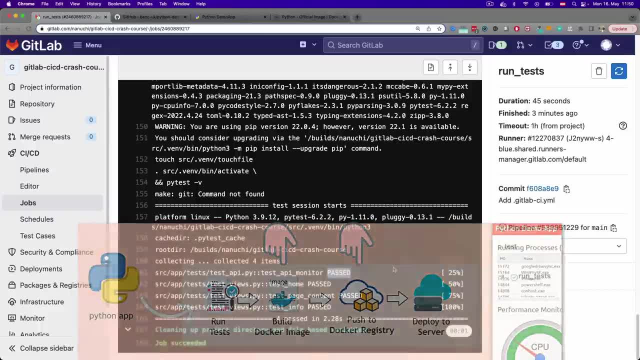 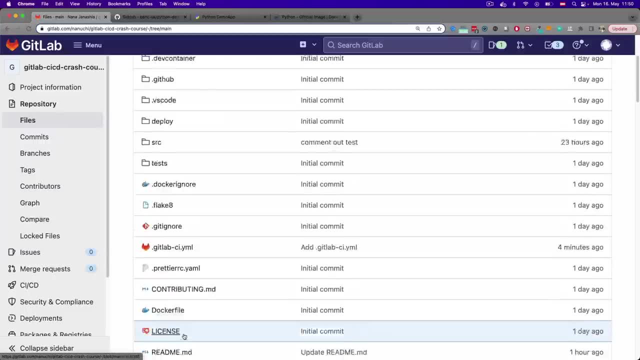 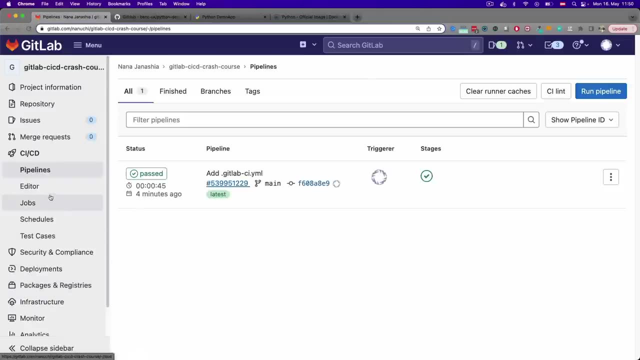 and push a Docker image of our Python application and to switch back to our pipeline code, We can go to the repository and basically in the GitLab CI file, or we actually have a shortcut here in the CI CD section with the editor tab. that takes you directly. 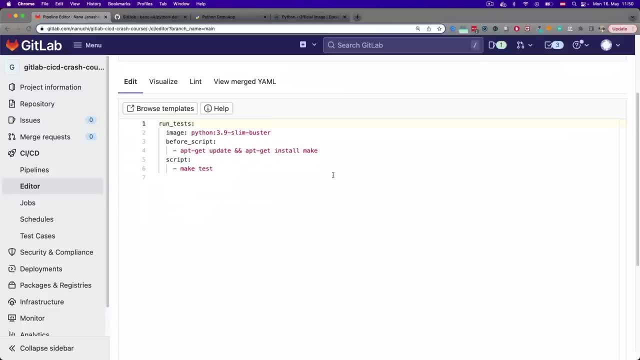 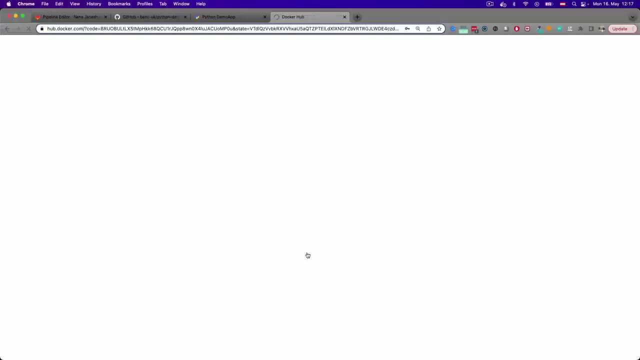 to your GitLab CIyaml code in the edit mode, So you can continue working here on your configuration. Now let's create the next job, where we build a Docker image and push it to Docker Hub's private repository. So first of all, to have a private repository on Docker Hub. 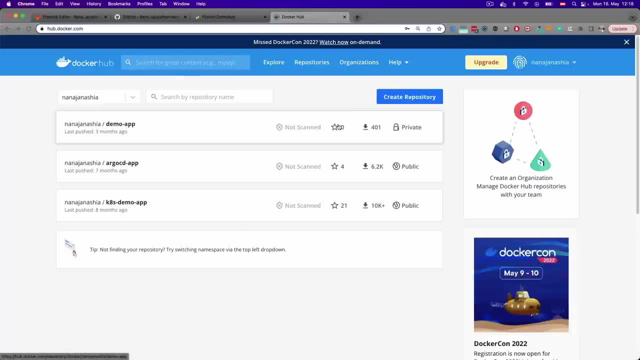 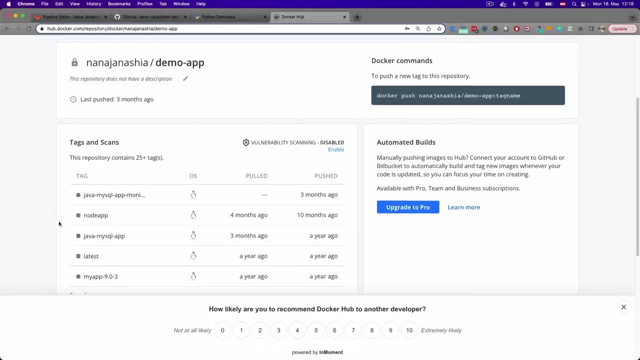 you can simply sign up and create an account by default in the free version. Basically, you get one private repository. So that's what we're going to use- And I have some other apps here, but that's what I'm going to use for the demo. 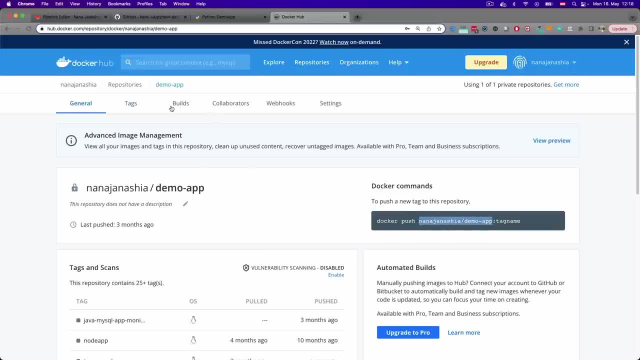 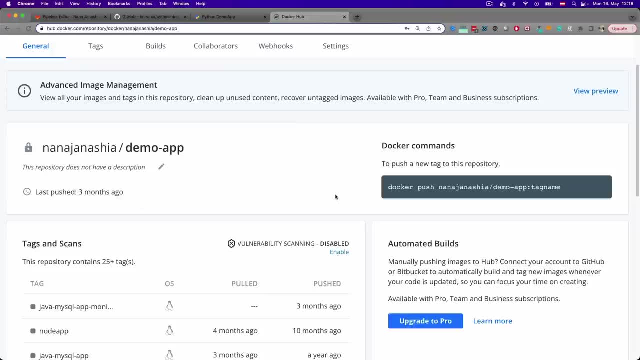 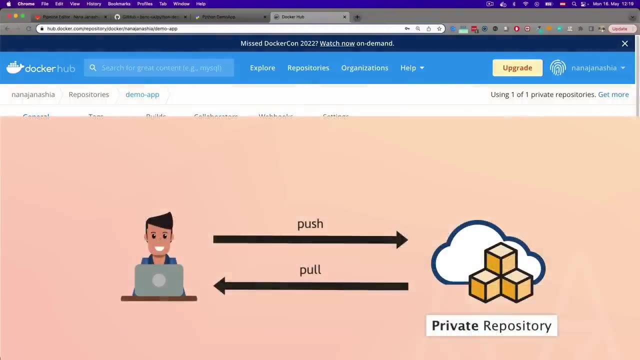 So that's the address of my private image registry on the Docker Hub And I'm going to be pushing an image that the pipeline builds into this repository. Now, in order to push an image to a private image repository, we need to log in into that repository first, because of course we don't want. 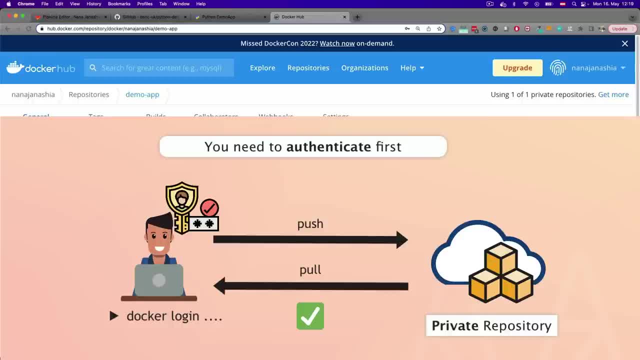 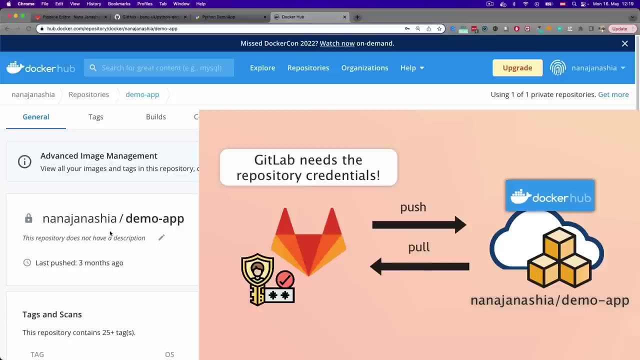 to allow anyone to pull and push images from a private repository. It has its credentials and you have to log in before you actually push an image or pull an image from it. So we would need repository credentials for this repository to be available on GitLab. 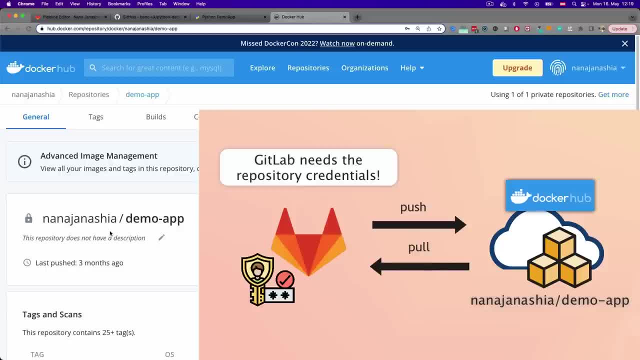 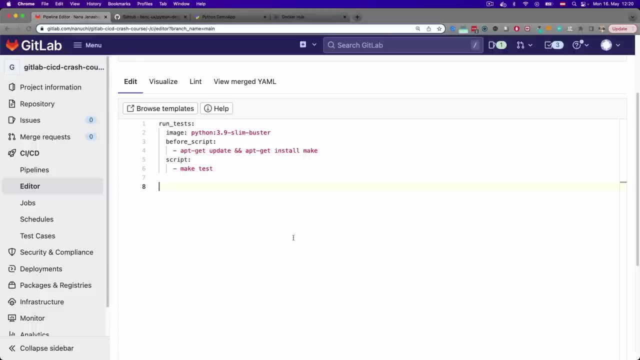 So that GitLab runner can actually log into the registry before it pushes the image. And the credentials are actually username and password of your Docker Hub account. So this is what we're going to use to log in to the private repository, And of course we don't want to hard code. 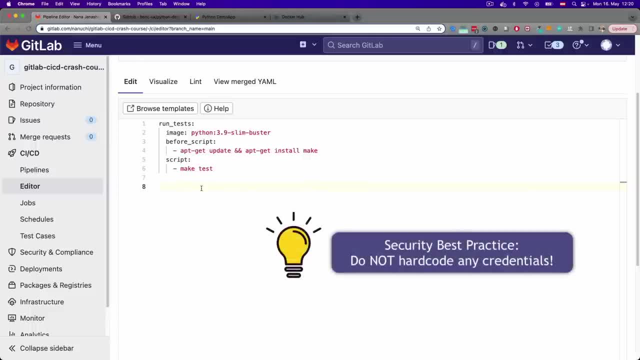 those credentials, that username and password, inside the pipeline code, because, again, this is part of the repository, So anyone that has access to the repository will be able to see that. plus, it's going to be in plain text and so on. So it's not secure. 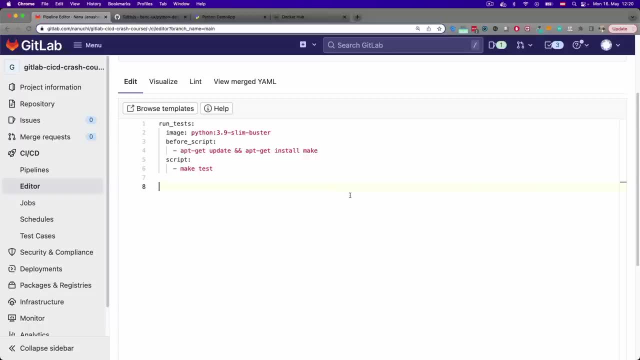 So we want to create what's called secret type of variables that will be available in our pipeline, And the way it works on GitLab is in the project settings. So if you scroll all the way down, you have this settings tab here where you can. 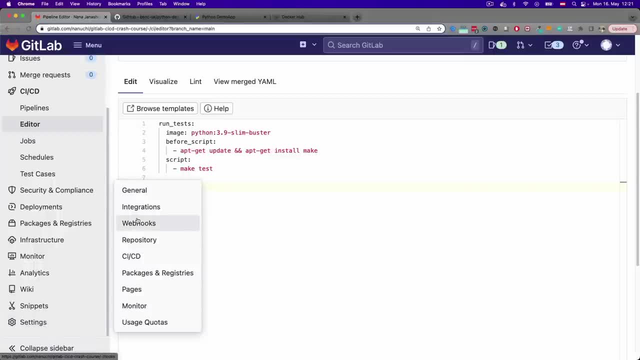 actually configure some of the administration settings for different parts of your project. So you have settings for the repository, you have settings for CICD and so on. And if you're wondering why it is actually separated, So why don't I have the settings here directly in the CICD or the repository? 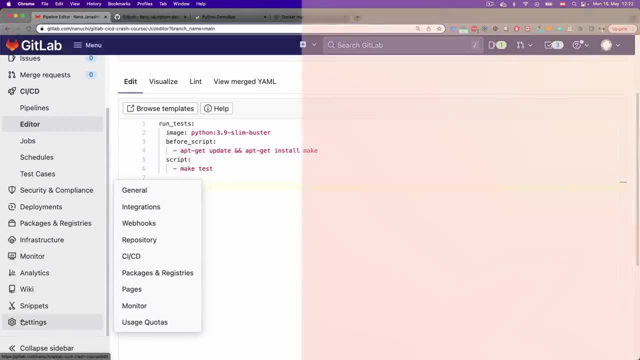 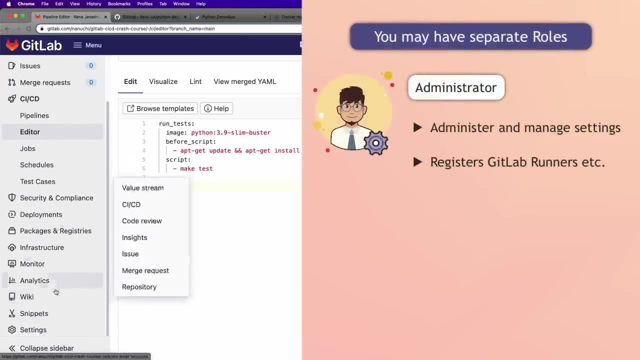 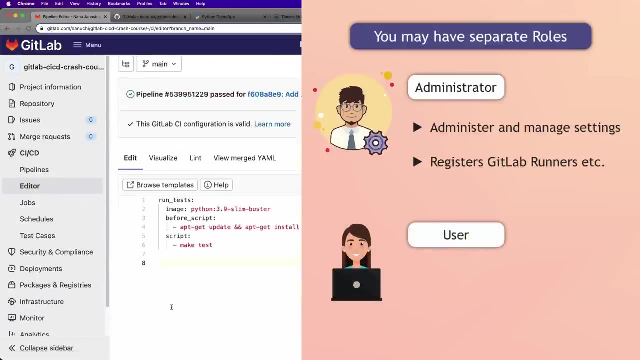 settings here directly in the repository, is that this would actually be two different roles. So for your project, you may have project administrators to actually administer and manage the settings of the project, And you will have the project users. These are your developers. These are your developers- junior developers, interns, senior developers. 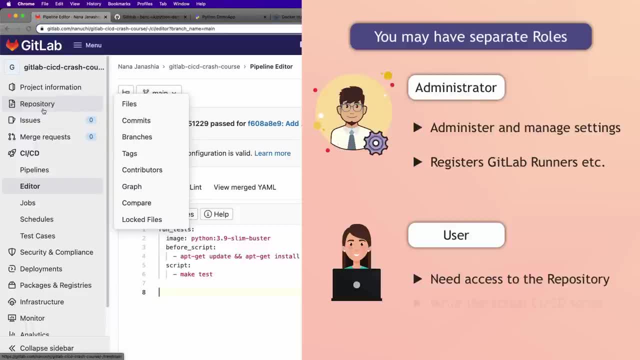 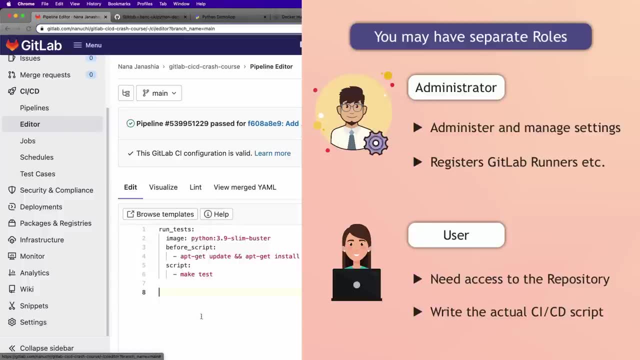 whoever needs access to the project to work in it, Right. So you may want to separate those permissions and have just a dedicated people who have access to the settings, responsible for that part, And then your developers, or most of the developers, do not see the settings at all. 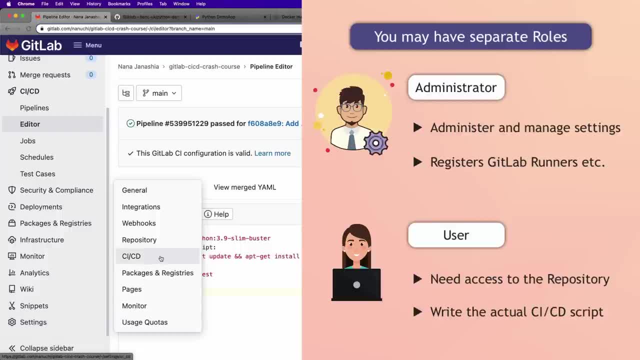 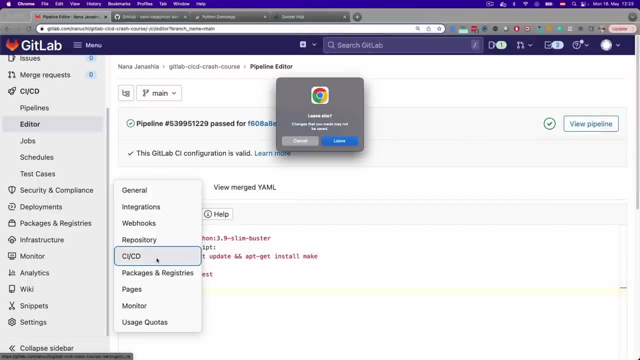 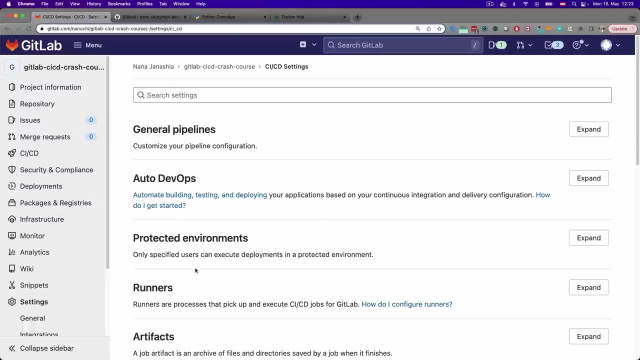 So that's basically the idea of having this CICD setting separately and the pipeline configuration separately. So in the settings of the city, if I click inside and we can leave the edit mode of the pipeline, that's fine. Right here we have again different settings for our city pipelines for. 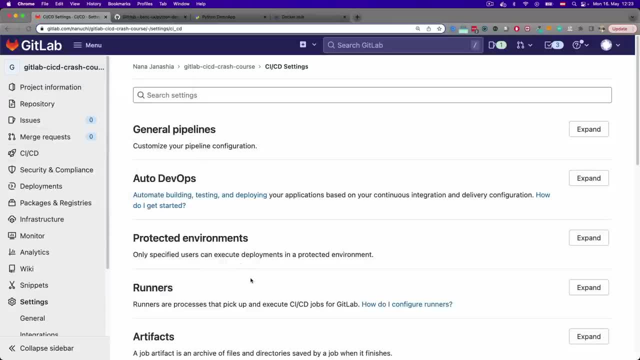 the project which an administrator of the project can configure. So obviously this would be someone more experienced and knowledgeable about how to manage all this. That's why you want to give maybe a limited set of people permission to see and modify the settings of the project. 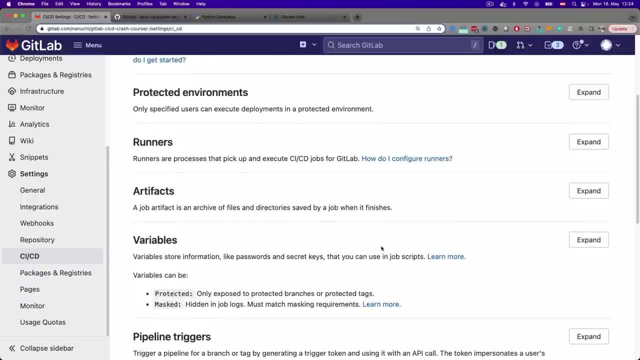 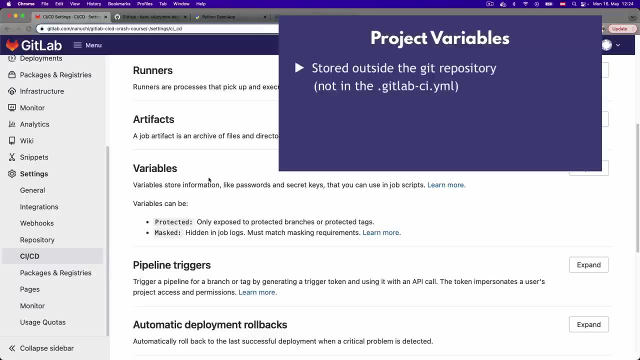 So, right here, we have multiple things we can configure, And one of them is project variables, And this is where we can create custom variables. This could be secret variables like password, username, but also just normal variables, Right, And this will be then available inside the pipeline code. 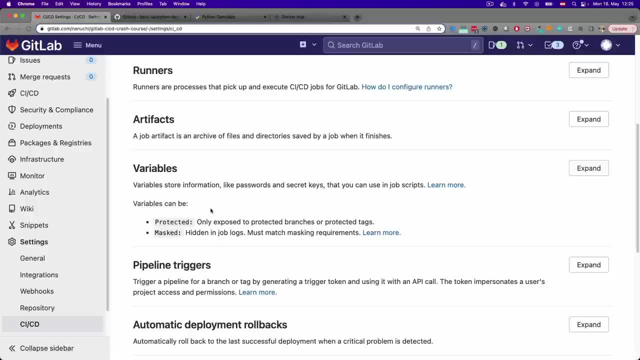 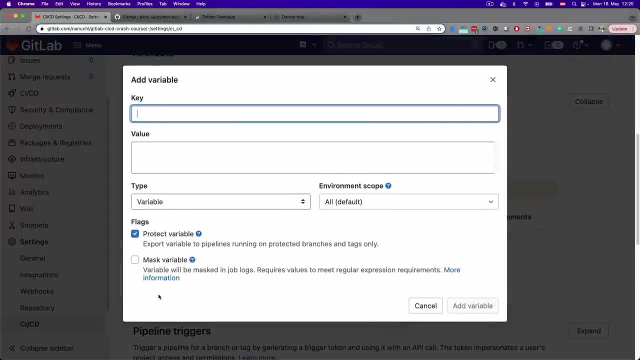 So we can actually reference those variables in our pipeline configuration. So, if I expand this, we can create variables here. click on a variable and we're going to define Docker user, or this could also be registry user, And here we're going to have the value. 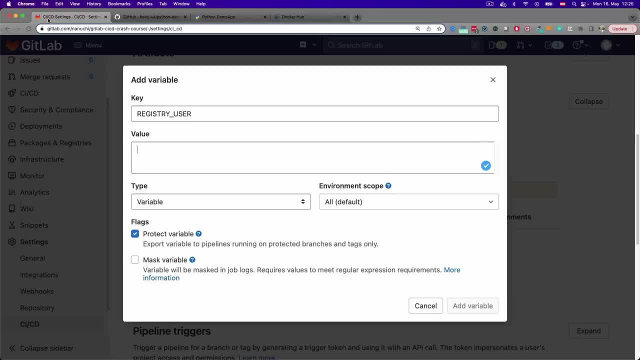 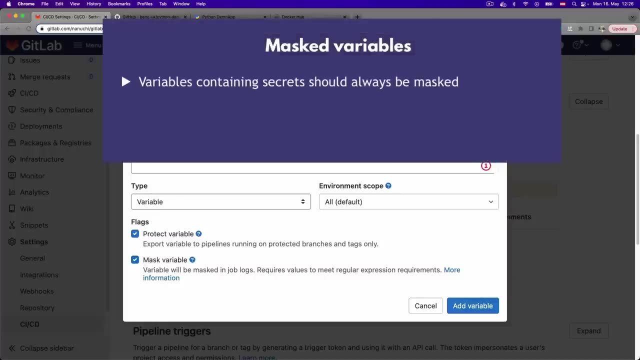 So I'm actually going to copy that And this is the Docker ID, So your username on Docker Hub, and the type variable, and we're going to click on mask variable. So what this will do is whenever the variable is referenced and used inside a job- for example, job execution of the pipeline- the value will be masked. 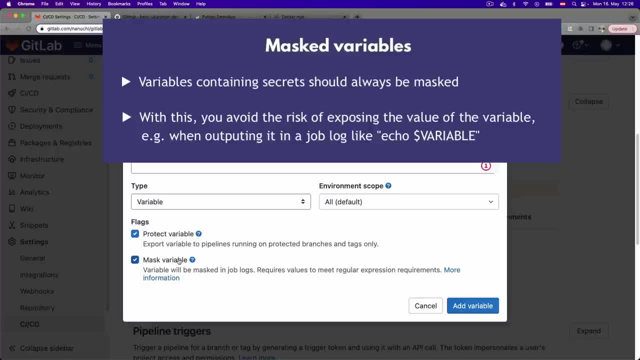 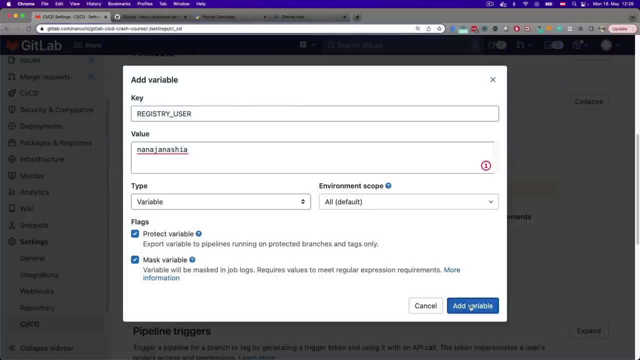 So it's not going to be visible in the job logs, which is, of course, more secure. So, for secret or sensitive data, we're going to check that. So that's it. That's going to create our first variable, And now let's also create registry password. 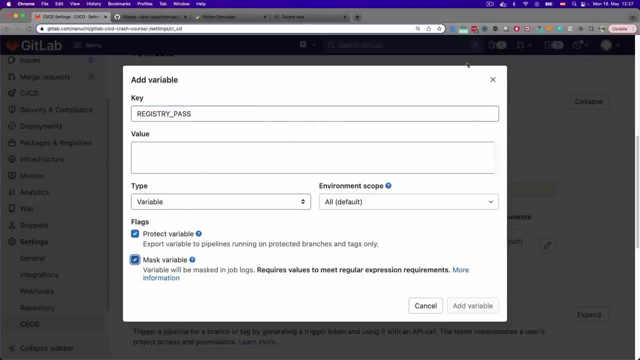 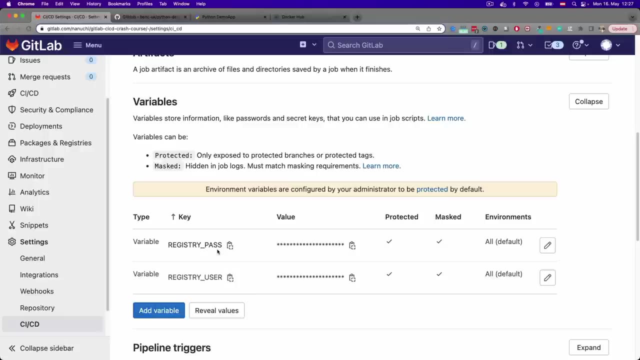 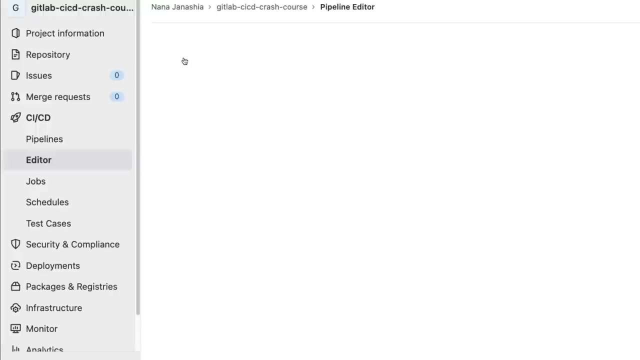 Let's call it registry pass, And again mask the variable, And for that you're going to grab the password. And there you go. We have those two variables and now we can actually reference them inside our pipeline configuration. So I'm going to go back to the editor and right here we're going to create a job. 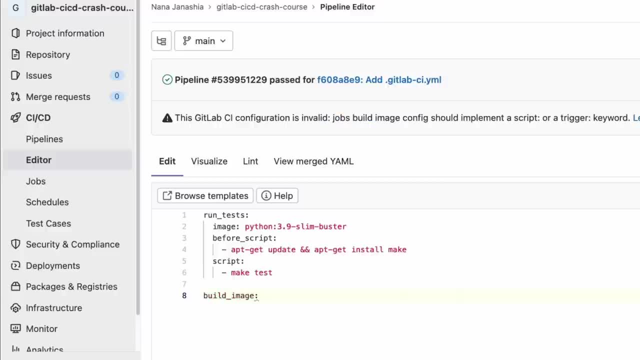 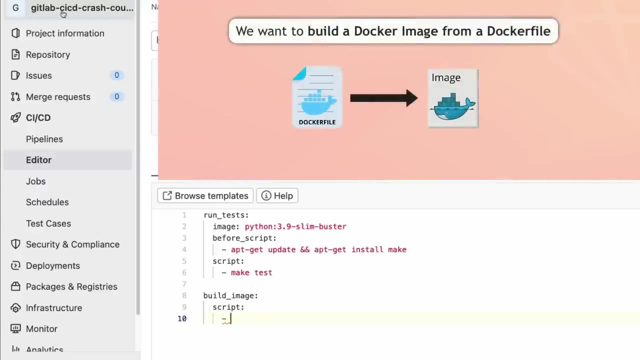 called build image. Obviously, you can call it whatever, but I'm going to call it build image And let's define the main script. So what is the main logic that we want to do in this job? Well, first we want to build a Docker image of our Python application from Docker. 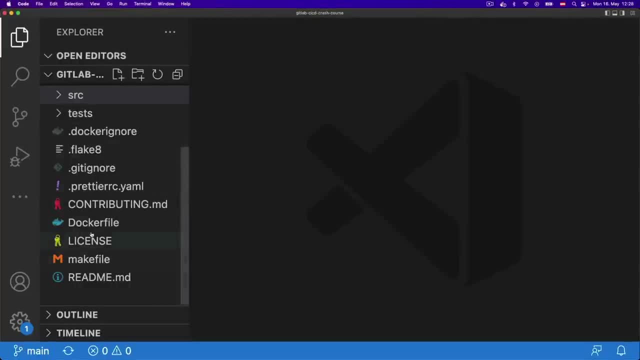 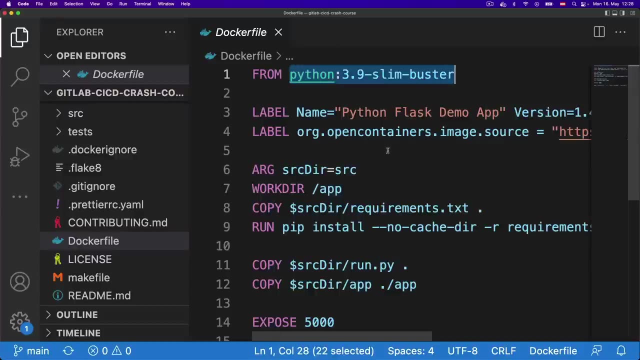 file, and we actually have a Docker file as well in the project. So right here in the root of the project, we have this Docker file that defines the Python base image, which is, by the way, the same as we used right here to run tests. 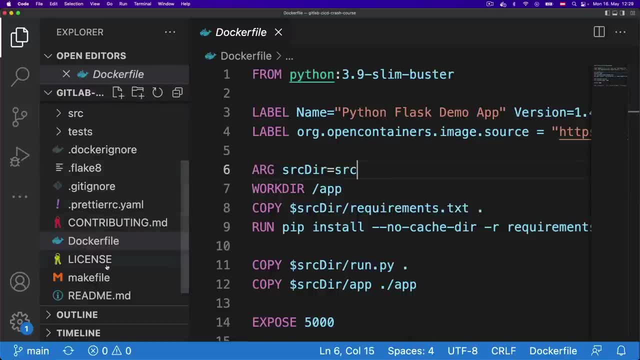 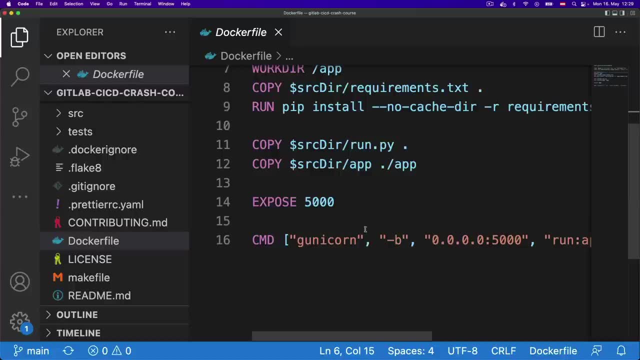 And the rest of the configuration is simply copying the relevant files inside the image, installing all the dependencies from the requirements file and then finally starting the application on port 5000.. So that's what's happening. We already have the Docker file, so we're going to use that to build the image. 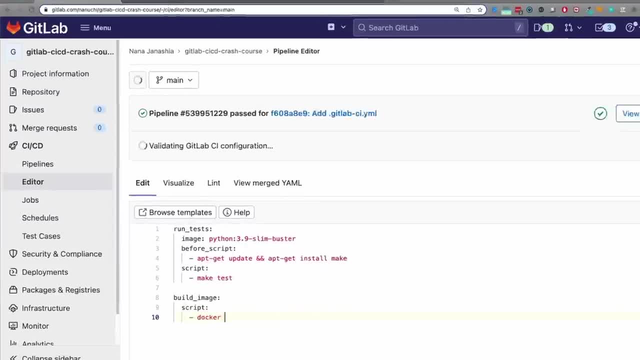 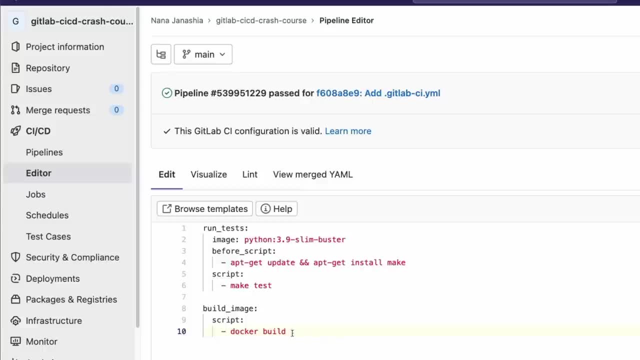 And, as I said, it is in the root of the project. So we're going to do Docker build And, since our GitLabCIEyaml file is also in the root, this is going to be the current location of Docker file, which is the current directory. 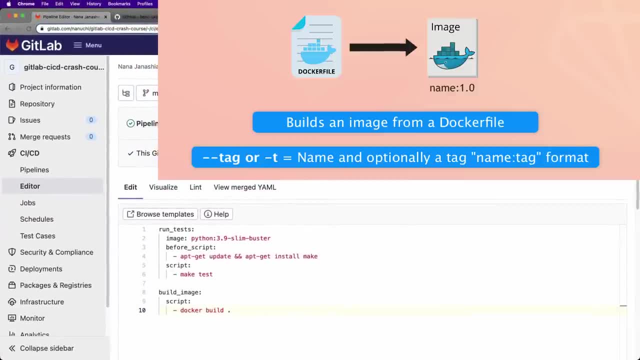 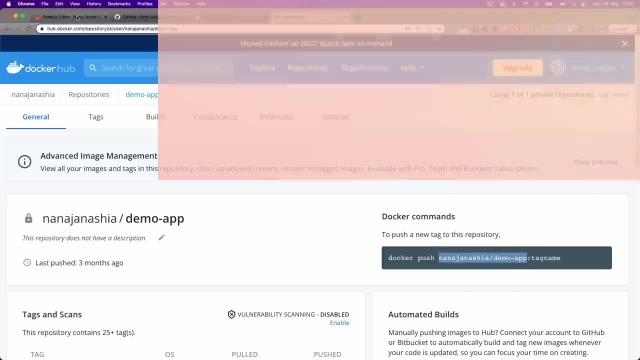 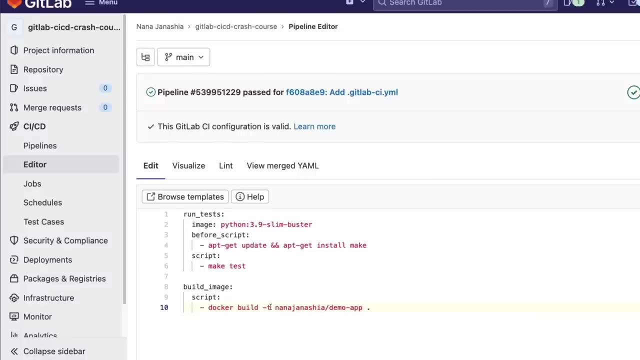 Now, in order to build an image that we can later push into our repository, we have to tag that image using the repository name. So I'm going to copy that and I'm going to add minus T. So that's for tagging the image with the repository name. 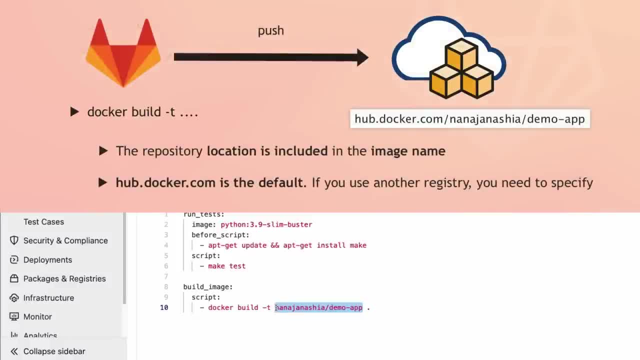 So in Docker the name of the image includes the repository name, so that Docker knows where to push that image. when you execute Docker push command And you also need to have a tag, just like here, Right, And in this case let's hard code a value here. 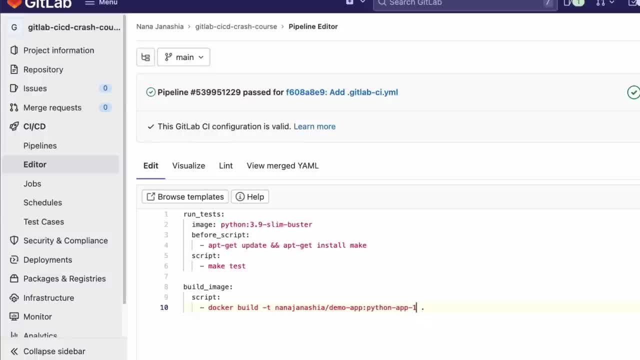 Let's do Python App 1.0. And this will be the complete name of our image. And then, once we build that image, we're going to do Docker push because we need to push that image and I'm going to copy the name. so that's going to be the push image. 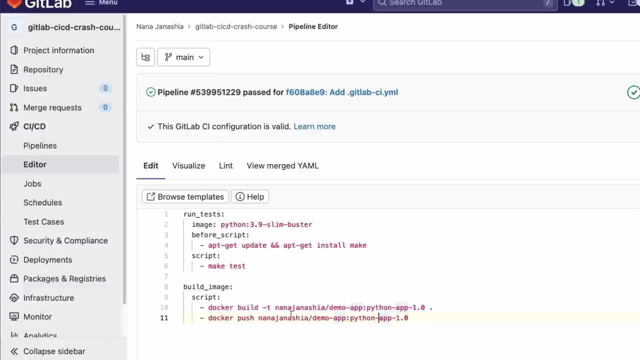 And, as I said in Docker, the way Docker knows where you want to push that image or the address of the repository is inside the image name itself. So it knows. on this Docker registry you have a repository called this and you want to tag the image using this specific tag. 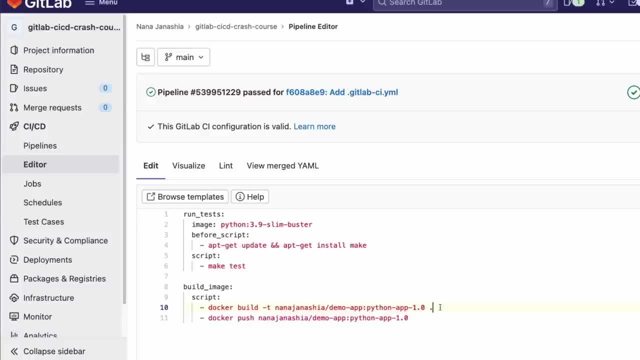 But before we can do Docker push, obviously we need to authenticate with the repository, otherwise it's not going to work. So right here, before push, we need to execute the Docker login command, which takes username and password as parameters. So we have this, you for username. 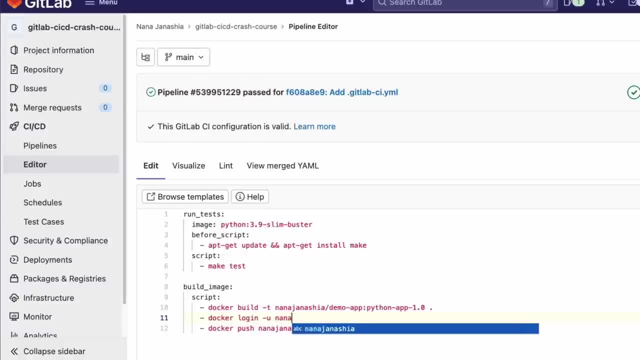 And now, instead of hard coding the value here, we can reference the variable that we created in the settings, called registry user, And we can reference it super simply using the dollar sign and then name of the variable, registry, underscore- user, And we also have the password and that's going to be registry pass. 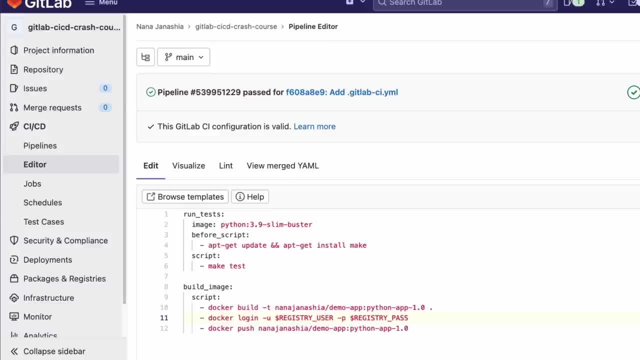 That's what we called it, And for Docker Hub. So if we're using Docker Hub, we don't have to specify the registry, because Docker Hub is the default. But if we're logging into some other registry, like on AWS, ECL, for example- 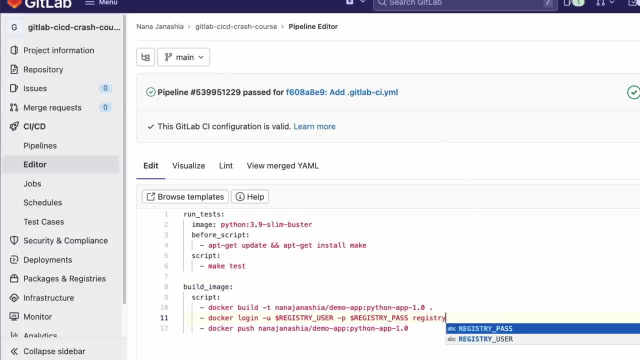 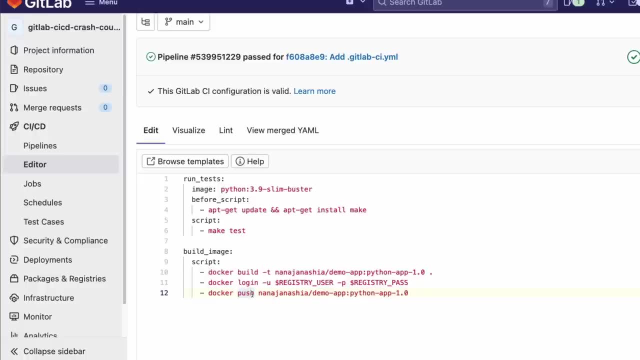 then we would have to specify the registry right here. But, as I said, Docker Hub is a default, so we don't have to do that. And since the Docker build and push, our main commands and Docker login needs to be executed before we can push to the repository, we can actually set it. 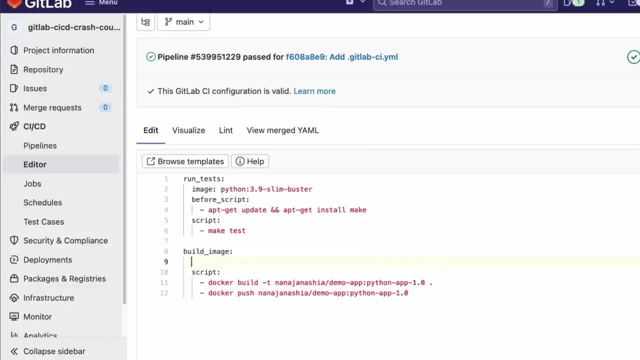 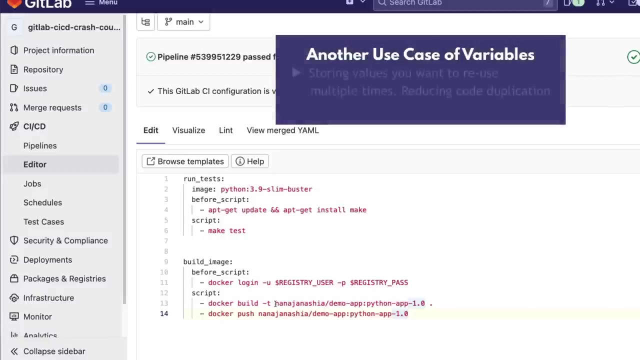 in before script section. Like this: so we have our main commands and supporting commands, so to say, separated. like this: So that's our job configuration. And, by the way, when we're repeating the values inside our pipeline, we can also extract them into custom variables. 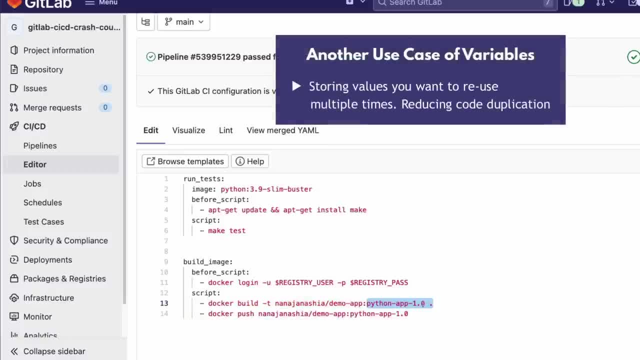 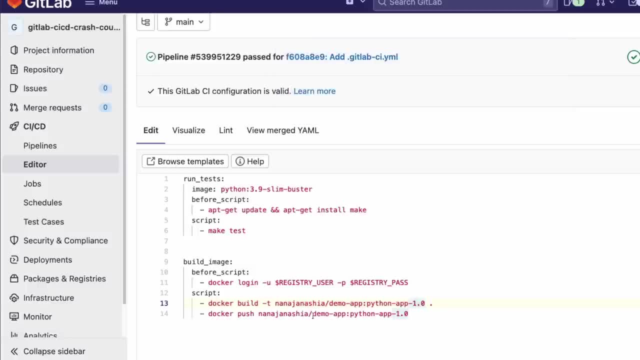 So for example, the repository name and the image tag could be variables inside the pipeline. then we can then reference here instead of hard coding them and then repeating the value multiple times, And for that you don't have to go to settings and create these global variables. 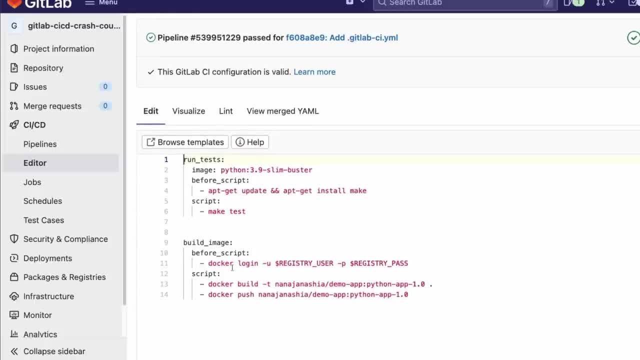 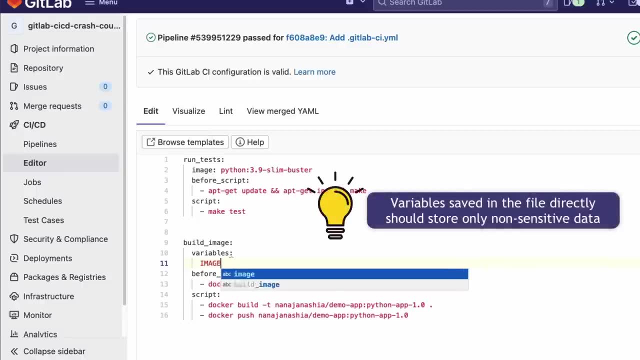 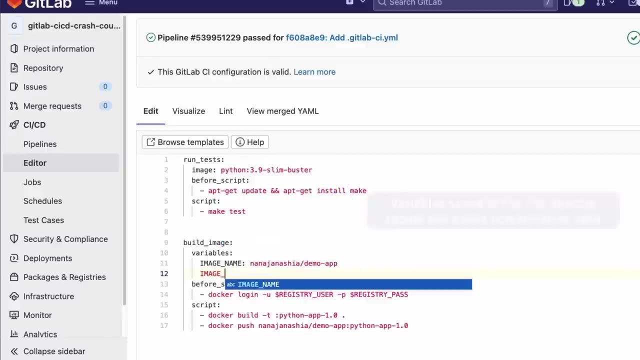 You can simply define them here inside the pipeline configuration, Either on a job level, like this, So we would have something like image name, And this will be the image name, and image tag, Like this, and then we just reference both variable values using the same syntax. we 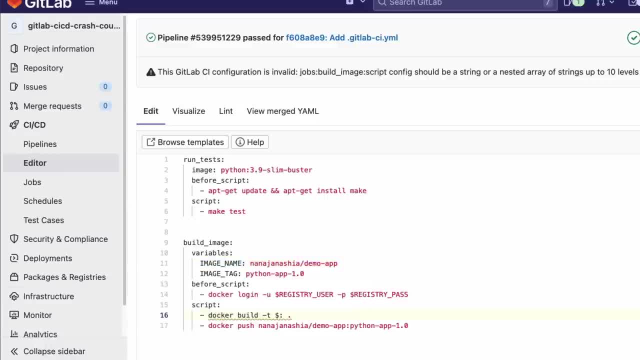 use to reference the variables from the city settings. So with dollar sign, variable name and image And And the same here. you know that the uppercase letters with underscore is just a standard. You can obviously call it whatever you want. It could be also image name, doesn't matter. 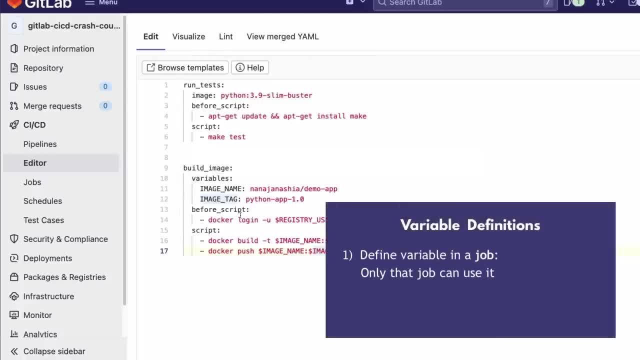 And, as I said, you can define the variables on a job level or if you have other jobs that also reference this image, name and tag, for example in a deploy stage, for example, if we also need the same variables, we can extract that and make it available. 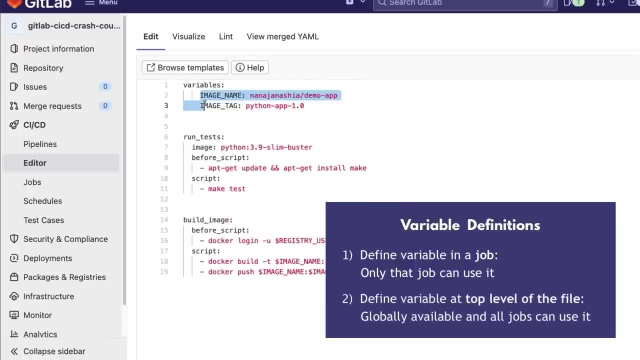 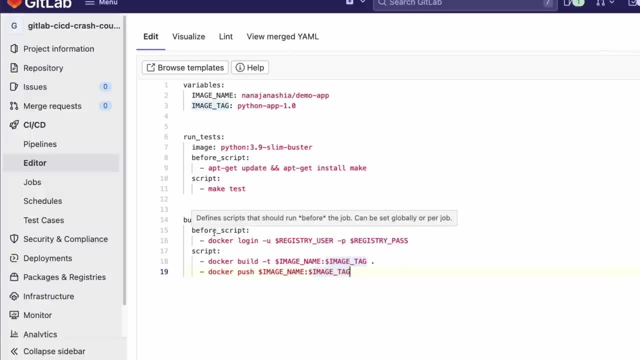 On a pipeline level for all the jobs Like this. So, even though our job logic is complete, we still have to make sure that the job execution environment of this specific job has all the needed tools to actually execute these commands. So, as we know, on managed GitLab runners. 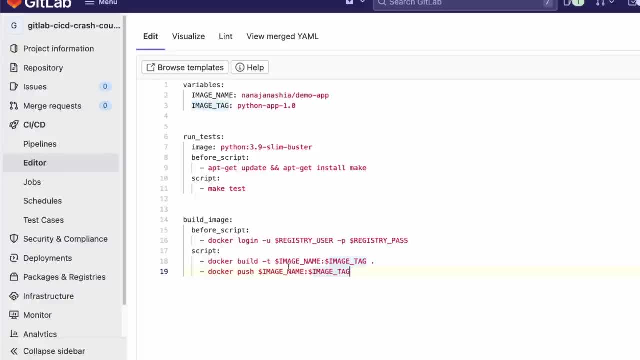 all our jobs will run in the Docker container and in that Docker container we need to have the commands, whatever we're executing inside the job, available. Otherwise it's going to say it cannot find the command Right. So in this case we have a little bit of specific situation. 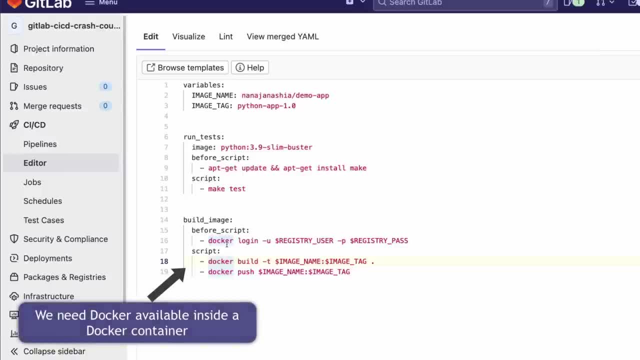 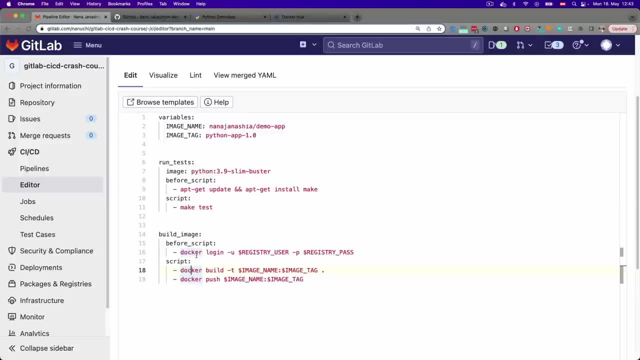 where we need Docker to be available inside a Docker container, And that is what's called Docker in Docker concept. So, within a Docker container, you have Docker daemon and Docker client, both available in order to execute the command, And again, the default is a Ruby image, but we need an image that 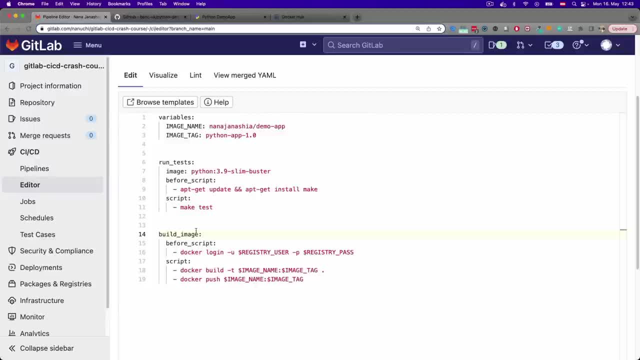 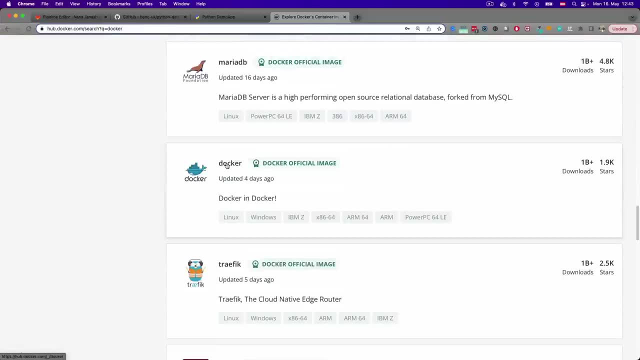 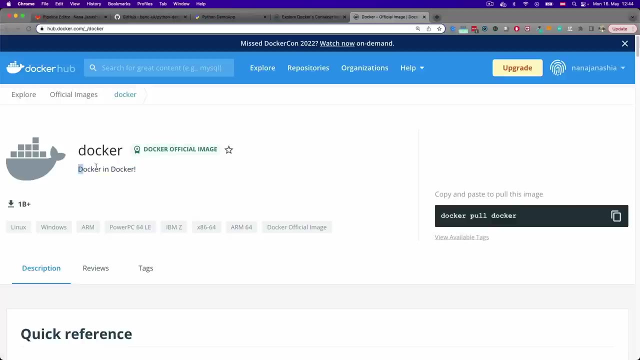 will have Docker available inside the Docker container And there is actually an official image of Docker Right here. That is meant exactly for that scenario where you have Docker in Docker. So you build a Docker container with a Docker image, which makes again Docker. 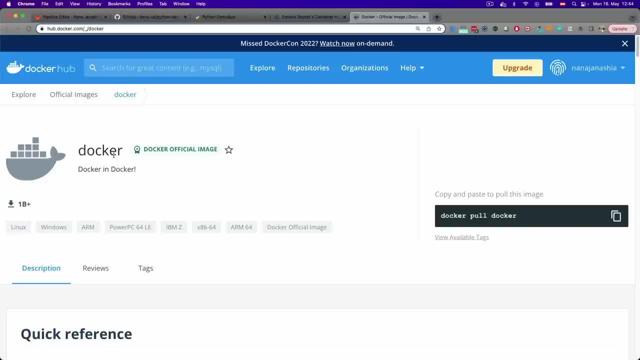 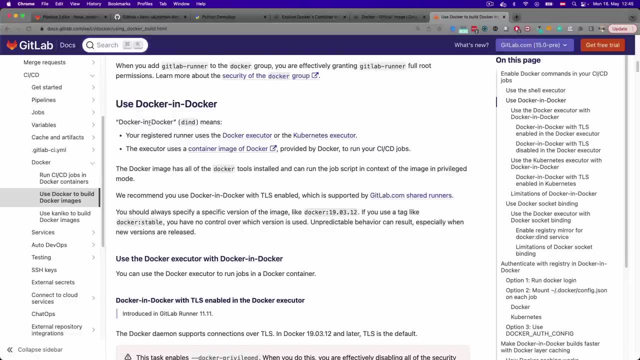 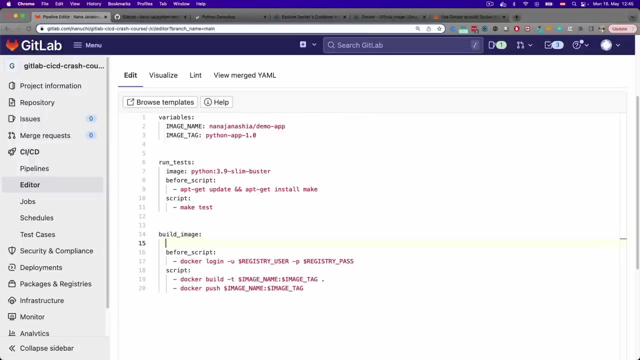 commands or Docker client and daemon available inside your container in order to execute Docker commands. So that's what GitLab CICD official documentation also references. whenever you have this kind of use case- and the configuration is actually pretty simple- The first thing we need to do is obviously set the image to this Docker image and we 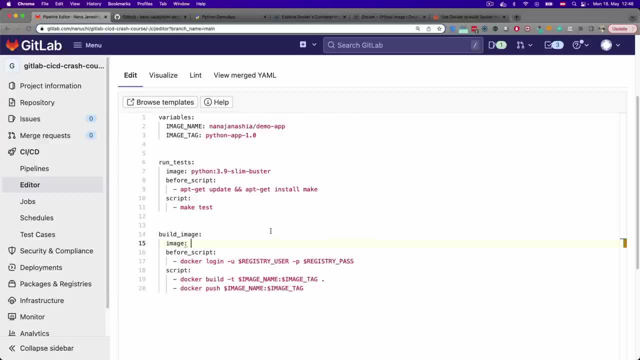 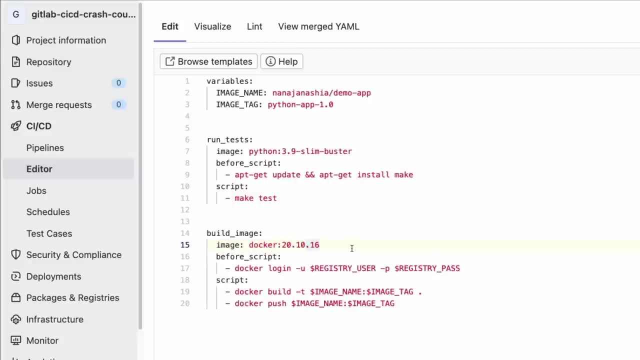 can actually take one of the latest tags. So right here we're going to do Docker and the image tag. So this will take care of starting a Docker container from Docker image. So we have the Docker client available inside. However, we also need Docker daemon available inside. 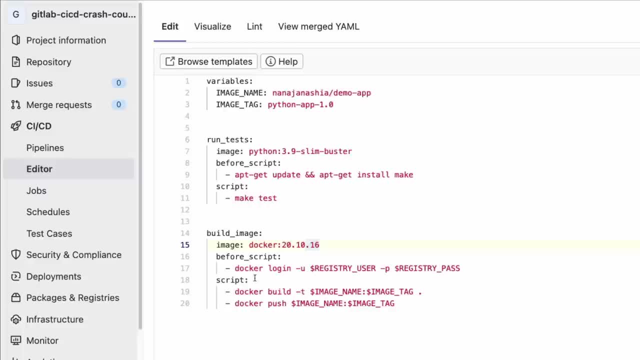 Right. So Docker daemon is the process that lets the client actually execute those commands: connect to the Docker registry, pull the image, push the image, etc. So in order to make that available, we actually need to configure another attribute which is called services on GitLab. 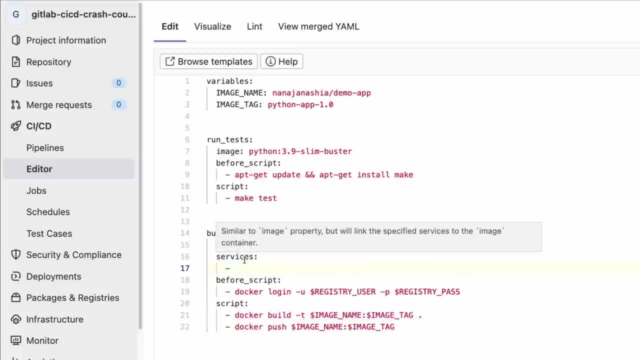 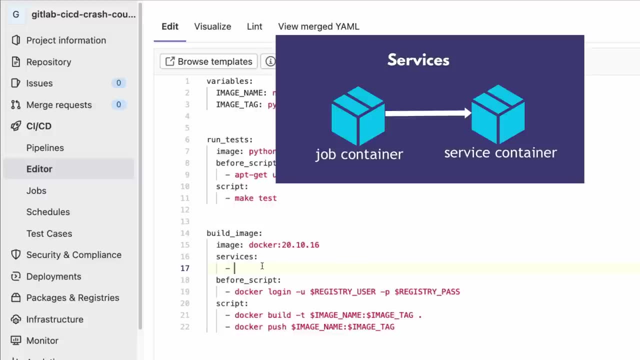 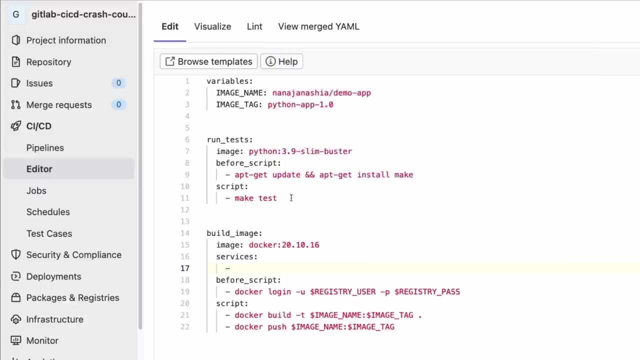 So let's actually define that And I'm going to explain what that means. So service is basically an additional container That will start at the same time as the job container and the job container can use that service during the build time. So, for example, if your test execution needs some kind of service, 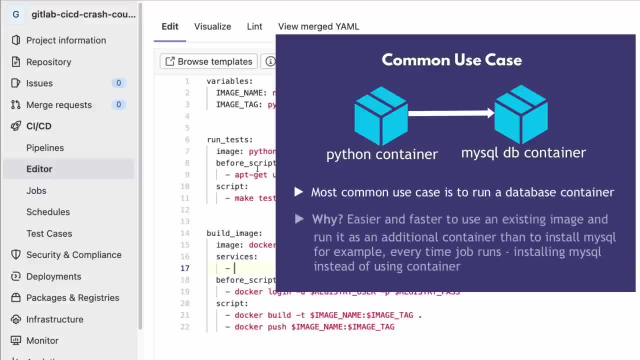 like a database service, for example MySQL, then you can actually start a MySQL service or MySQL container during your job execution. In addition to this, Python container and the service attribute will make sure that these containers are linked together so they run in the same network and they 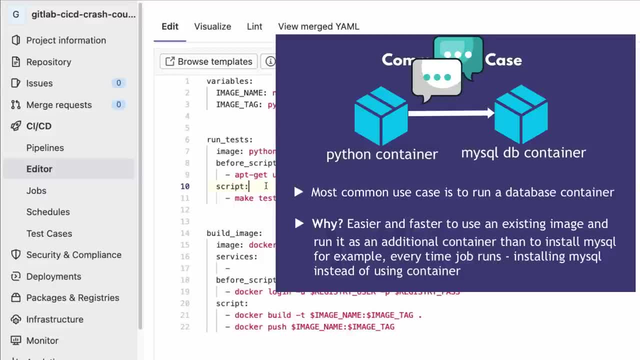 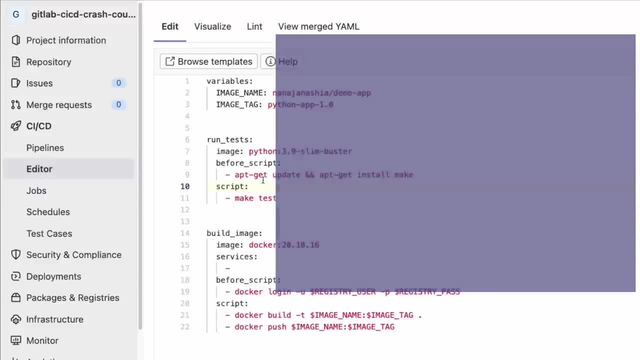 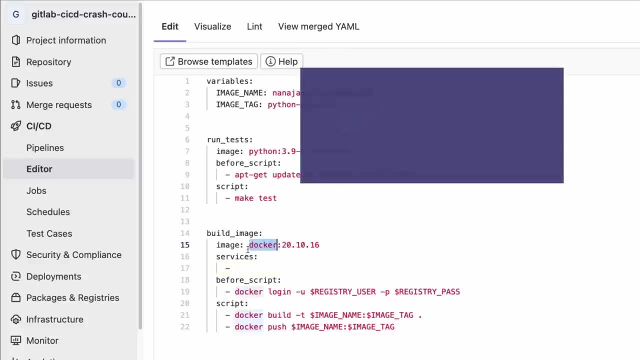 can talk to each other directly. So this way, Python container will actually have access and can use the MySQL service from the other container. So that's basically what the concept of services means in GitLab CICD. So, right here, what we're doing is we have this Docker container with Docker client. 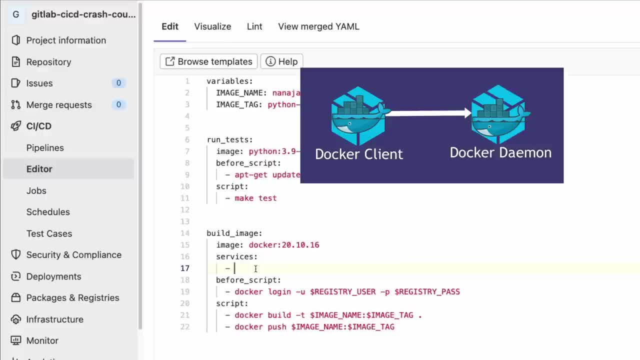 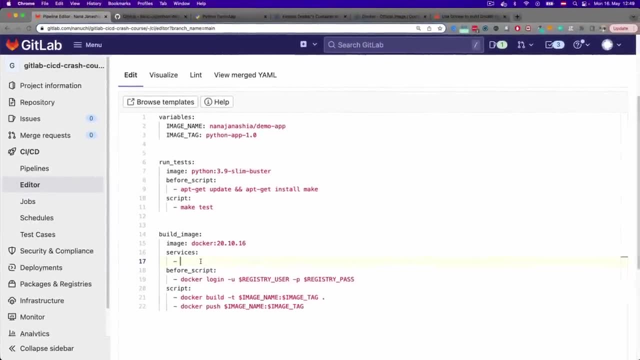 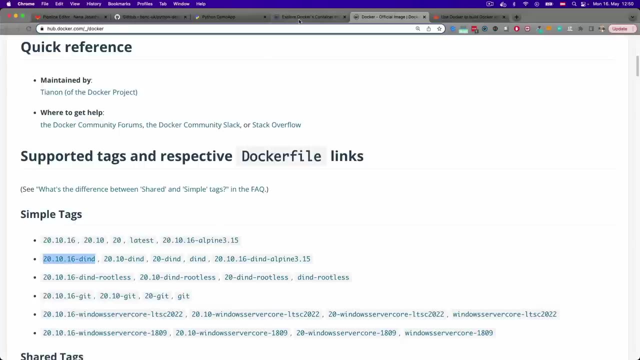 inside and we want to start another Docker container with Docker daemon inside So the client can actually connect to that daemon, the Docker server, and then execute these commands, And then image for the Docker daemon is actually this tag right here, So that's going to be Docker. 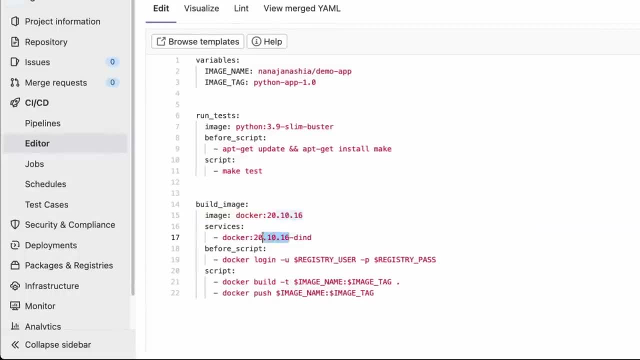 and the same version. So that's the client, That's the daemon, with D I and D, which is Docker in Docker. So these two will basically give us the complete set of Docker client and server in the same job execution environment. So these two containers will be linked. 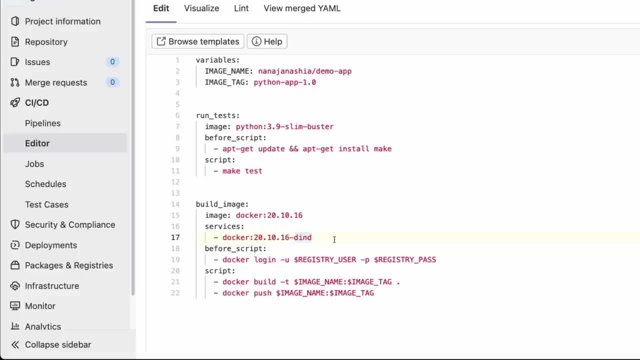 to each other and they will be able to communicate with each other. There is one final thing we need to do here, which is to make sure these two can communicate with each other using the Docker certificates. So these two need to have the same certificate so that can authenticate with each other and talk to each other. 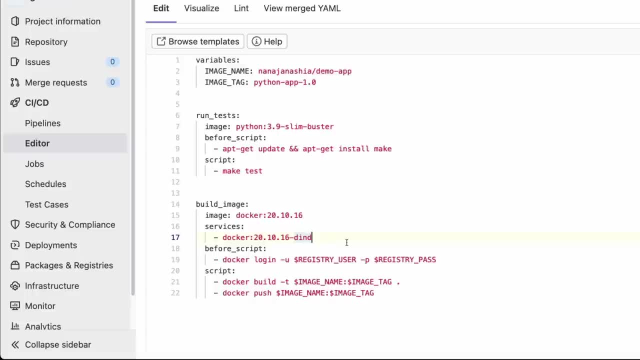 And for that we want those two containers to start to share that certificates directory so they can read from the same certificates folder. and we can do that by defining a variable or environment variable called Docker TLS cert dear and setting that to slash certs. So what this will do again is this will: 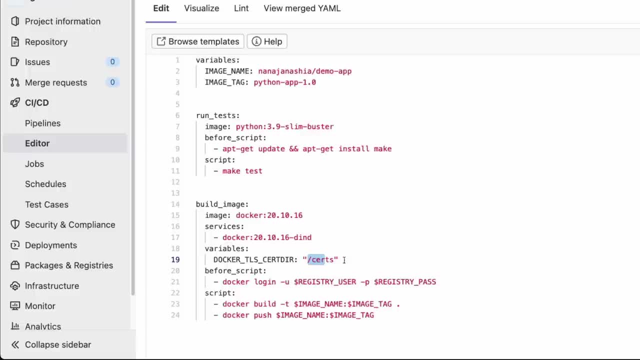 tell Docker to create the certificates in this location And then this certificate will be shared between the service container and the job container. So in this configuration we have a full Docker set up of client and a server or Docker demon, and they can talk to each other. 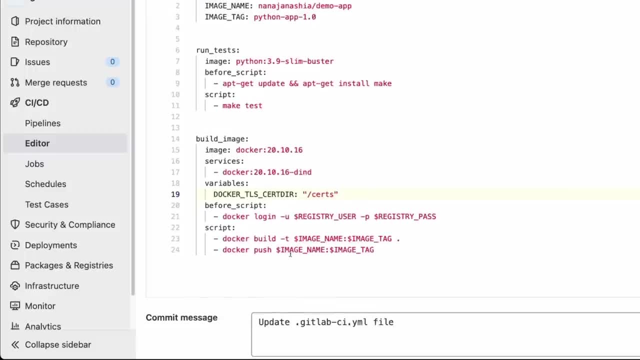 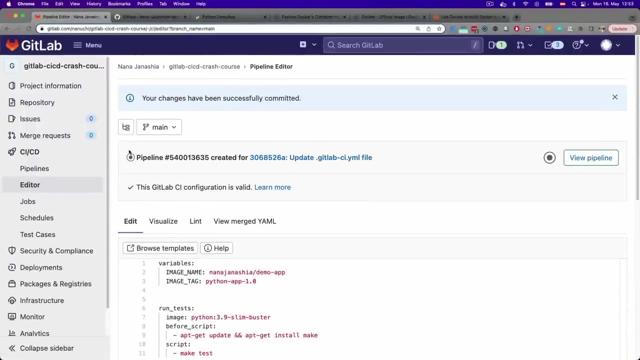 authenticate with each other and so on, And this way we're going to have Docker commands available inside our job. Great. so now let's actually commit our changes and GitLab will automatically trigger a pipeline for us, And you see that pipeline execution here. 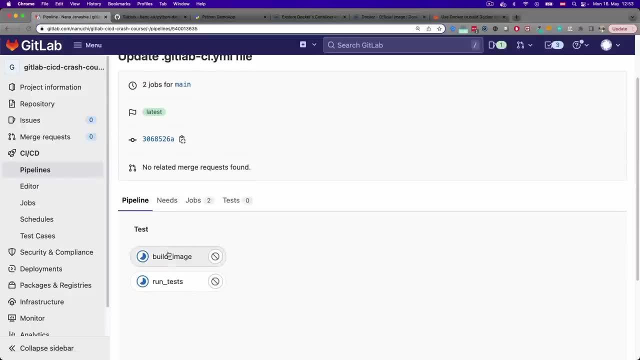 if I do view pipeline now, you see that two jobs are being executed inside the pipeline, both running at the same time. So let's wait for them to finish. And there you go. Both jobs were successful, which means we should actually already. 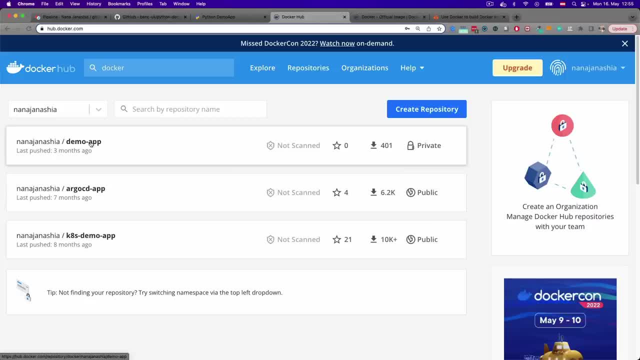 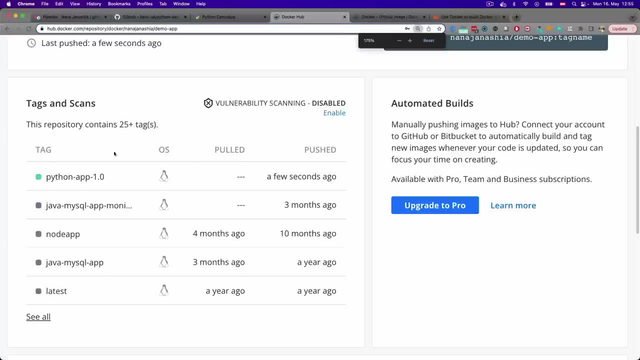 see an image in our Docker Hub registry, So I'm going to go to my repository and right here, pushed a few seconds ago, we have Python app, One point zero. So we have successfully built and pushed a Docker image to Docker registry using 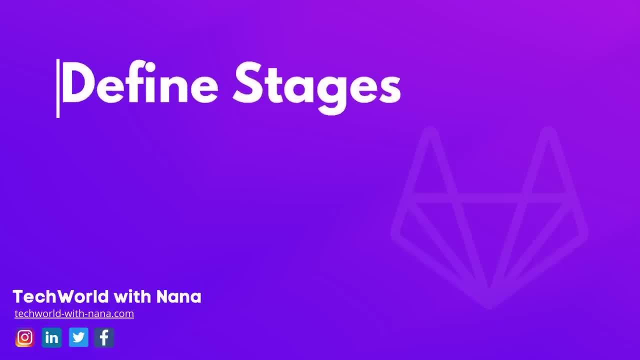 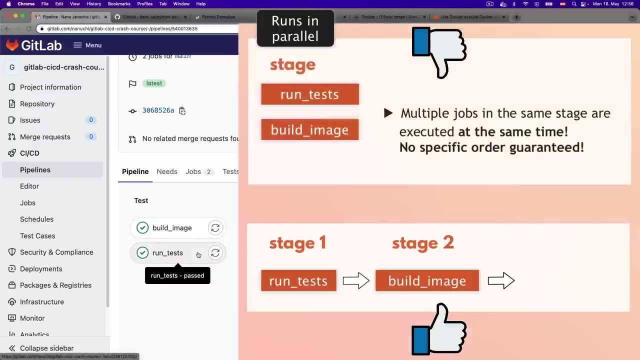 GitLab, CI city pipeline. However, there is one issue here, which is that both jobs get executed at the same time, And if we add deploy job, it will also run in parallel to these two jobs, And this makes no sense for us, because we want to. 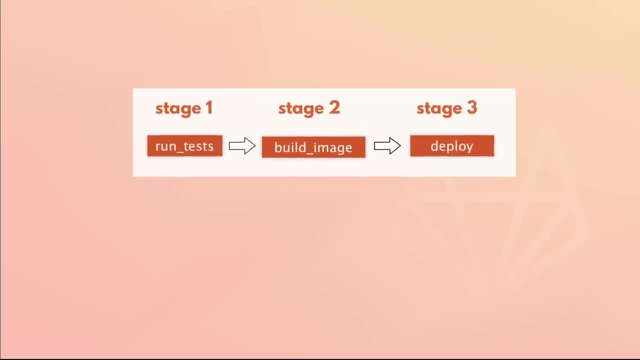 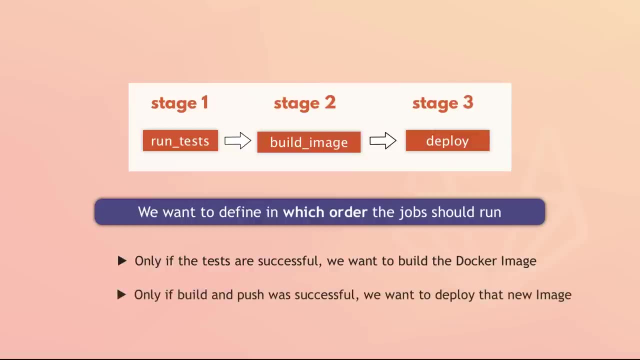 Run these jobs in order right. So we want to run the tests, and only if the tests are successful we want to build and push the image, and only if build and push job was successful Then we want to deploy that image, because if build fails we have nothing to deploy. 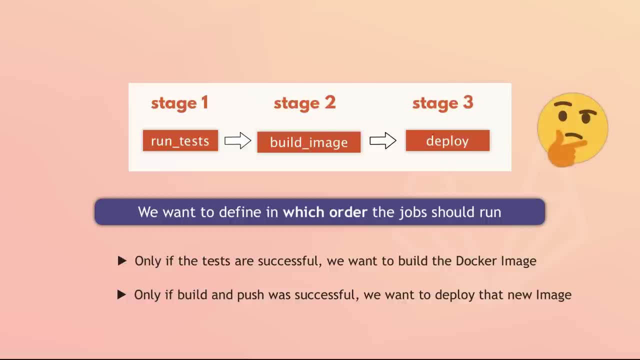 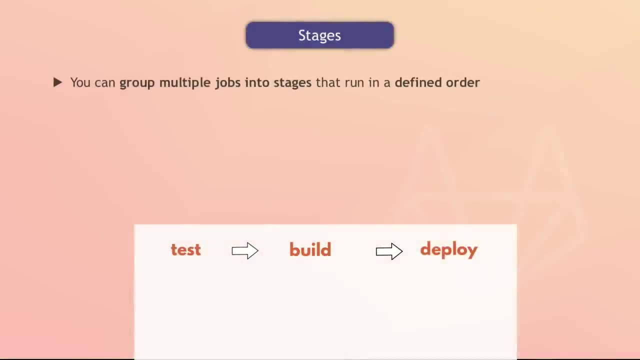 Right. So how can we force this order in which the jobs will execute in the pipeline? Well, we can do that using what's called stages. So the stages can be used to organize the pipeline by grouping related jobs that can run in parallel together. 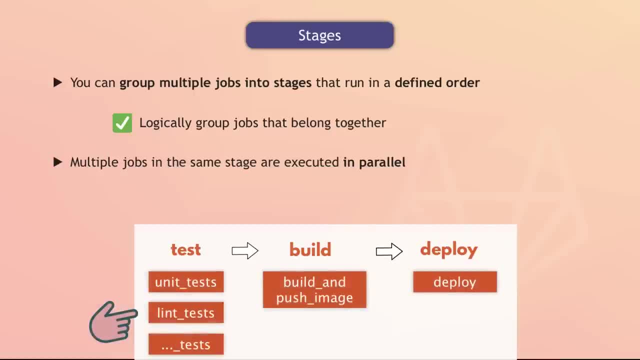 So, for example, if you have different tests that you run for your applications, like unit tests, linked tests, whatever- they can all run in parallel by being in the same stage. So let's see how that works. Going back to the editor, 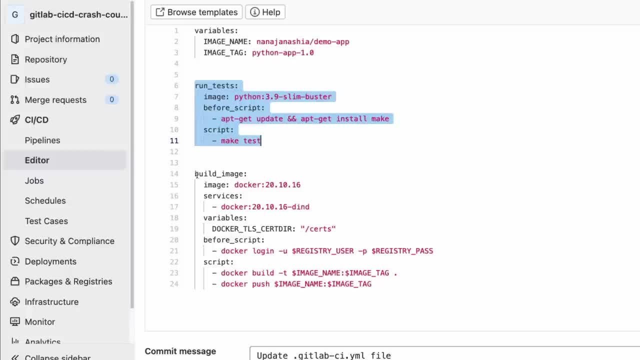 We want to put the run tests in one stage and then have built the image as the next stage. So build image will basically wait for the run test to execute And only if the run test was successful it will execute the build image job. 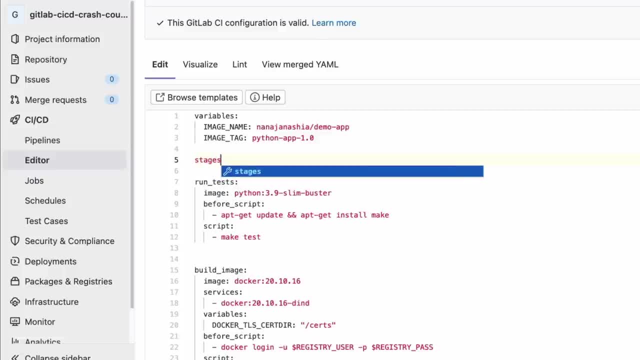 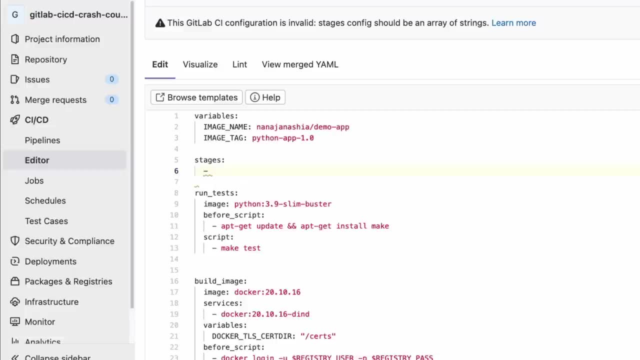 And it's super easy. We have the stages attribute where we can create a list of stages and we can call them whatever we want. I'm going to create test stage and build stage And then, from those stages that you have defined here, you can. 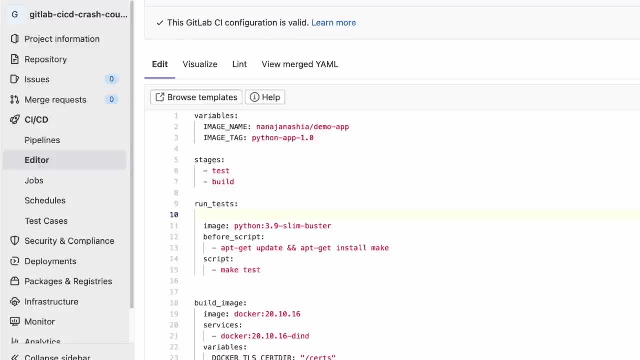 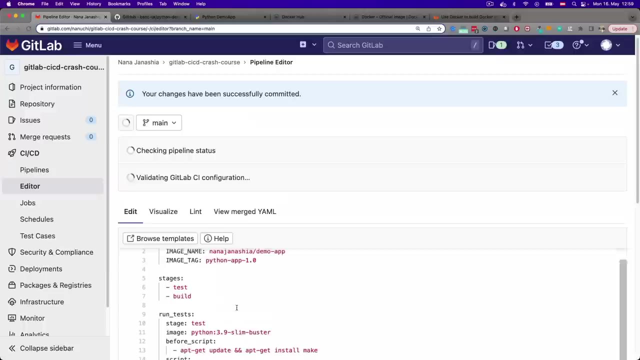 reference them within your jobs. So right here we can say: run tests in test stage and build image in build stage. That's it. That's the whole configuration. So I'm going to commit that And let's see the result. So the pipeline got triggered. 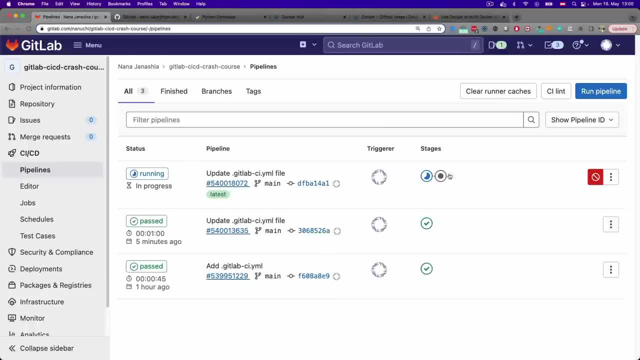 If I go to pipelines, The first difference right away that you see here is we have two stages now, So we have test stage and build stage, Whereas here by default, we don't specify any stages. GitLab gives you a test stage. 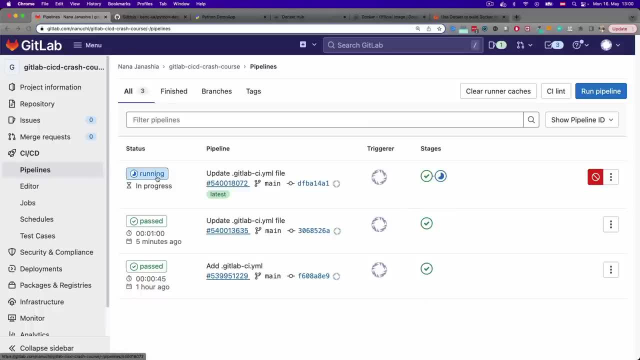 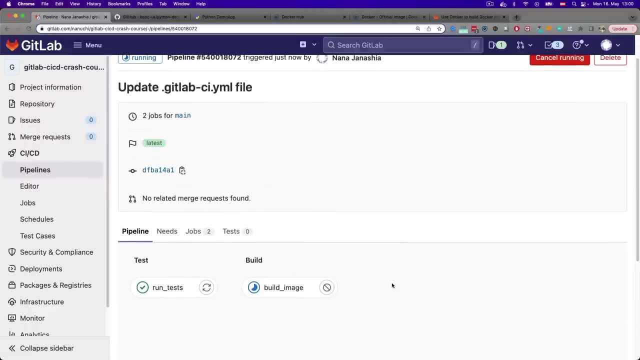 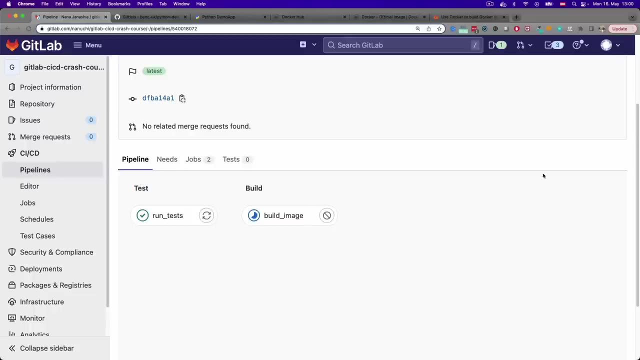 So everything gets executed in that test stage And if we go in the detail view of the pipeline, you also see a visualization of those stages. So instead of the jobs being just listed here within one stage, you now have the stages listed next to each other. 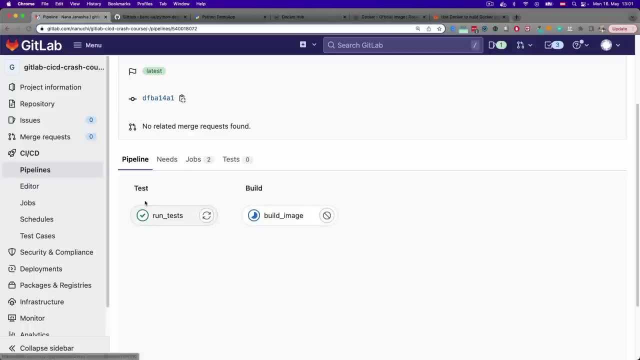 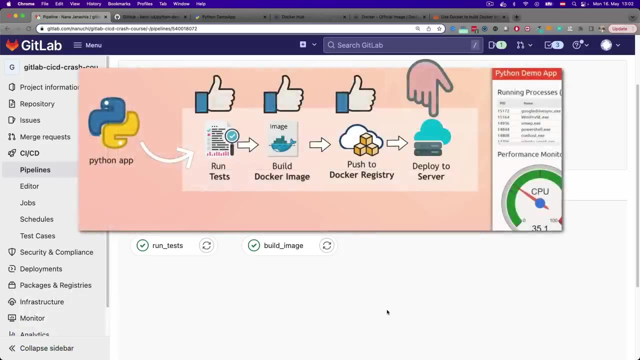 And the jobs in the build stage will wait for any jobs in the test stage to complete before they run. So that's how the stages looks like, And when we add more stages they will basically just appear next to each other. So these two steps are configured. 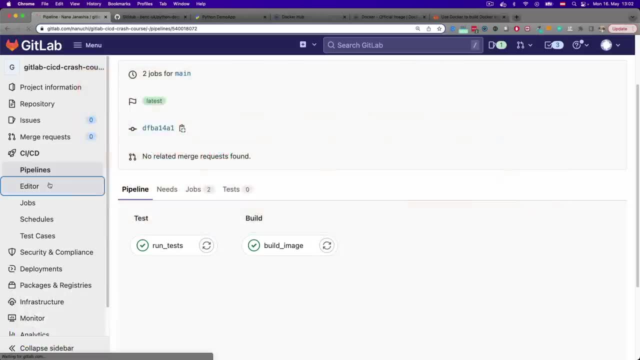 Now let's add the final job to our pipeline: to deploy that newly built Docker image to an Ubuntu server and run that Docker application there. For that we first need a deployment server right. We need a server that we're going to deploy to and run our application. 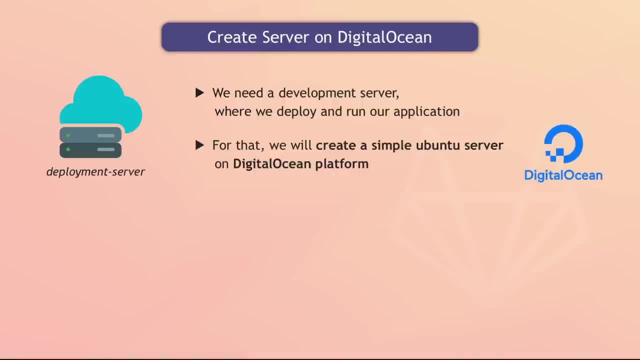 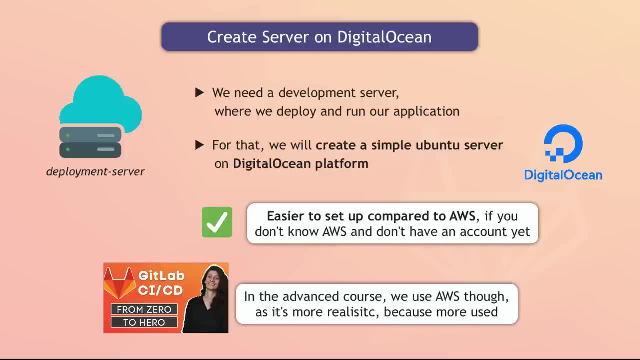 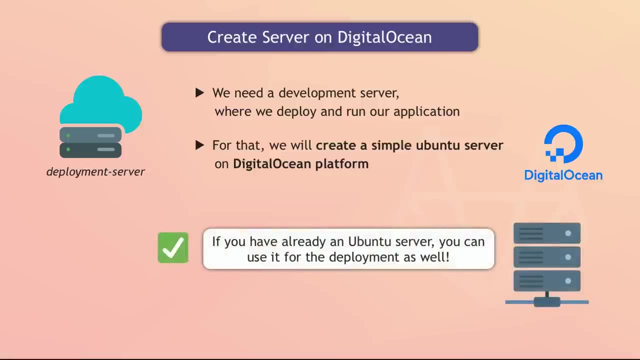 To make this easy, we will create a simple Ubuntu server on a DigitalOcean platform. It's way easier to set up and configure than AWS if you don't have an AWS account. So that's the platform we're going to use. Now, if you have an Ubuntu server or other server, you're welcome to use that as well. 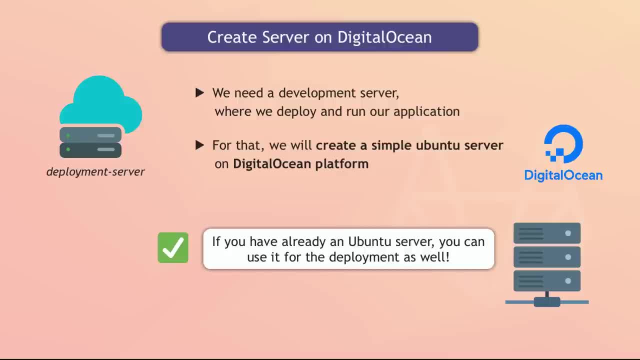 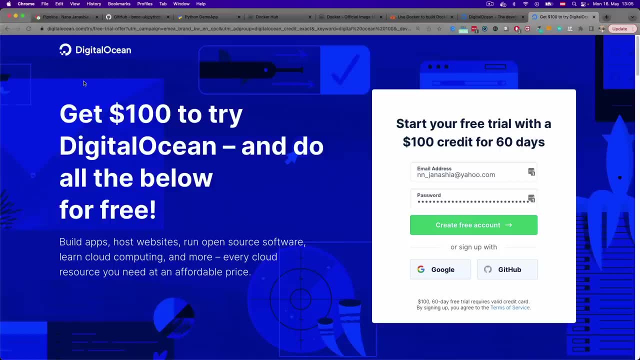 So this is not specific to any cloud platform. We just need an Ubuntu server that is connected to Internet that we can deploy to And on DigitalOcean. actually, you can sign up a new account with $100 credit, So make sure to take advantage of that if 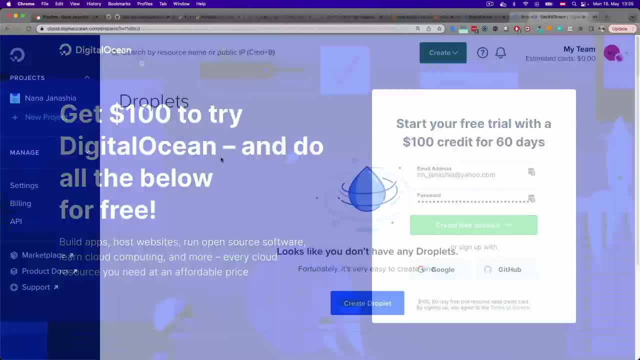 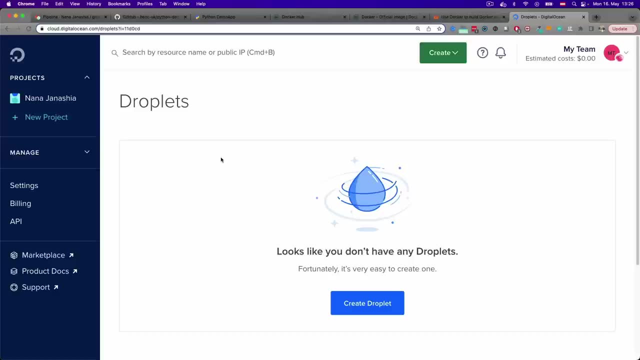 you register here so that you can work through the demo for free. I already have an account, so I'm going to look in And I'm starting with a completely clear state. I don't have anything configured yet, So we're going to do all this together. 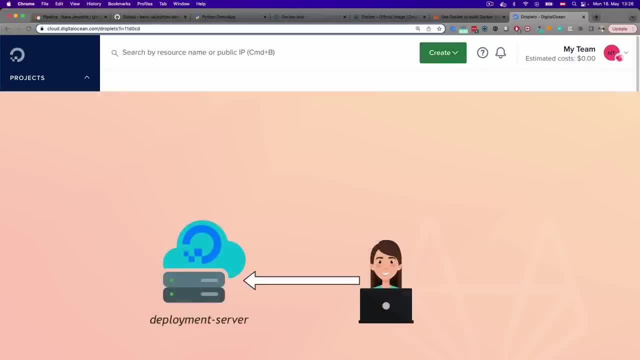 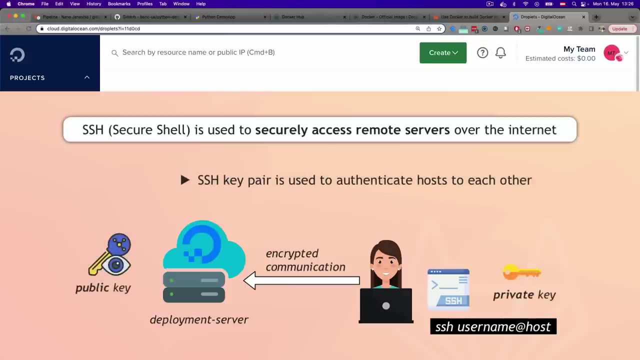 First of all, when we create the server, we will access that remote server on DigitalOcean from our local machine using an SSH command, And to SSH into a server obviously we need an SSH key And on DigitalOcean we can add our own SSH key in the settings here. 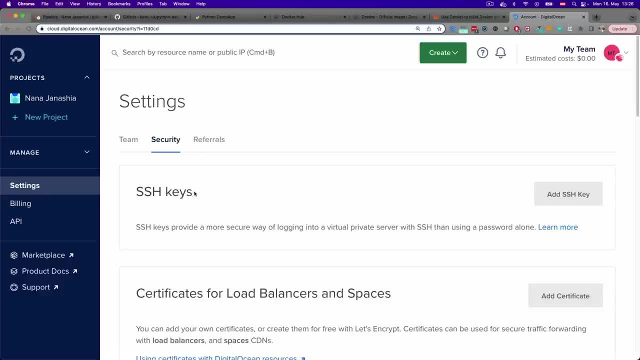 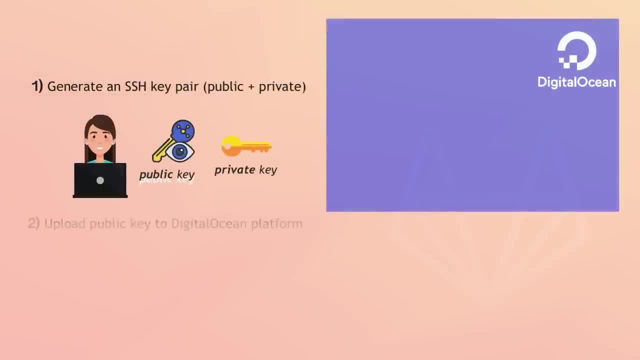 So in settings, security, you have a section here that says SSH keys and you can add one right So you can generate an SSH key here. you can upload the public key of that key here to DigitalOcean And then all the servers that you create. 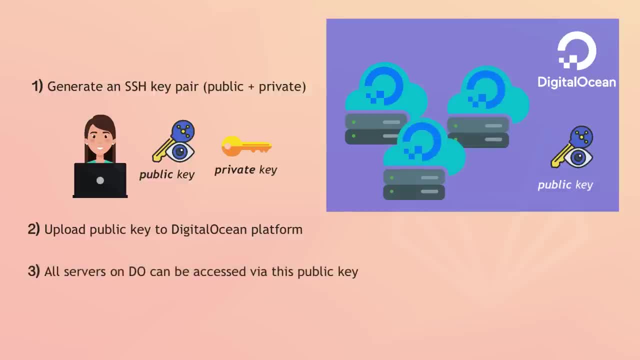 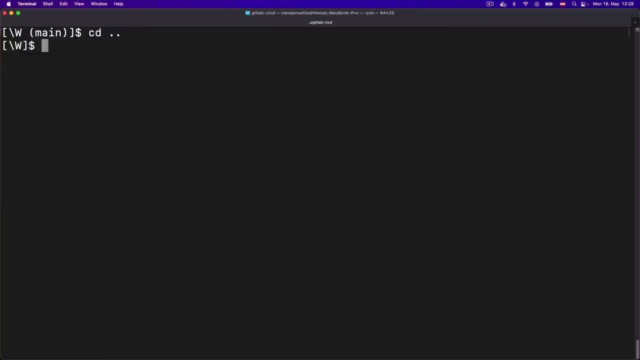 on DigitalOcean will be accessible using the public key that you uploaded here. So that's how it's going to work. So what we're going to do is actually create a new SSH key locally, which is very simple. I'm going to leave the project and right here I'm going to execute a simple 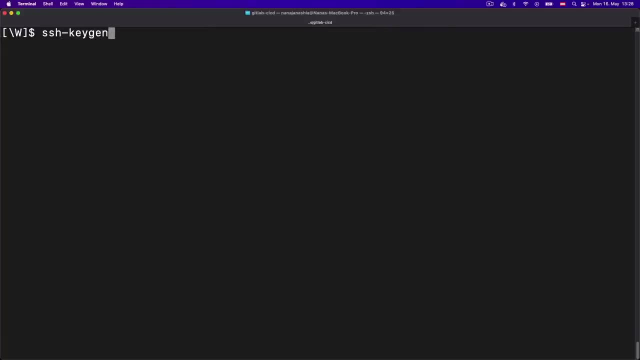 SSH key gen command And this will basically generate an SSH key pair for us. So enter, And this is the default location where your SSH keys are, And this is the default key pair that is always used when you SSH. So we're going to. 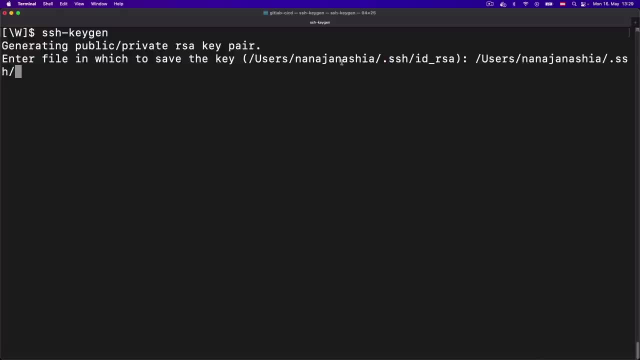 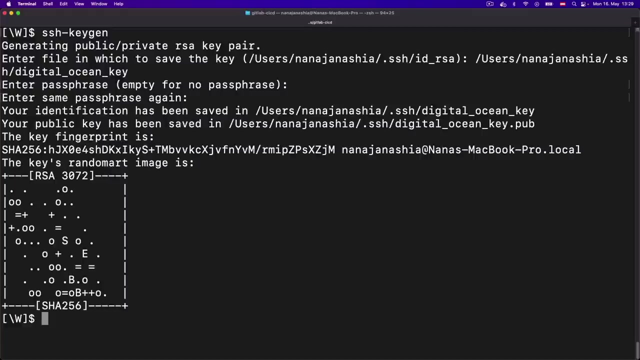 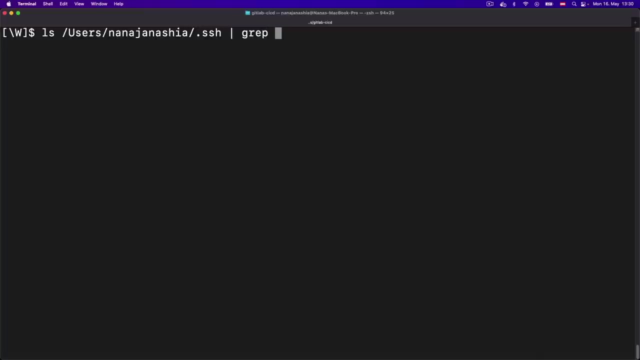 use a different name inside the ssh folder in your users directory And let's call this DigitalOceanKey. We're going to leave the passphrase empty, Repeat And there you go. That was it. And now inside that SSH folder, we should actually see our DigitalOcean key pair. 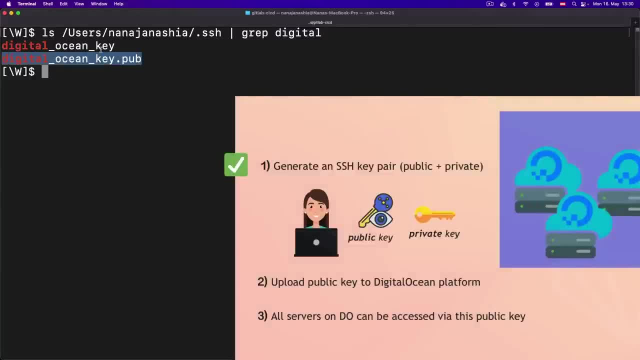 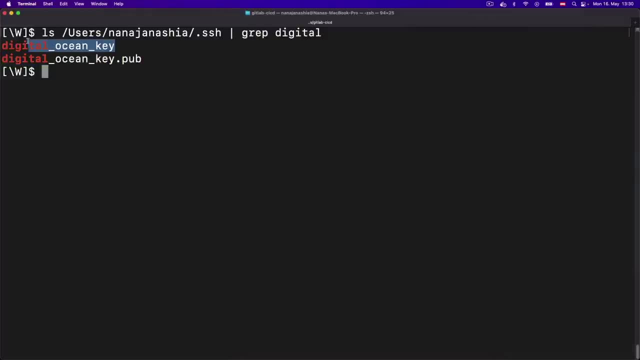 So we should have two keys: One of them is public and this is the private one. So that's the one we need to upload to the platform, And then we're going to be able to connect to any server created on the platform and using the private key. 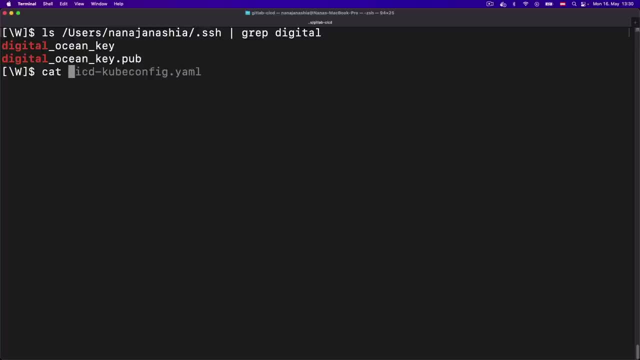 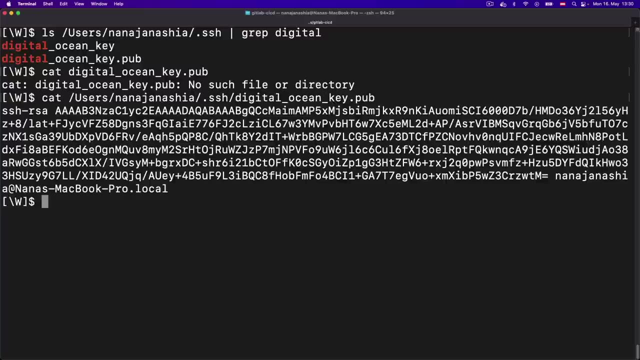 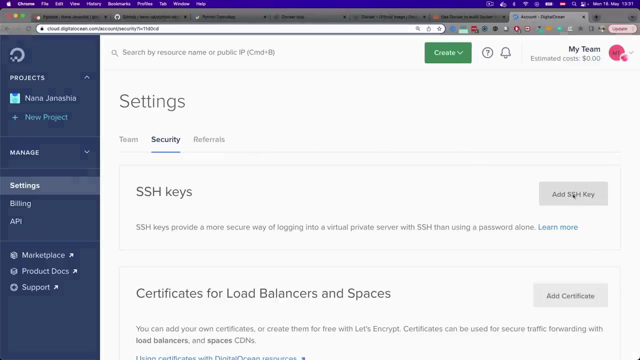 And to upload that. we're simply going to cap this And obviously I need the whole path Like this And that's our public key. So I'm going to copy that to new SSH key. copy the contents. Let's give it a name. 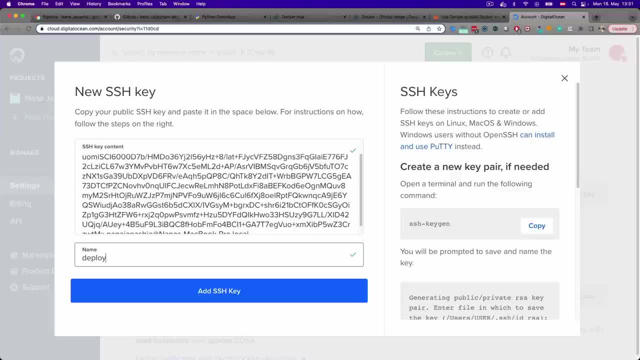 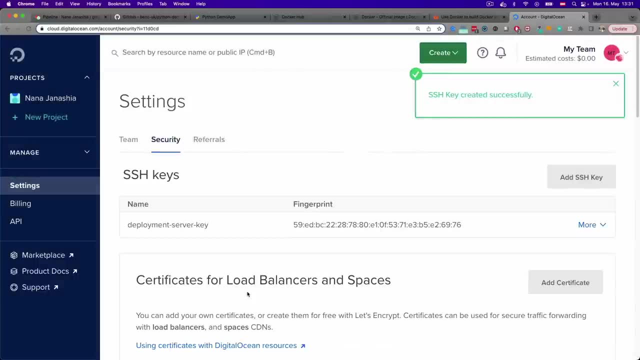 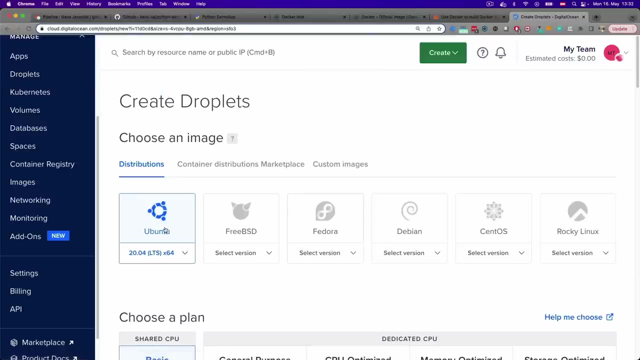 Let's call it a server or deployment server Key and add SSH key And that's it. So now I'm going to go back to the droplets and create a deployment server. So click on create droplet. I'm going to choose Ubuntu with the latest version. 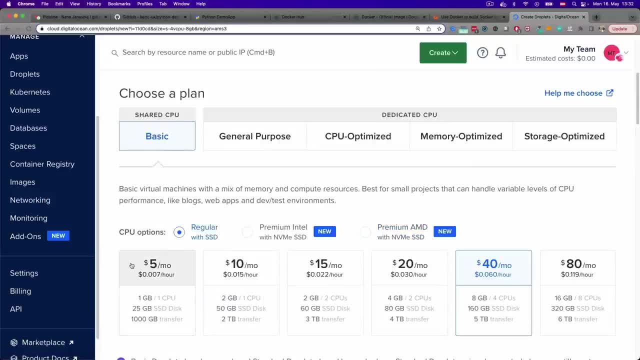 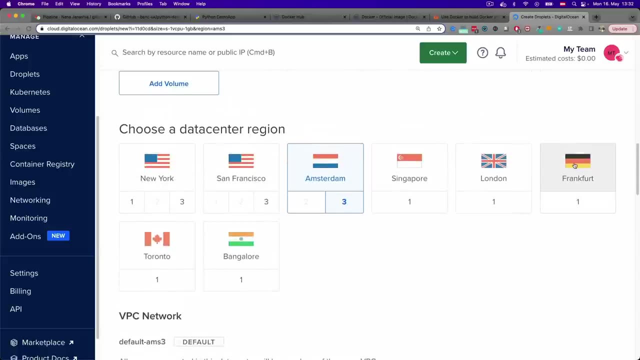 Basic plan, regular with SSD, And I'm going to select the smallest server with the smallest resources, because we're just going to be deploying one application container, which is our Python app, So we don't need much resources. And, finally, we're going to choose the region which is closest to our location. 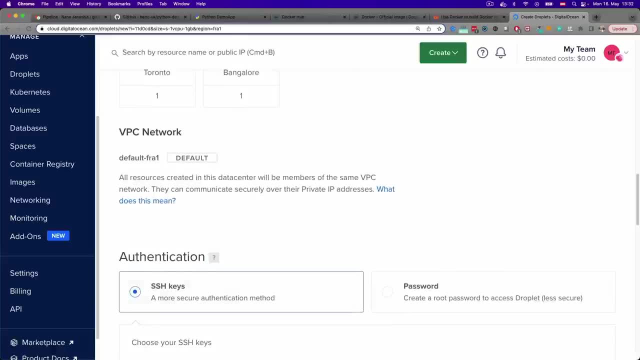 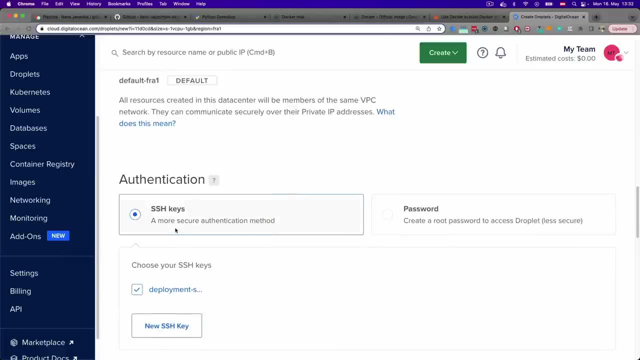 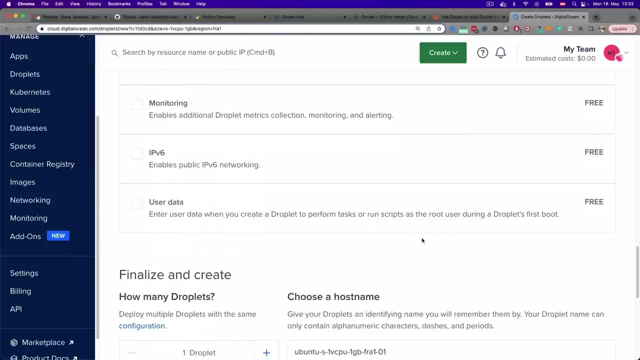 And that's it. All the other stuff will stay the same. right here in the authentication You already see that SSH keys is selected. So that's going to be how we connect to the server And that's the key that we added. So we'll leave everything else. 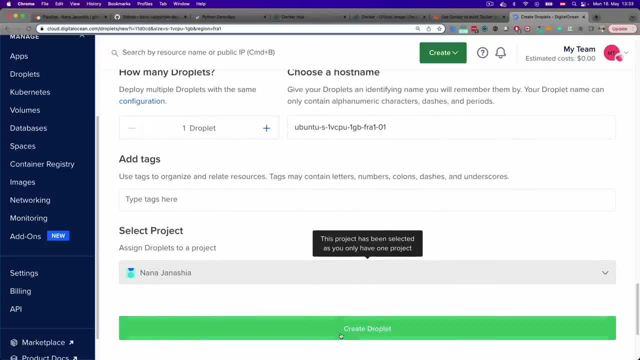 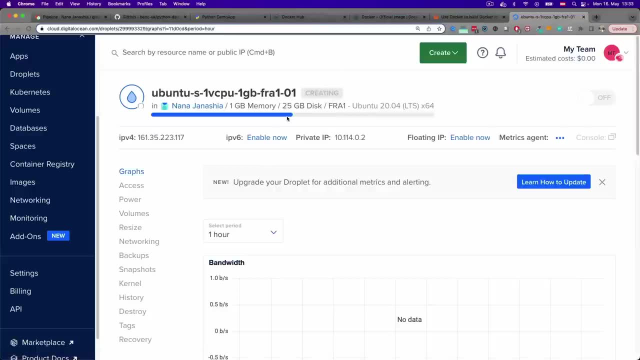 With defaults. we are creating one droplet and create And let's wait for our droplet to be fully initialized. There you go, And once it is initialized, we're going to need to configure one thing on that server before we're able to deploy and run our Docker image to that server. 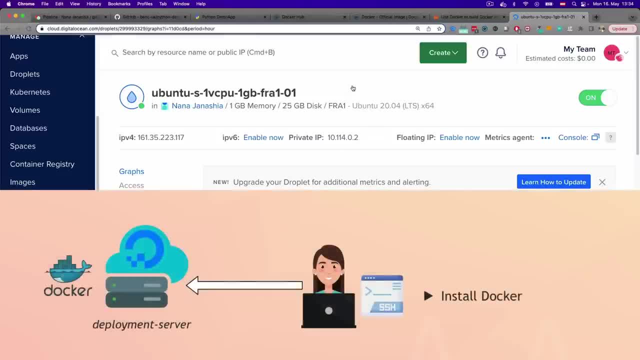 which is, we need to install Docker because we're going to be running Docker container on it. So we need Docker available And for that we're going to grab the public IP address of our droplet, of our server, which is this one right here. 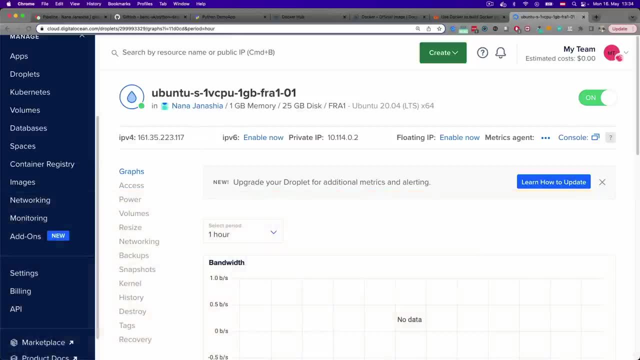 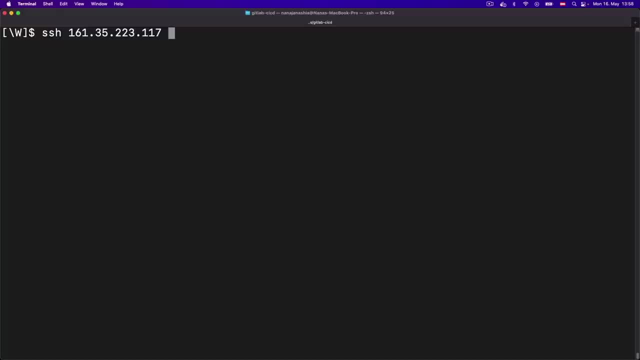 Let's copy and we're going to connect to that machine locally And we're going to SSH into the server using an SSH command and the IP address of the server, which is a public IP address. But of course, when we SSH into a remote server, we need to authenticate ourselves. 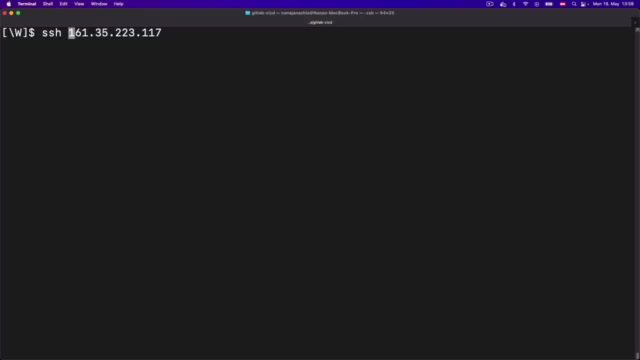 Right. We need to provide credentials- in our case username, or Linux username, and private key. So the Linux user on droplet servers is root. So that's the user we're connecting with, And here we're going to specify the private key that we want, the SSH command. 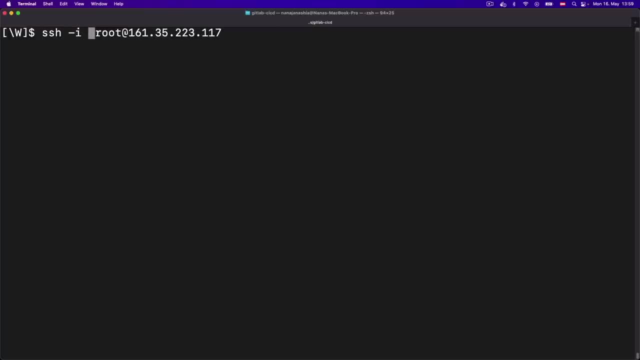 to use to connect to the server using this I option. and we need the location, So that's the home directory of my user, Dot, SSH and Digital Ocean Key. So with this command we should now be able to connect to the server. 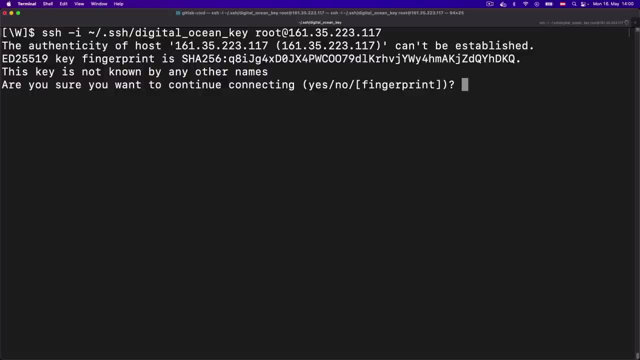 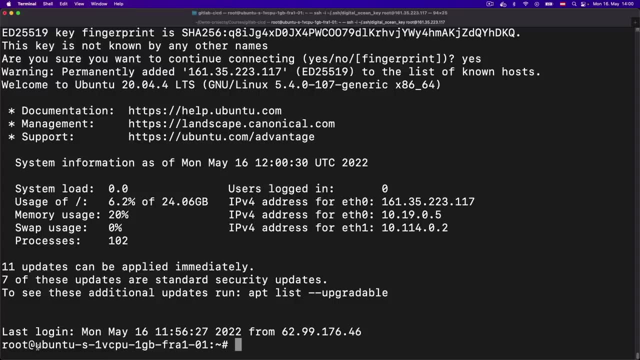 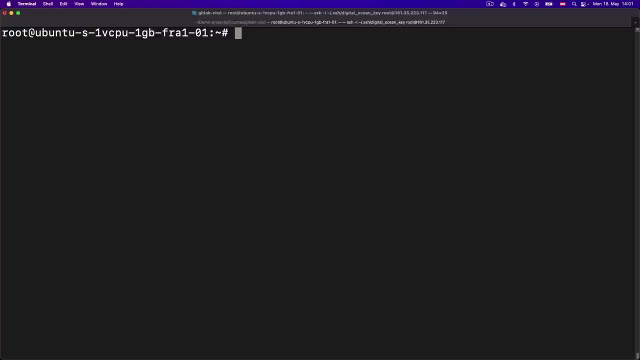 So let's execute- And this is a confirmation- to save that remote server locally as a known host. So let's confirm, And there you go. We are inside our droplet, connected as a root user And, as I said, we need to install Docker on this machine. 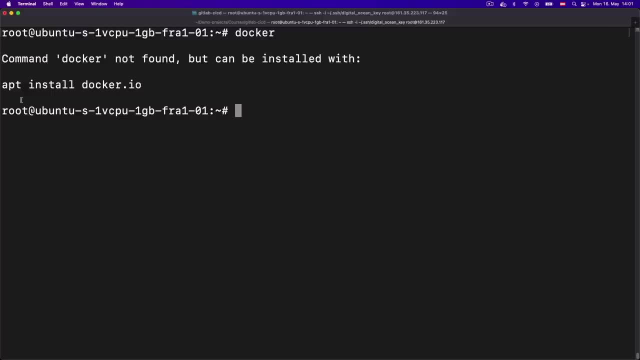 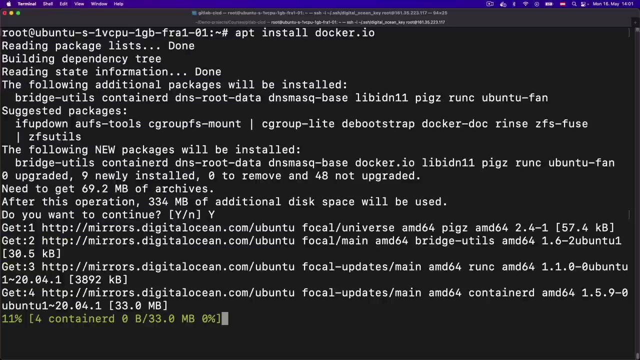 So if I do Docker- obviously right now it's not available and I'm going to use this suggested command to install Docker. But before that we're going to do Ept update And now we can do Ept install Docker. There you go. 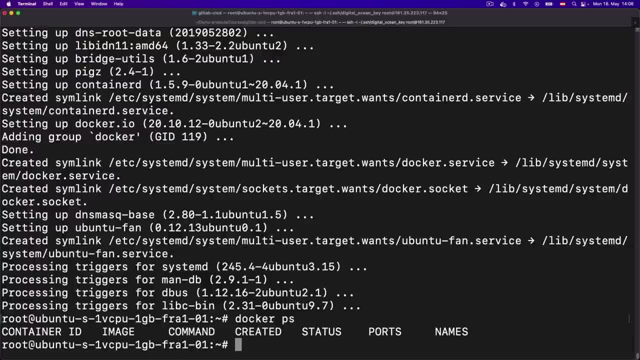 And now we should have Docker commands available. Let's do Docker PS to check. And there you go. Currently nothing is running, but we're going to deploy to the server from our pipeline so we can exit from the server. Our work is done here. 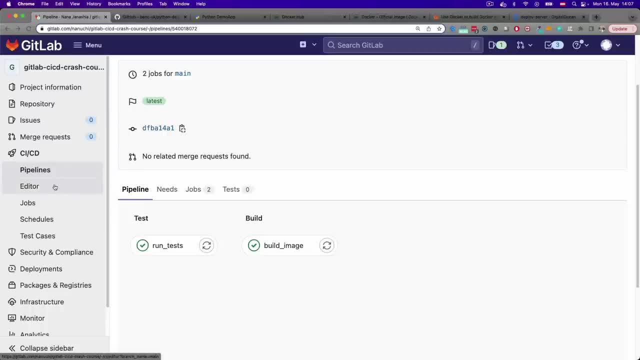 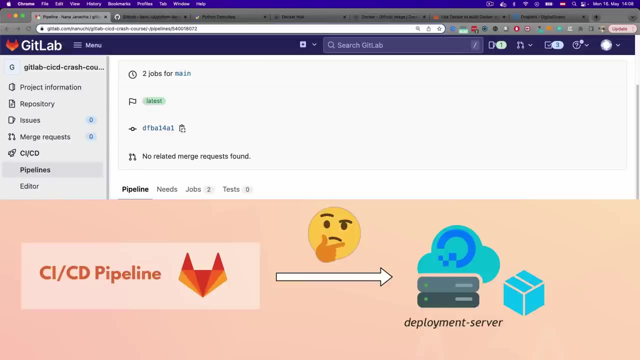 And we're going to go back to our pipeline configuration and add a third job that will deploy to that server. So how is GitLab going to deploy a Docker image to the droplet server or how is it going to connect to the server in order to deploy the Docker image? 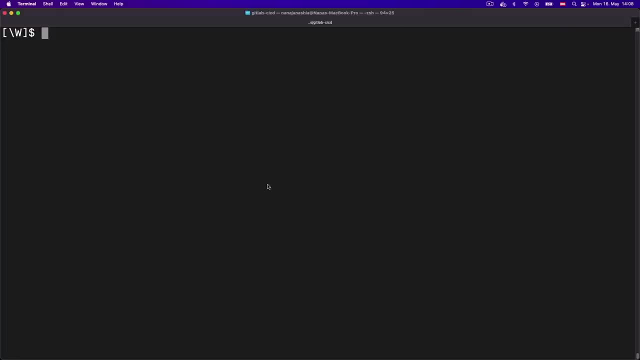 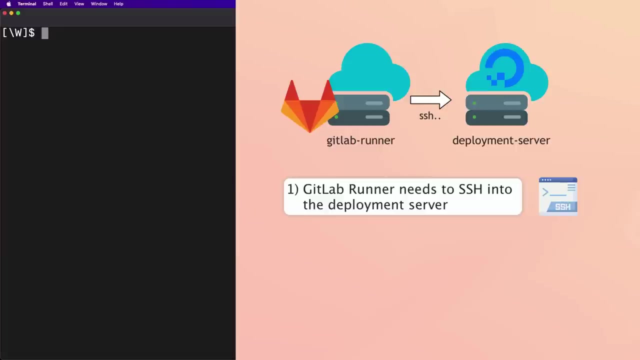 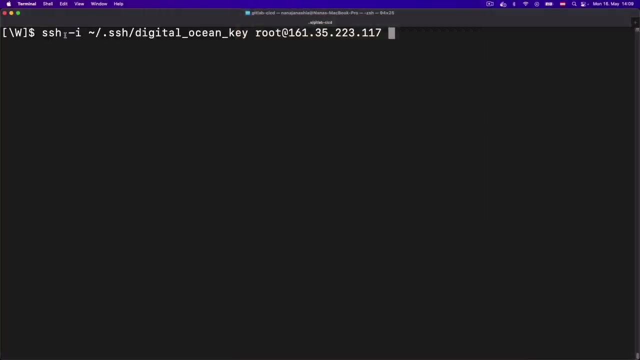 Well, actually the same way as we did locally using SSH command. So again, GitLab runner will start a container for the deploy job and inside the container we're going to execute SSH command to connect to the remote server. And for that SSH command we're going to need exactly the same information, right? 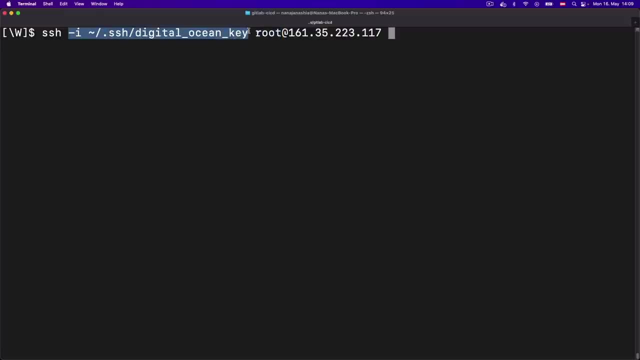 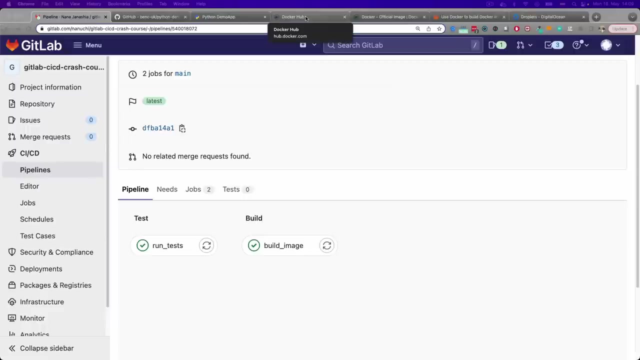 So we're going to have the root user and we're going to need that private key to connect to the server, which means we need to make this private key also available to GitLab. And just like we created variables- secret variables- for Docker Hub private repository, we're going to create a secret. 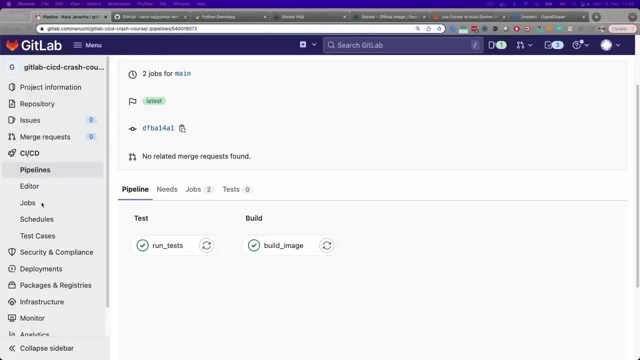 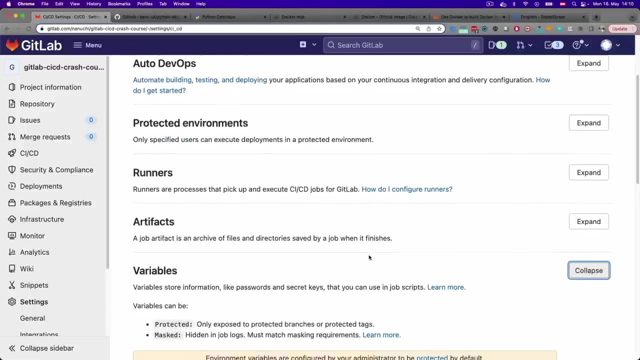 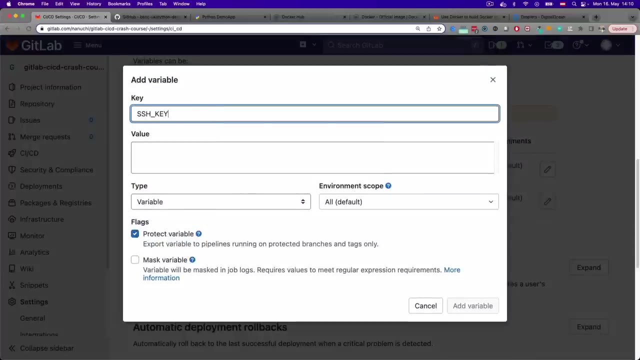 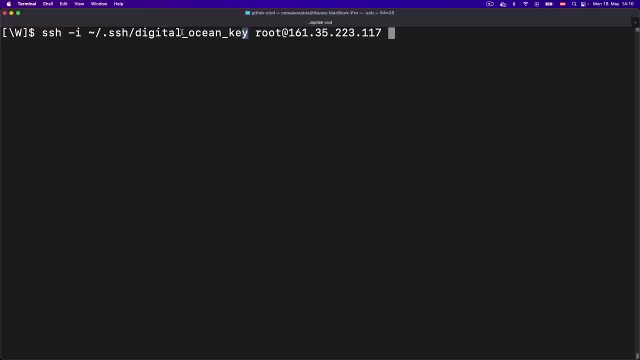 variable for the private key in the CICD settings. So, going to settings, CICD In the variables section, we're going to add a third variable and we're going to call this SSH key And the value of that key will actually be the contents of that key file. 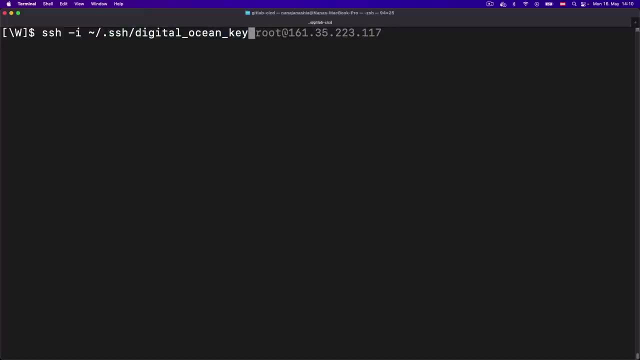 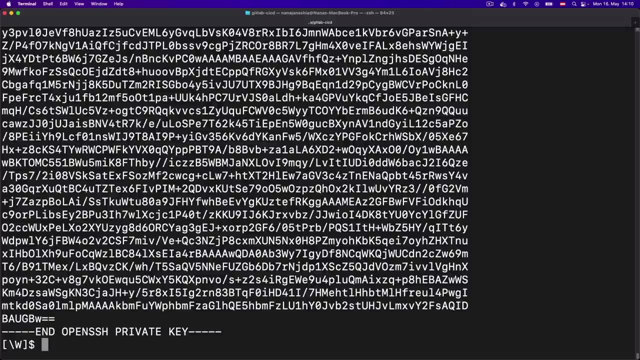 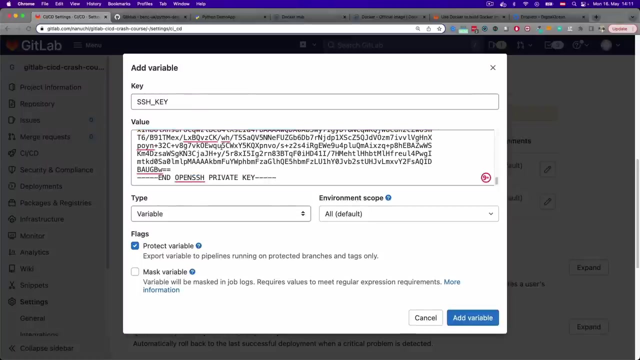 Right, The private key file. So I'm simply going to get that, print that out to the console like this, and copy this whole private key and paste it in here. So these are the file contents of the SSH key And right here in the type field, 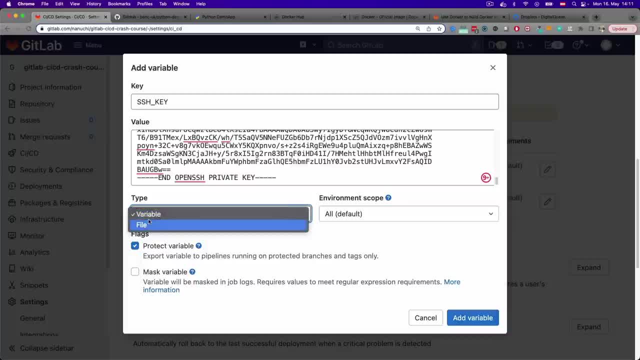 if I click inside this dropdown, you see that we have two options: We have variable, which is a simple text variable, and we have a file. In this case, we actually want to have a file variable because we're going to reference this as an SSH key file. 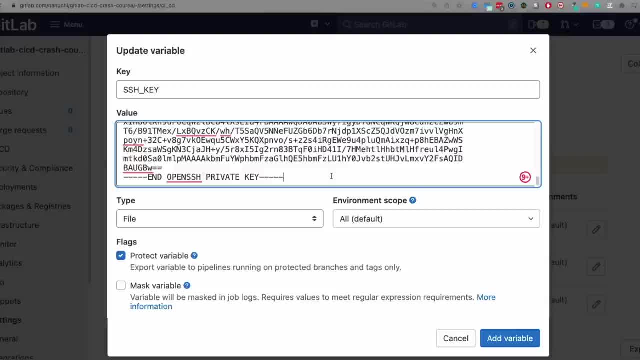 So let's select that one, And there is one kind of a workaround so that GitLab can create a temporary file from these contents with a correct format, And it's kind of a weird workaround To fix the issue. So it could be a bug in GitLab. 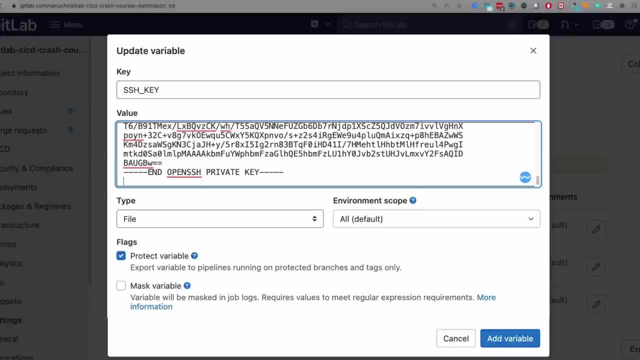 I'm not really sure. So what we're going to do is we're going to add a new line here at the end of the contents so that a correct private key format is created by GitLab. So what GitLab will do in the job execution environment. 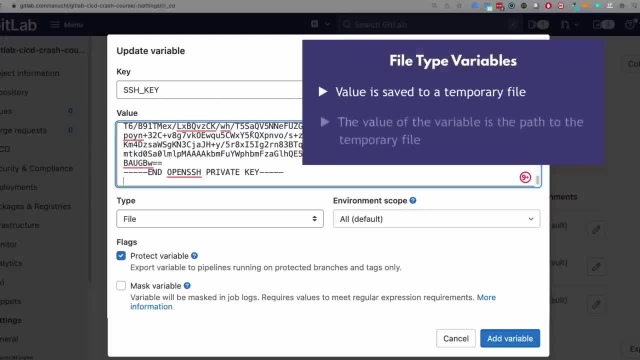 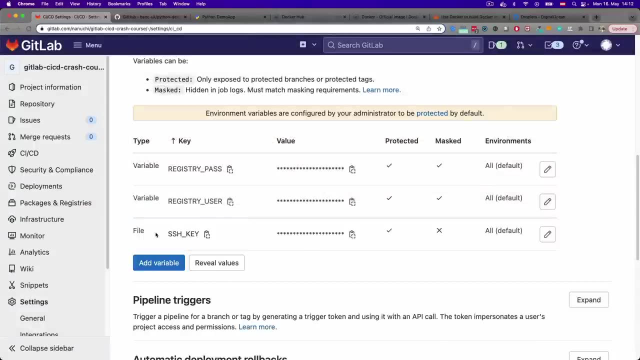 it will take actually these contents of the variable and it will create a temporary file from this, because we have a file type specified. So it will create a temporary file with the contents that we have. here We're going to add the variable. So now this SSH key file will be available inside the pipeline. 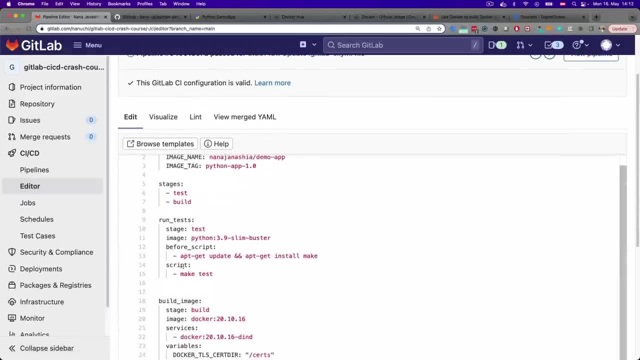 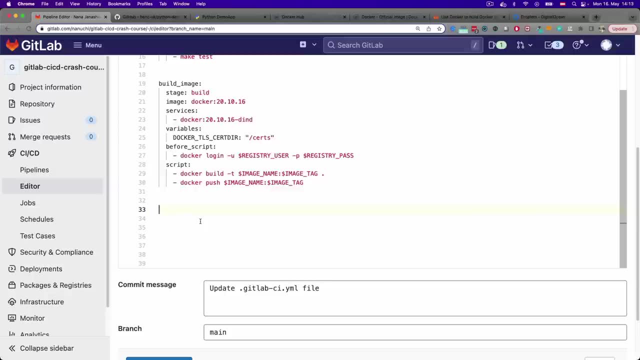 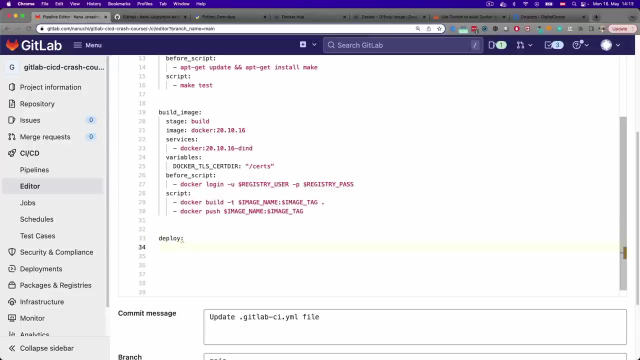 So let's go to editor, And first I'm going to add a new stage here. Let's call this deploy, And here I'm going to create a new job called deploy. You can call it deploy to development. whatever, I'm going to keep it simple. 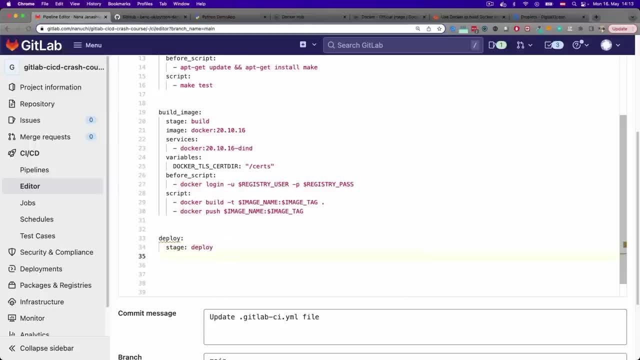 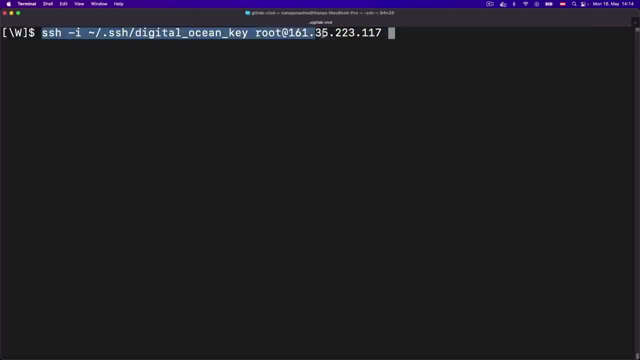 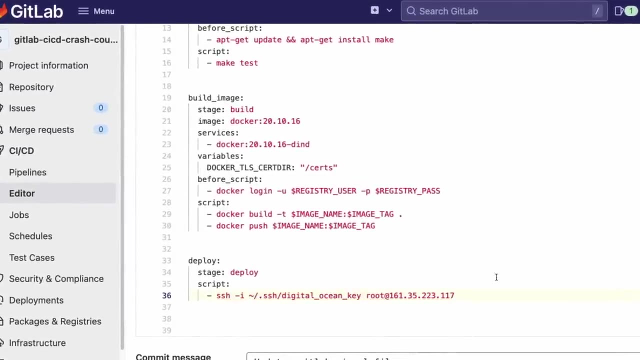 This is going to run in deploy stage And now we have our script and I can actually copy this whole command And modify the respective values here. so that's command we're going to be executing because we want to SSH from the job environment to the remote server. 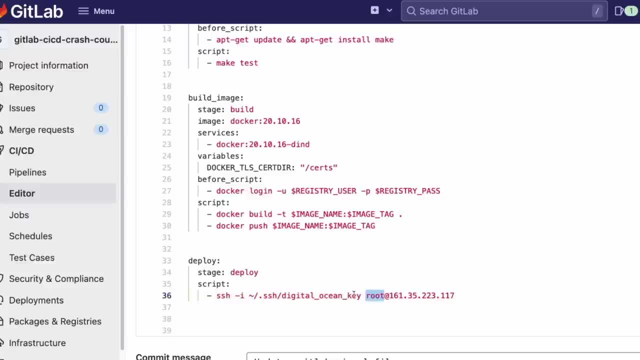 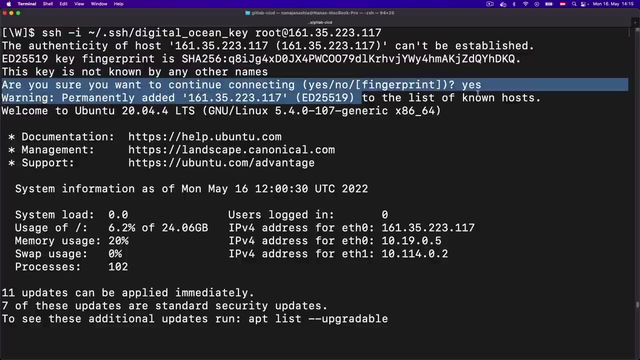 So the public IP address obviously will be the same, the root user, And this is the file that we have as a reference. We're using a variable, So we're going to reference that variable- dollar sign SSH key- And remember this confirmation we had to make here. 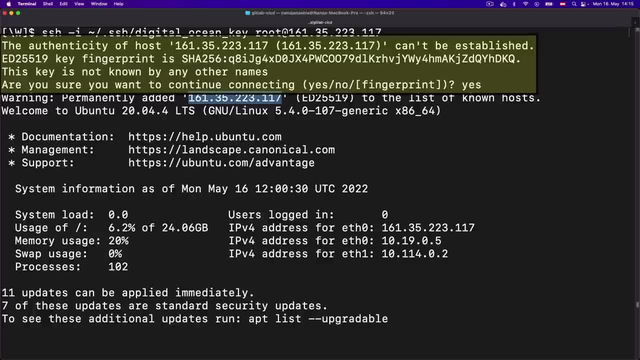 to save that remote server in the list of known hosts, And that's actually an interactive step, So it needs some manual input And if we don't provide a manual input this will not work. So want to actually skip this step because in the pipeline execution 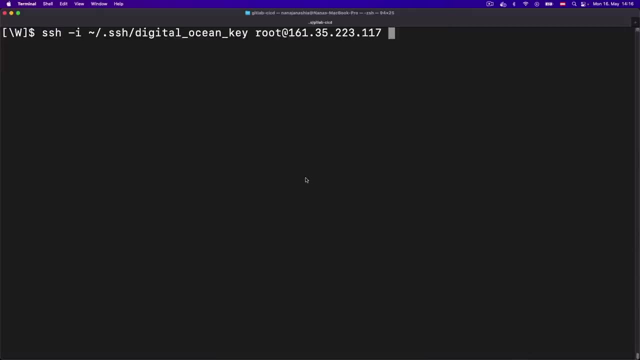 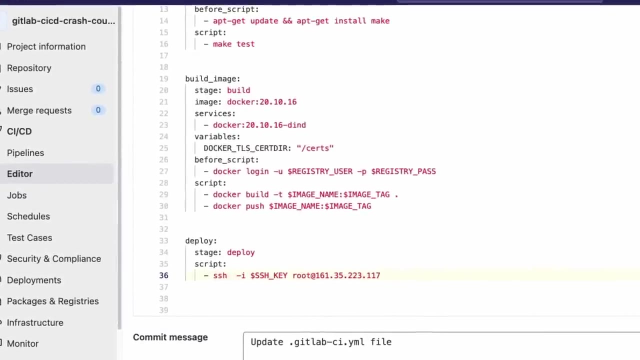 we don't have a manual step, So we want to tell the SSH command. you know what? Forget about that check. just connect to the server and that's it. And for that we're going to add an option here called strict host key checking. 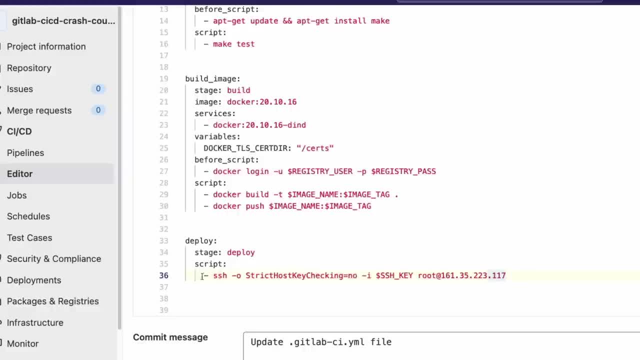 Equals no, so it will skip that. So no manual input will be required here. So that's an SSH command to connect to the server. But once we connect to the server, obviously we need to do something right. We need to start a container using this image: 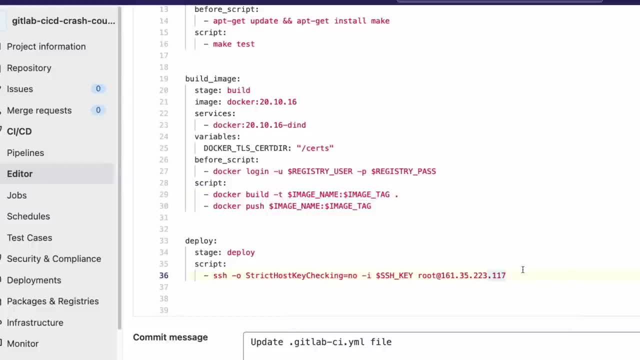 That we just built Right. So we need to execute Docker run or some kind of similar command, And we can do that passing the Docker command to the SSH command. So we're saying: once the SSH, please then execute whatever is defined here. to a line break here and let's write our Docker run command. 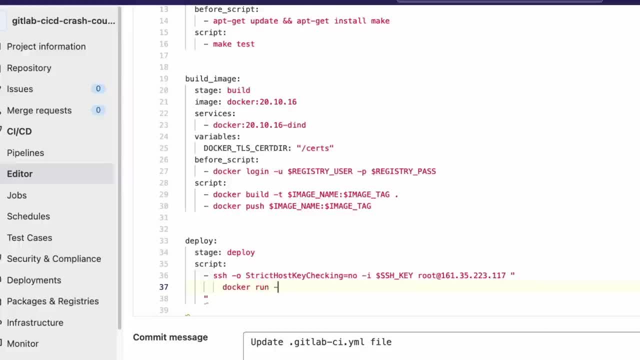 So, first of all, our application is running on port 5000. So we're going to expose that port on the host Like this. then we have the image And since we have parameterized this, we can just copy those values. 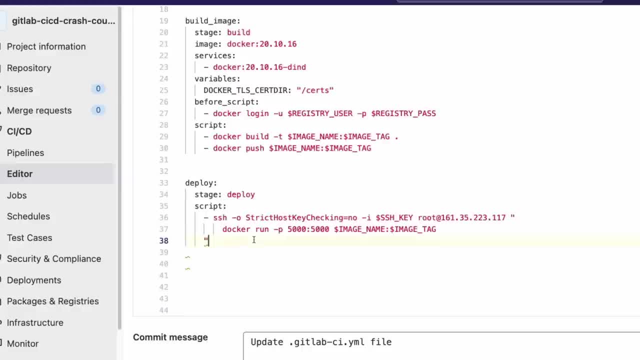 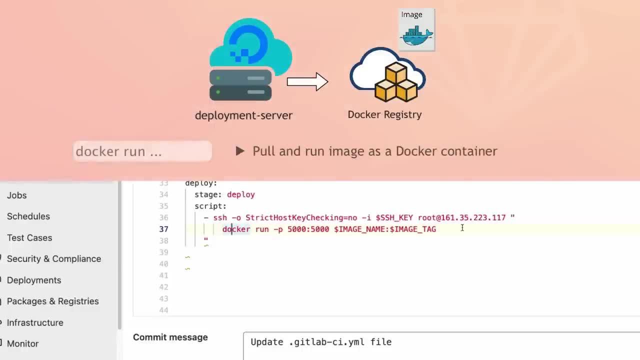 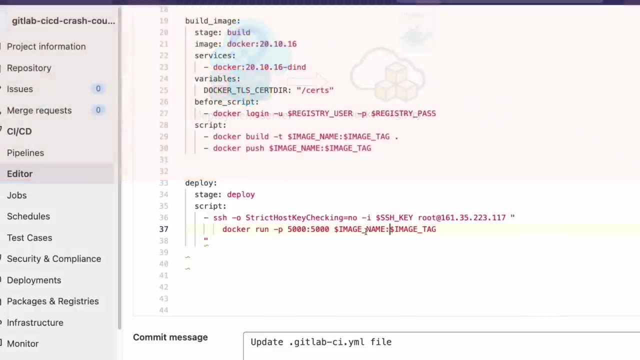 So that's the image. Now there are three more things that we need to configure in order to make this deploy job successful. First of all, this command will be executed on a droplet server, and it will actually pull the image that we specify here from the private registry. 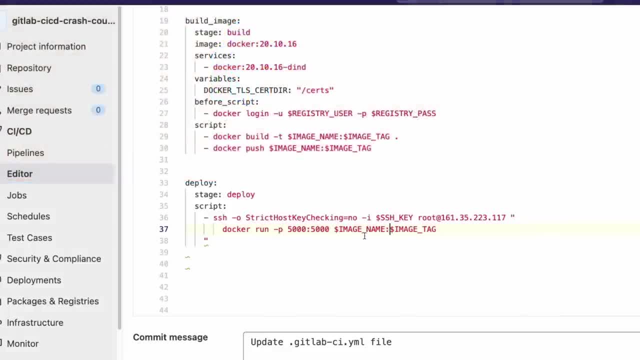 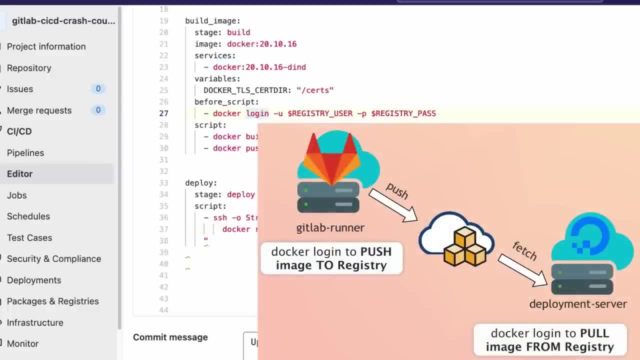 And that means we need to authenticate with that registry to be able to pull the image. So just like we had to do Docker log in here in order to push an image, we need to do Docker log in here in order to pull the image. 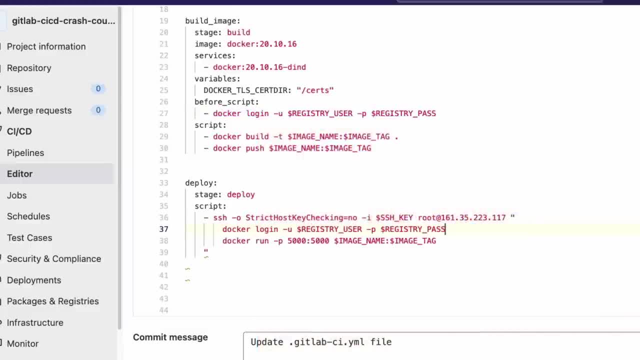 So we're going to copy this thing and edit here before we run the image, And since these two are going to execute inside the SSH, we need to add this ampersand here. So we're kind of chaining multiple SSH commands together. So that's one thing which will take care of. 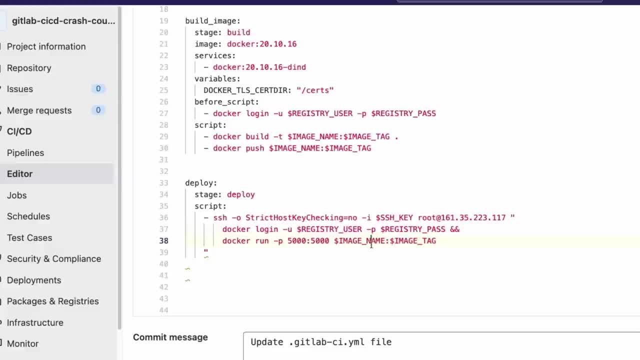 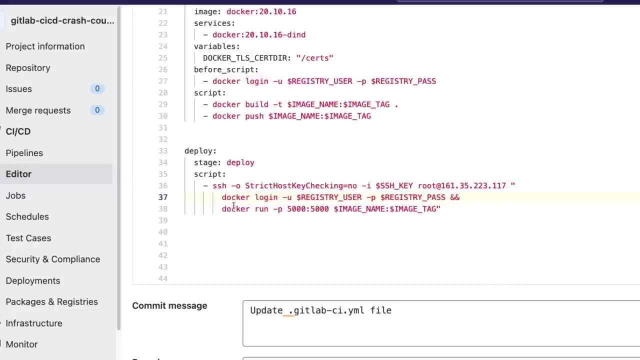 So authenticating with the registry and pulling the image from the repository. So this is the first one. The second one is that when we execute this pipeline the first time, it will actually succeed. right, It will create and start the Docker container on the server and that's it. 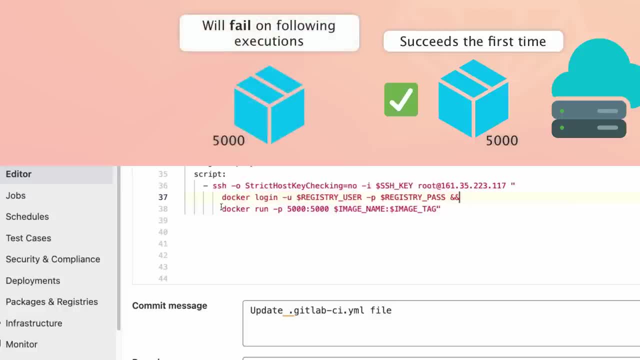 But on the second execution or any following execution, it will try to create and start a new container on the same host port, And obviously this is going to fail because you can't run multiple processes on the same port, right? So before each Docker run command, we also need to make sure to stop and 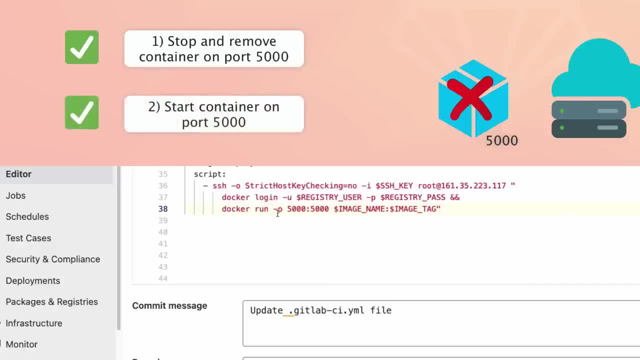 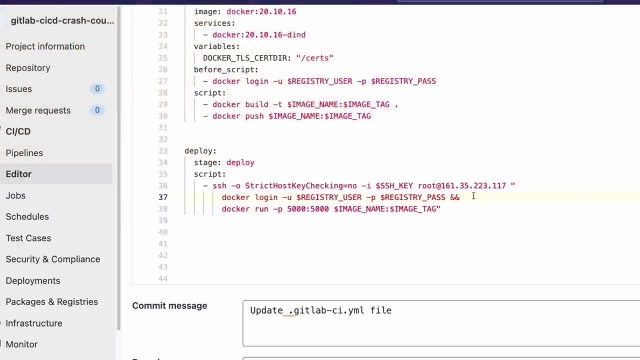 remove any existing containers or at least stop any currently running containers on port 5000 so that a new one can be created. So that's the second thing we need to do, And because we know that this server will only host and run our application. 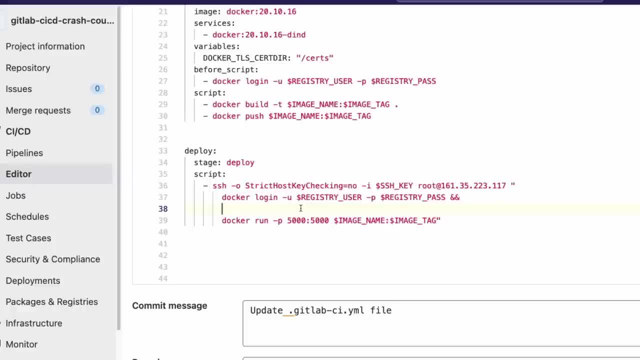 we know that there is going to be one container and we just want to stop that, And we're going to do that using the following command. We're going to do docker ps, dash a, So this will list all the containers. whether they're running or stopped doesn't matter. 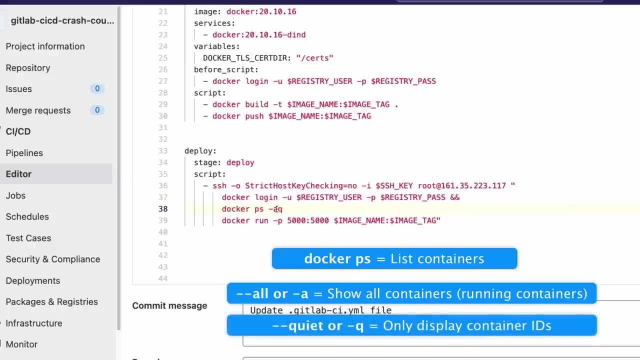 And it's going to list them by ID. So with dash aq version we're going to have a list of all containers Again. in our case it's just going to be one, And then we're going to pipe that command and we're going to stop. 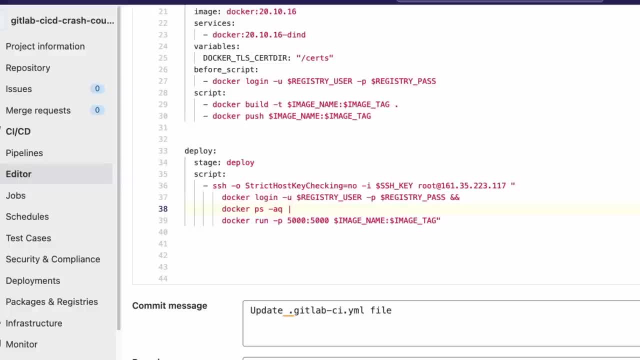 that container using Docker stop command. So we're going to take whatever this displays as an argument For Docker stop command like this, And we're also going to take that list as an argument for Docker remove command. So this will stop any containers using. 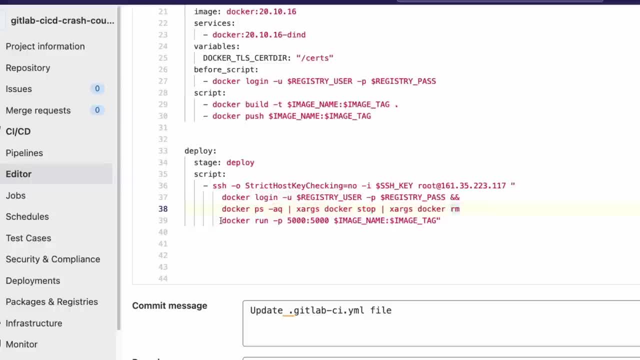 their IDs and it will also remove those containers. And then we're going to create a new one with a new image- And let's not forget the end here- to change the comments. And the third thing we need to do is to create a new one with a new file which is related to the SSH key file. 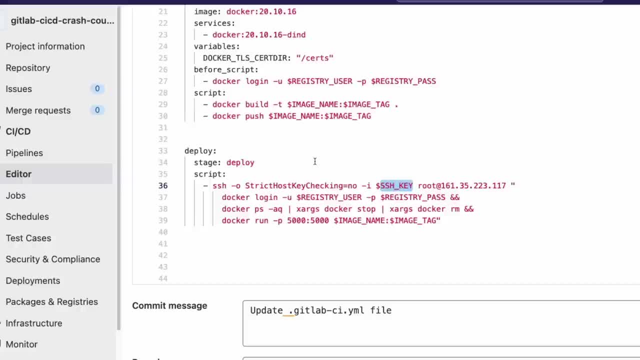 So when GitLab creates a temporary file from this SSH key variable that we created, it will actually set access permissions on that SSH private key file and those access permissions by default are to open so anyone can read and write to that file. And when we try to connect with a private 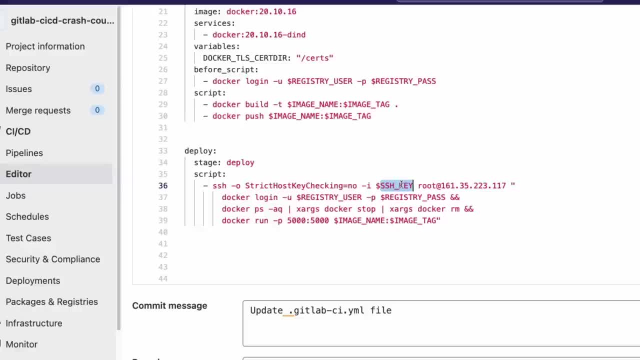 key file which has open access permissions so anyone can read and write to it. it's insecure that the file is not restricted and it has to lose or open access permissions, So we're going to need to fix that and to shortly explain to you what that means. 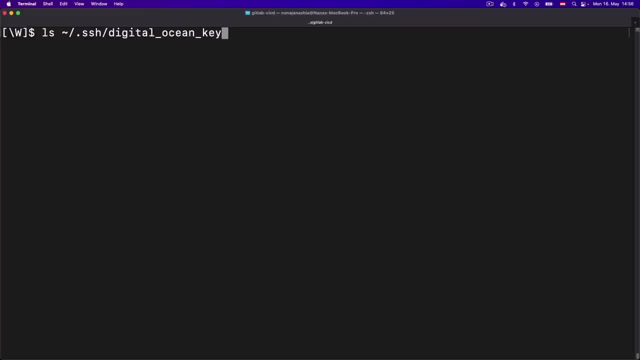 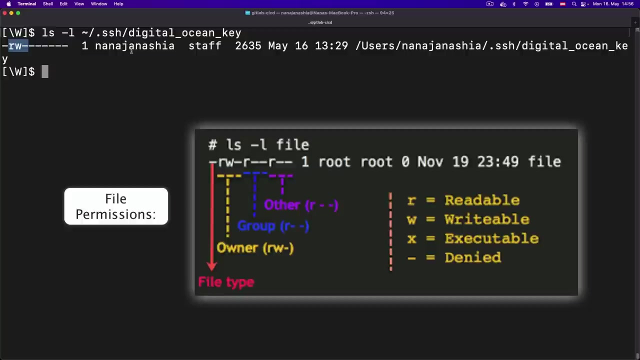 So if I go to SSH and our DigitalOcean key, if I do LS with option L- a long input- this will actually show me who has access to this file, Right? So these are permissions for the owner, which is my user, the group and anyone else. 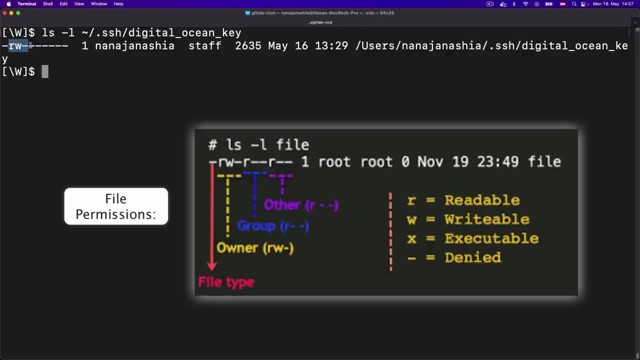 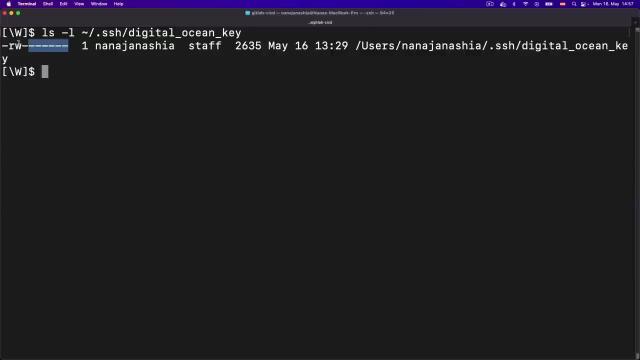 So for this file the owner has read and write permissions, but no one else can actually read or write or access this file in any way. So that's a restricted access, And that's what we need to do here on GitLab as well. 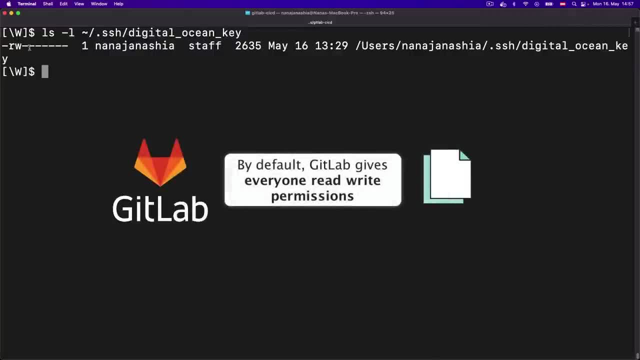 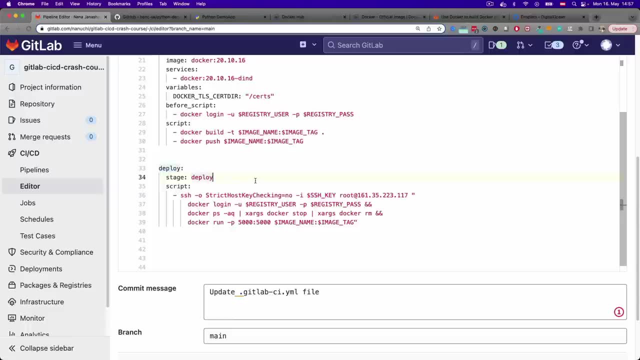 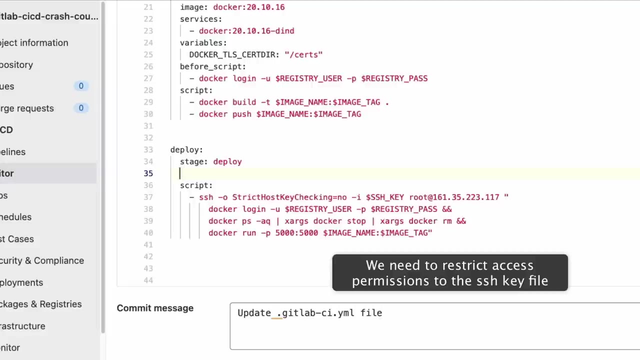 And, as I said, by default GitLab actually gives everyone a read write permission when it creates a temporary file from the file type of variable, And we can fix that very easily by setting the permission to a stricter access before the script will run inside a before script section. 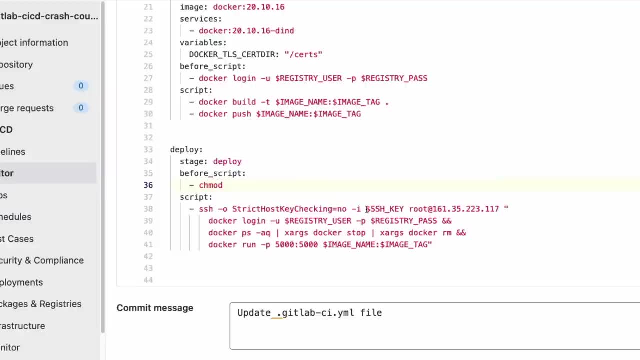 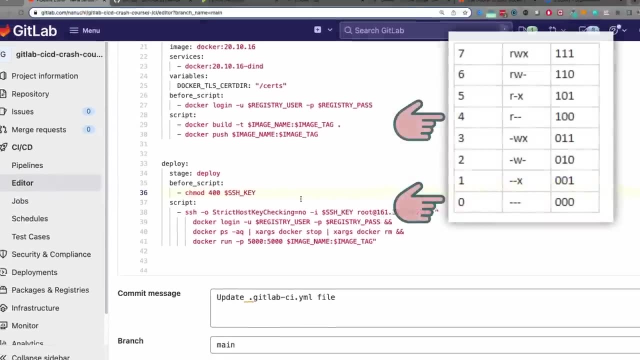 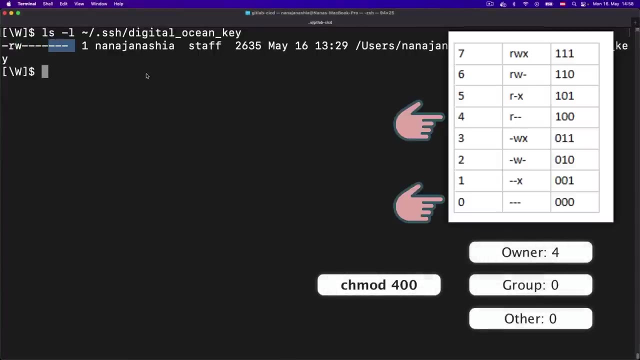 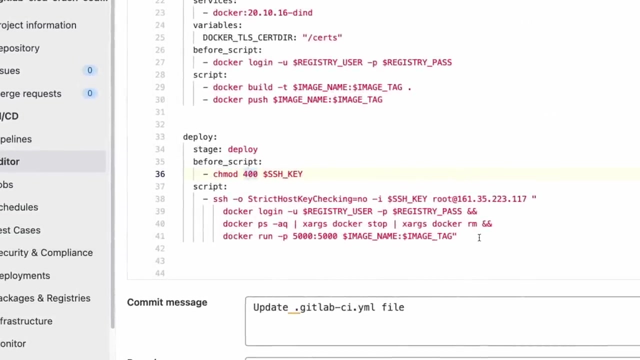 So right here we're going to do change mode of the file, the temporary file, to access 400. So 400 will actually be read, so without write, and then 00, so no access 400. So that's the third thing we need to do for this job to run successfully. 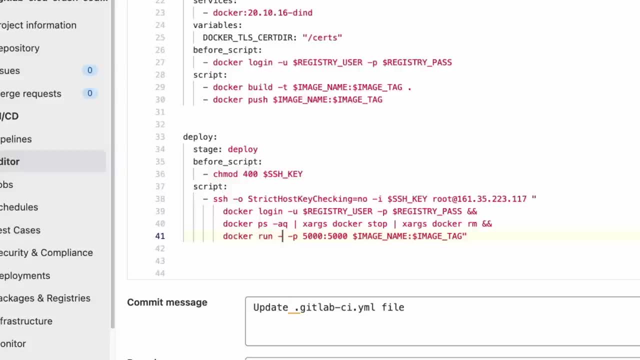 And we also need to run the Docker run command in a background or in a detached mode with minus D, because otherwise it will block our terminal or the jobs terminal and it will basically just endlessly wait. And with minus D or detached mode it will just send the command in the background. 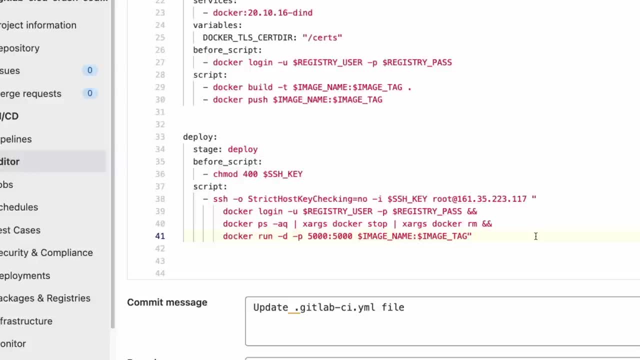 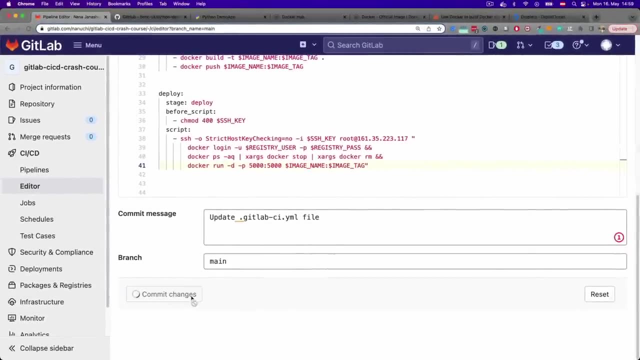 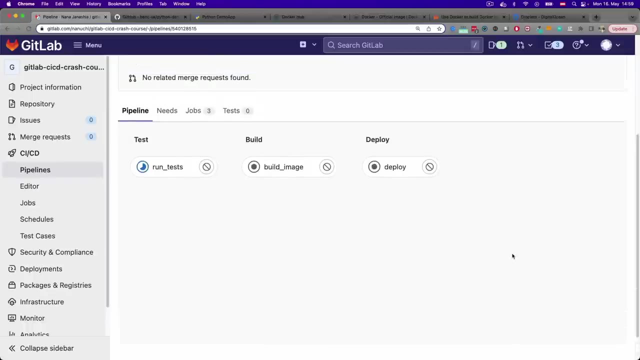 And we'll complete the job. OK, so that's the whole configuration. Now let's actually commit that and trigger a pipeline which will deploy our application to a deployment server. So let's go to the pipelines and let's wait for the execution. 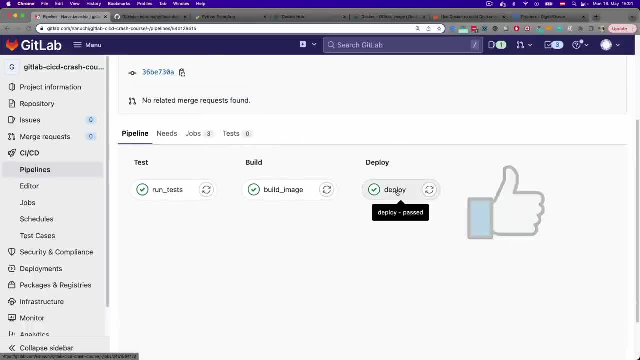 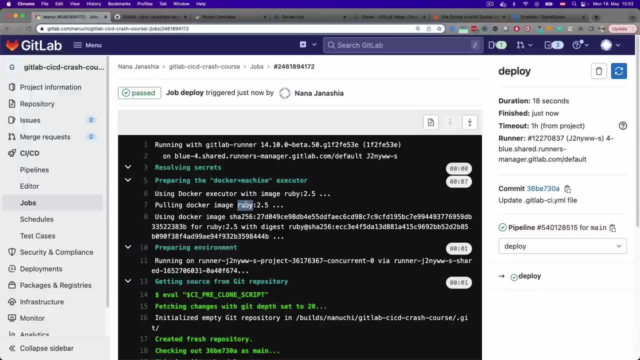 Awesome. So our pipeline went through. We have a successful deploy job. Let's actually check the logs. And first of all, I want to mention that, because we didn't overwrite the image, the default Ruby image was used to create the job container. 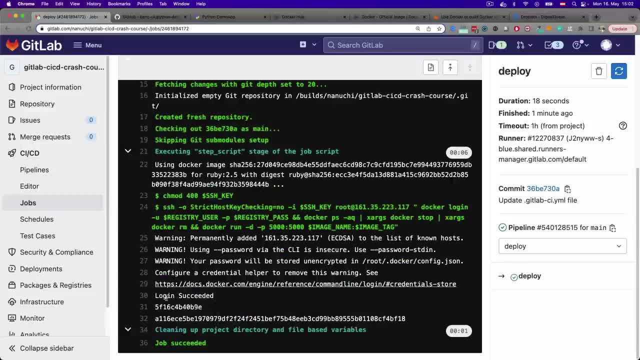 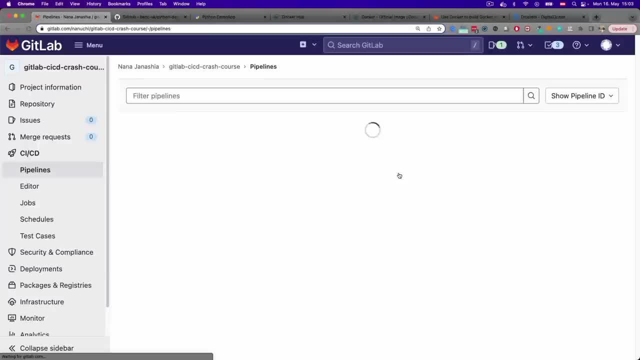 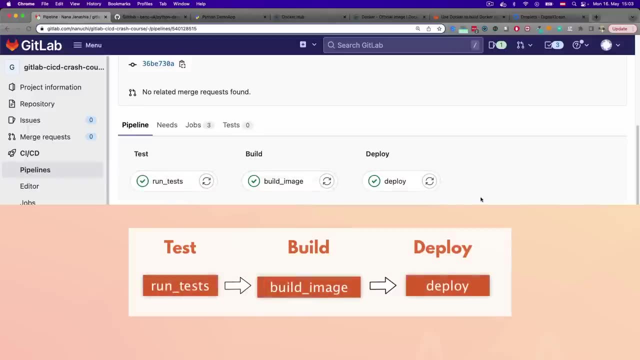 Then we have our change mode before script command, And here is a result of Docker login command. And then the container has also started And we also have three stages now: test, build and deploy stage, with each one having its respective job. So we can now validate that our application is running, first by going to 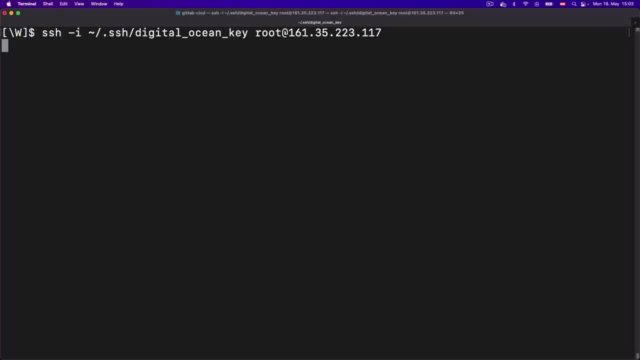 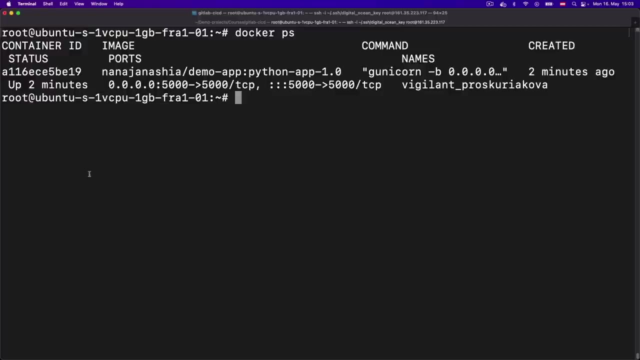 the remote server, that's SSH into it and checking that the Docker container is running. and there you go, we have our Python app. That's the image running on port 5000.. And the second way to validate: of course, we want to access this web application from a browser. 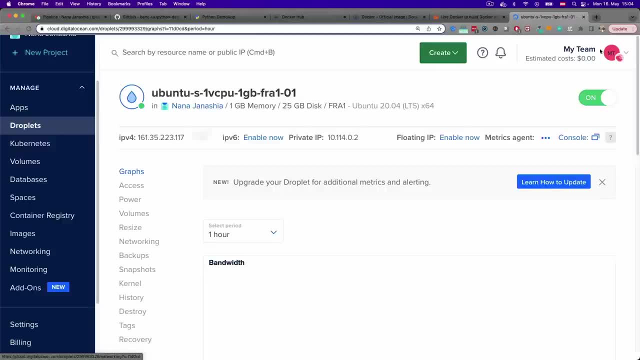 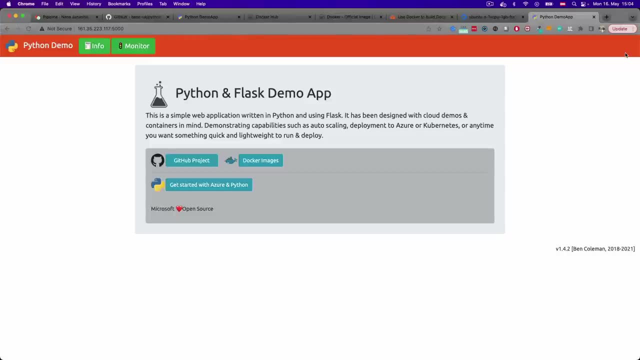 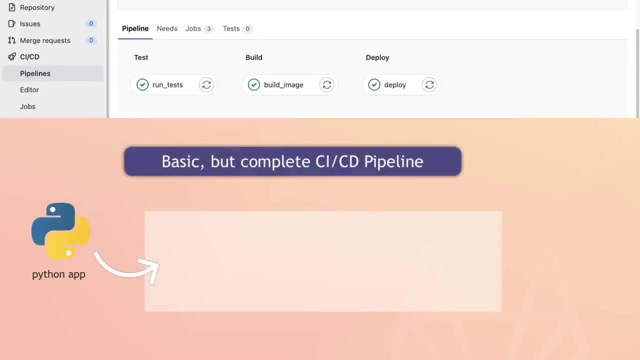 Right. So on the droplets, public IP address on port 5000, because that's where the application is exposed. There you go. We have our application accessible from the browser. So with this we have actually successfully built a basic city pipeline for our Python application. 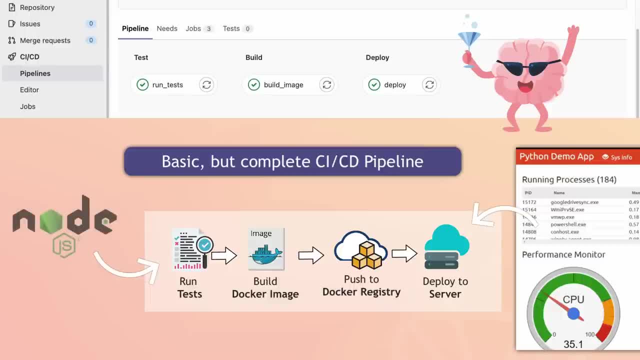 And, as I said at the beginning, this actually applies to any application written in any programming language. These two jobs are anyways very generic, And for this one you would just have to find a respective image, And that's basically it. Also, when you're done with the demo, 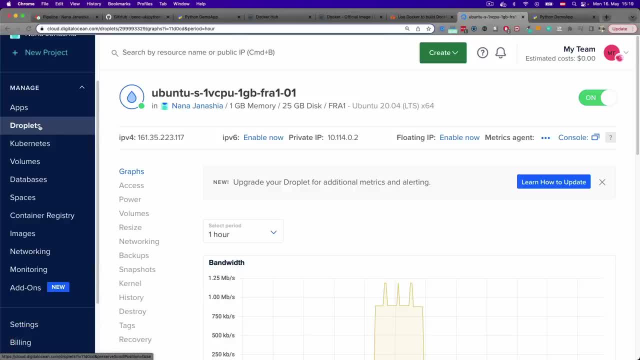 make sure to go to your DigitalOcean account and delete your droplets so you don't get charged for the server resources. So just wanted to remind you of that. And with that our demo project is complete And we have learned a few core concepts of GitLab, CICD.